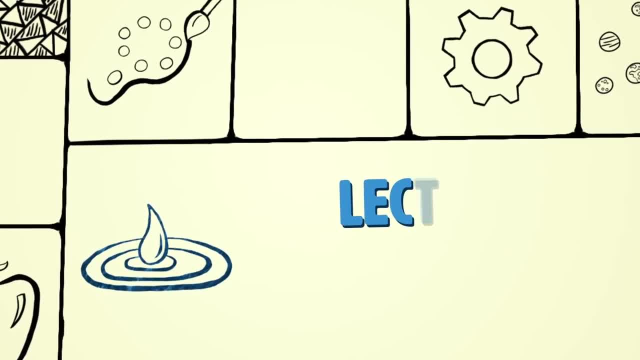 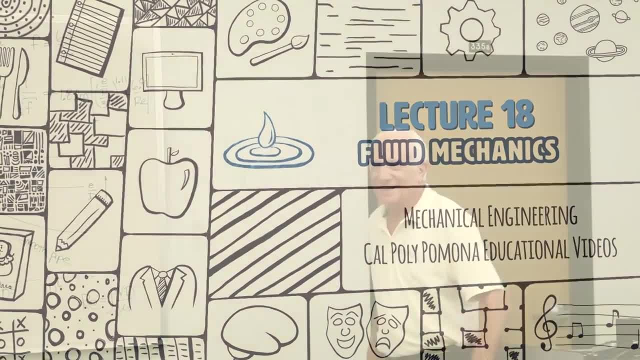 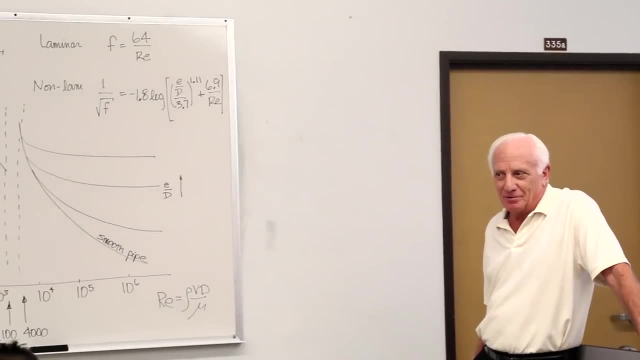 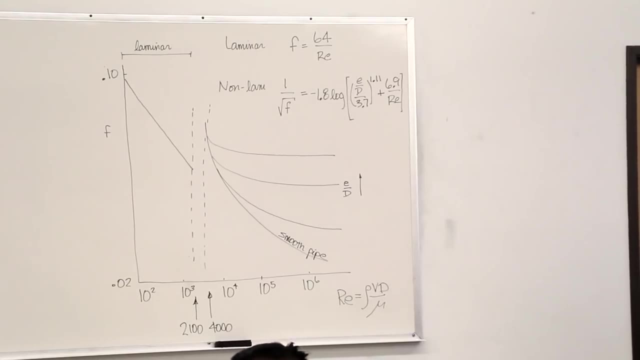 On the right side of the board is what's in your notes, but we're going to use that today, so I put it back on the board for us. You've got a hard copy of the Moody Diagram in your hands from last lecture and you've got a Moody chart in your textbook or e-version. 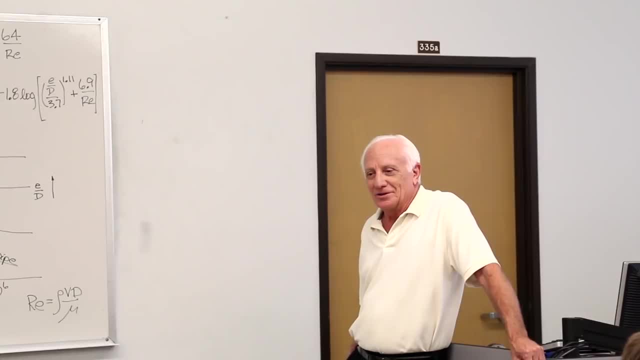 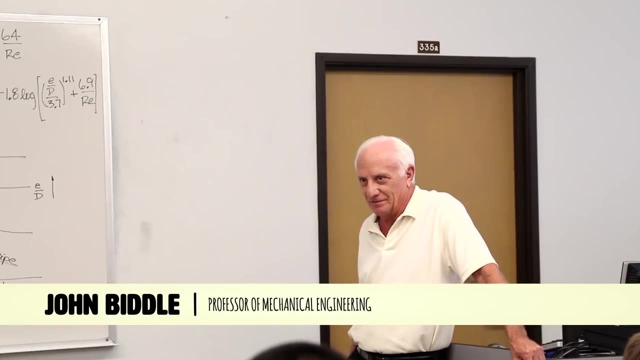 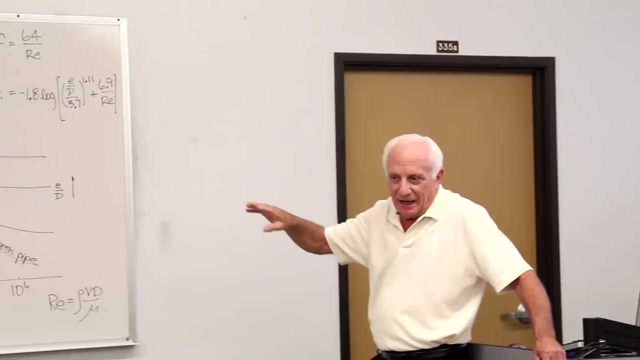 of that And it's on also your tables for the final. So you'll have the Moody chart on the table for the final. Okay, there's two ways you can talk about them, both Graphically. we have the Moody chart. If you're in the laminar range, I wouldn't even bother to use 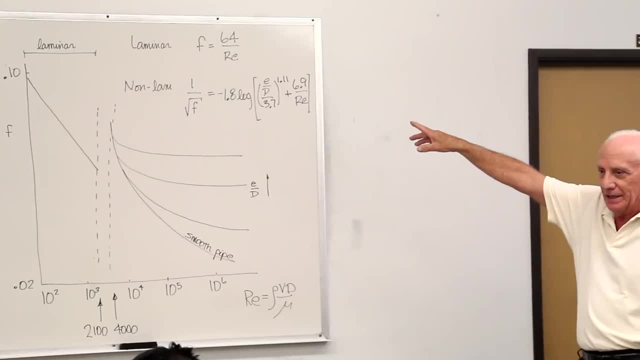 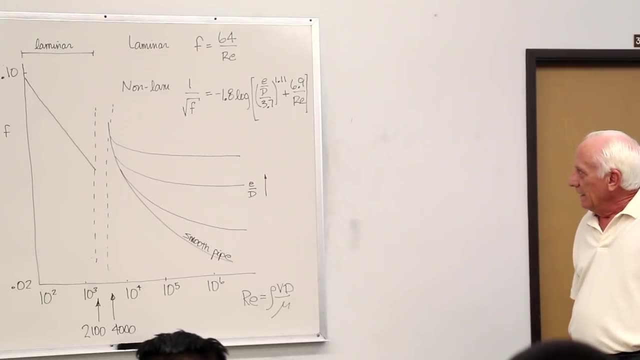 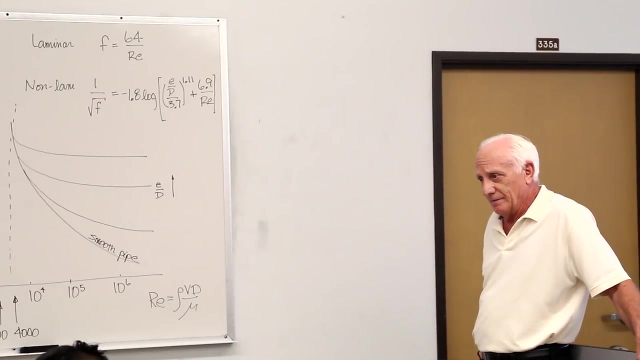 the Moody chart because it's very simple to calculate. F is 64 divided by the Reynolds number in the laminar range, less than 2100.. If you're in the turbulent range, there's different lines to follow Each of the set of lines. 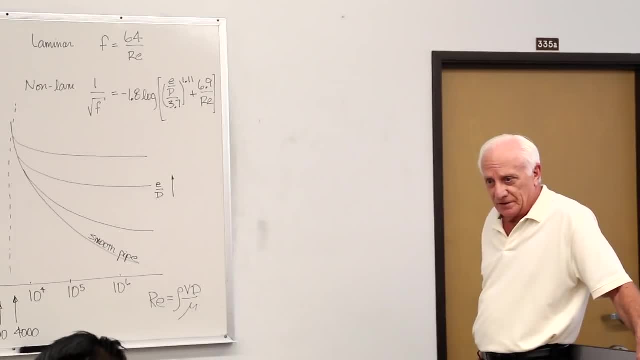 the family of lines offer different relative roughnesses. E is the roughness, D is the diameter. E over D is called a relative roughness because it's dimensionless. The friction factor is dimensionless. The Reynolds number is dimensionless. The Moody chart is a dimensionless graph If it's. 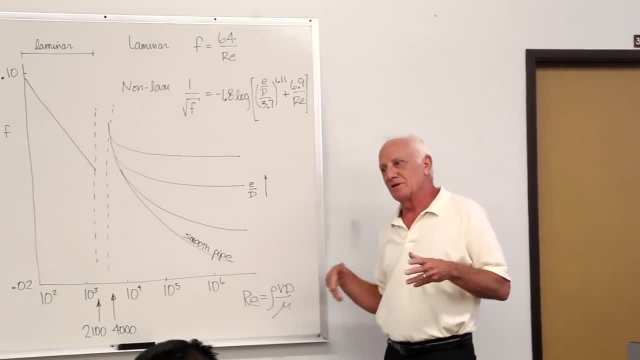 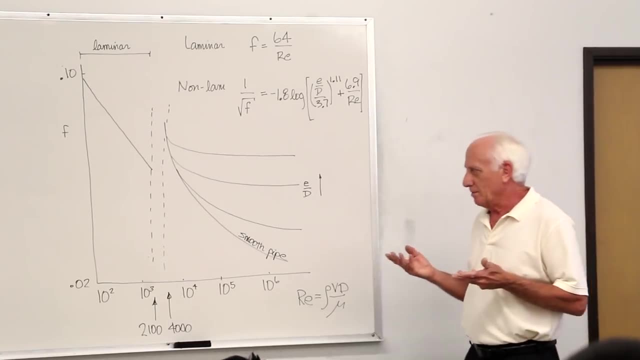 a smooth pipe the roughness is zero. we assume So. for instance, like a PVC sprinkler pipe, very smooth to the touch, slippery, almost to the touch, We can approximate that as a smooth pipe. E is zero for that. And on the Moody chart I gave you there's a little legend. 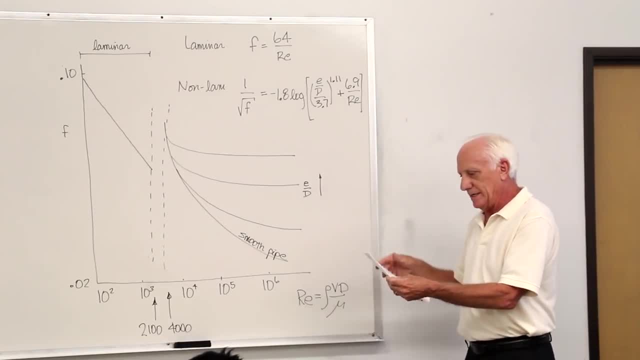 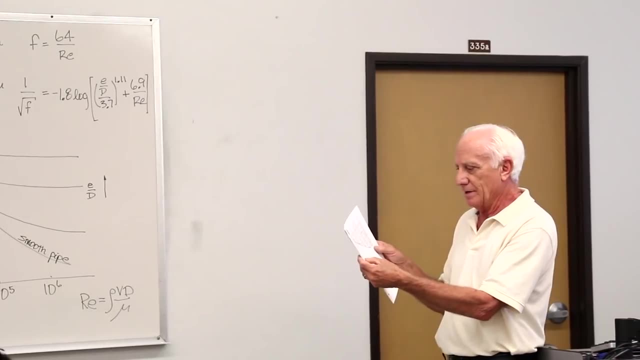 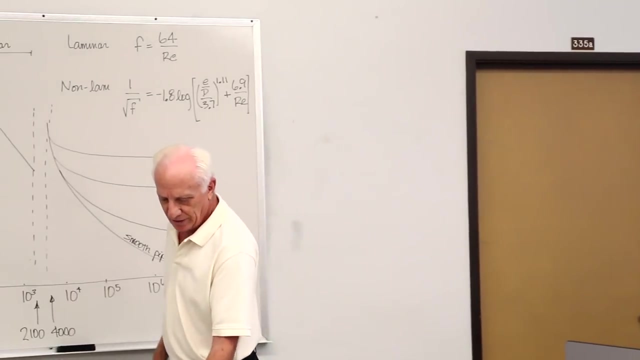 in there which has different roughnesses, values of E in both SI and British gravitation: Ribbon, steel, concrete, wood, cast iron, galvanized iron, raw iron, drawn tubing. So you have a whole selection of different pipe materials that you can get the value of E for. 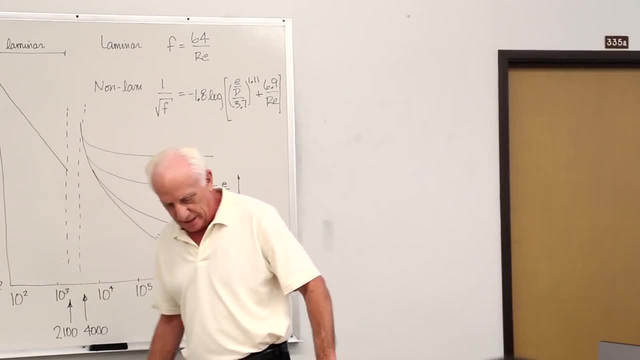 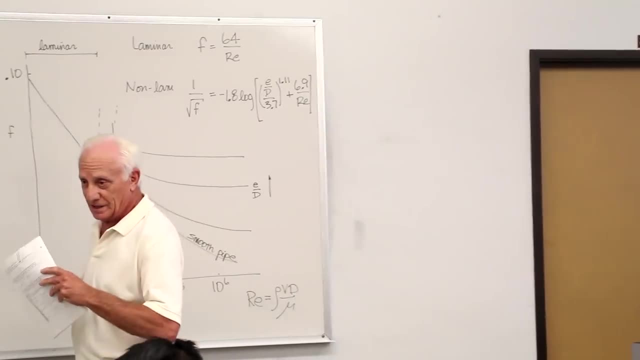 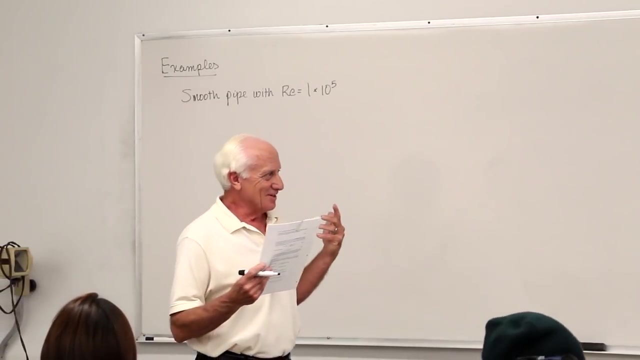 And the way that you use that just to do a quick review is we calculate the Reynolds number First. that's number one. as we said, In a fluid flow situation of a pipe, it's always a good thing to do is calculate the Reynolds number first. That's your first decision. 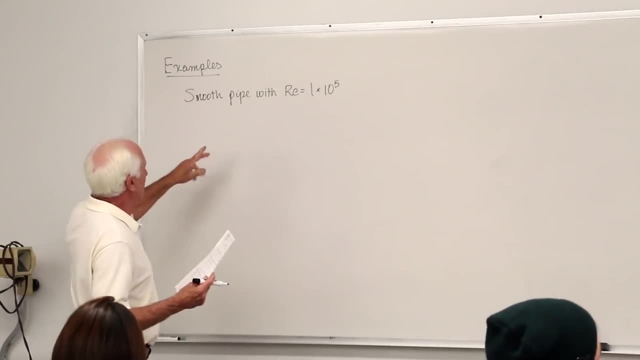 Is it laminar or is it turbulent? Okay, So I'm giving you an example here. I've got a smooth pipe, maybe PVC Reynolds, number 100,000. And I go to the Moody And then I go to the 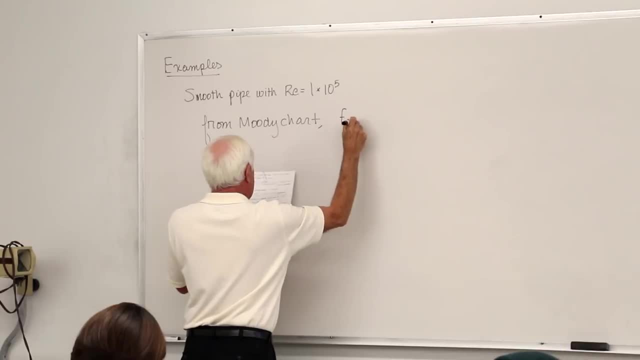 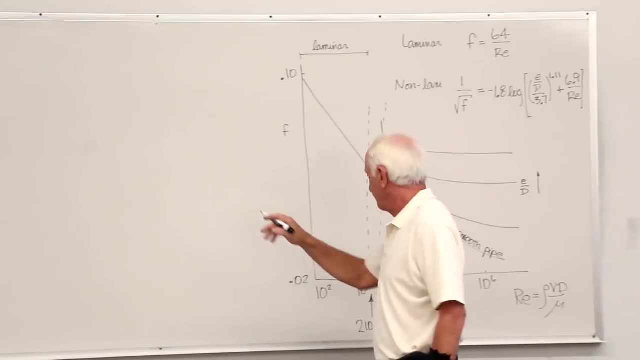 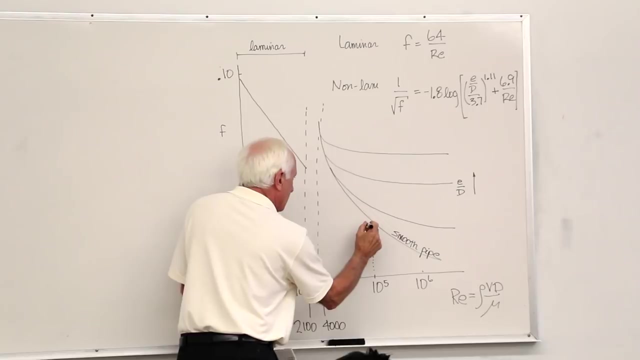 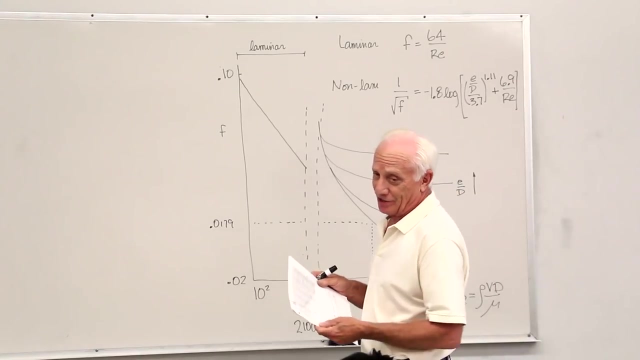 Booty chart. I get F equal 0.0179.. 1 times 10 to the 5th Over here. I go up here Smooth pipe. I go horizontally across 0.0179.. Both axes are logarithmic. They can be somewhat. 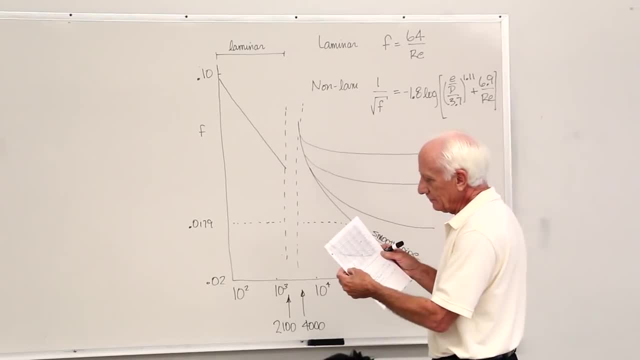 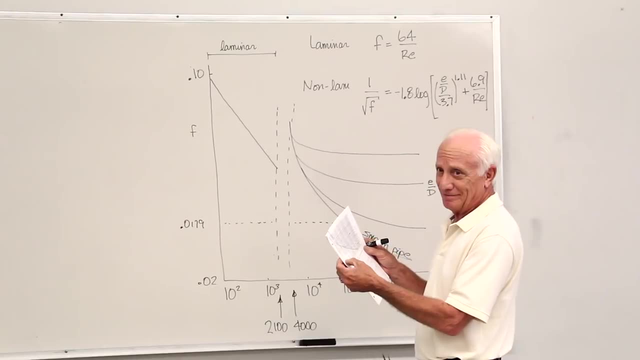 difficult to read. You have to be very careful. Can I read 179?? Well, I think my eyes are really good when I'm reading this. I can see 0.015,, 0.016,, 0.017, and 0.018.. So I just approximated. It's somewhere between: 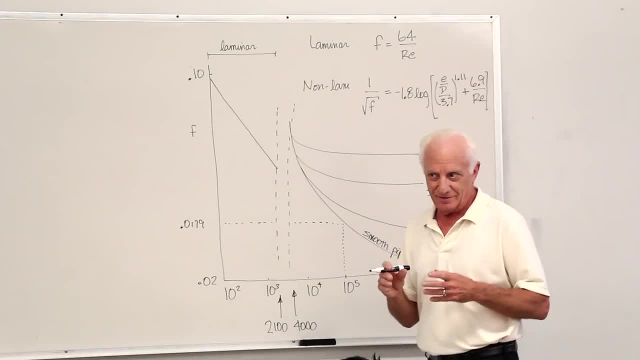 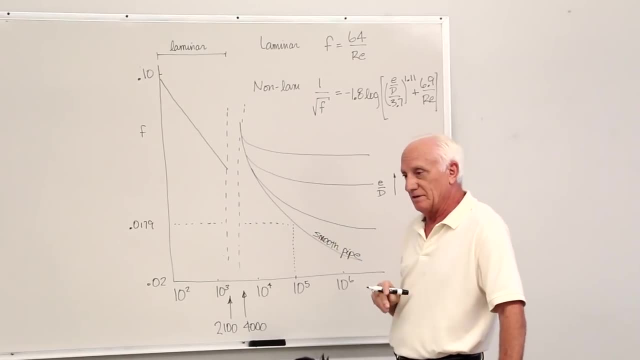 0.0175 and 0.0180.. You can't read super accurately, Probably just two sig figures, maybe three. I could read 0.0175, I think from that graph. 179, I think I'm really close to 180 if I. 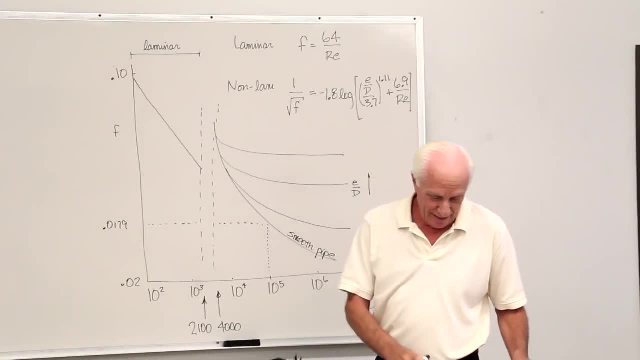 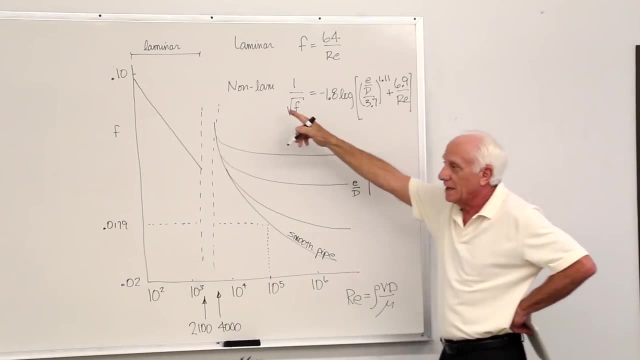 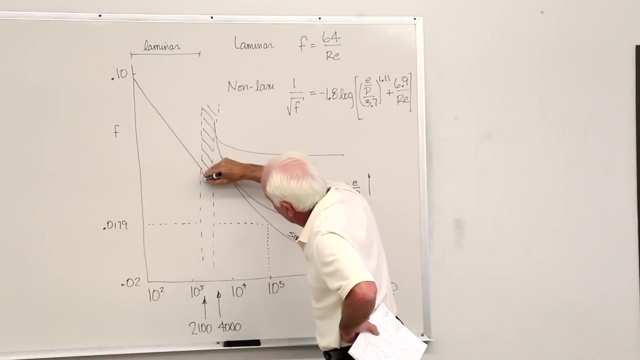 look at it, We'll do that again. OK, Now you also can use this equation, which fits Everything nonlaminar, except the critical zone. Don't forget this zone. right here, We have no equation, We have no graph for that. That's the no fly zone. You don't want to? 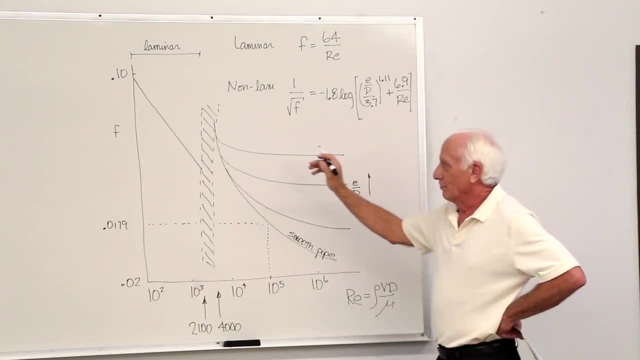 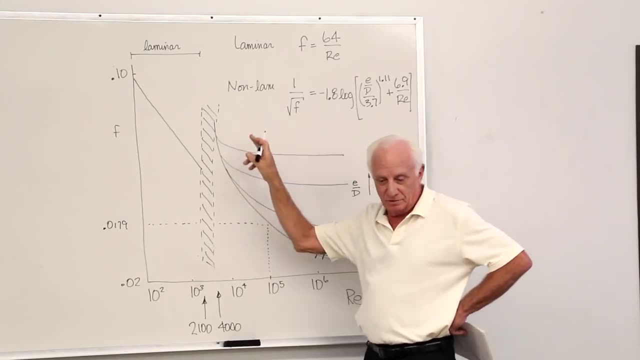 end up there, so stay out of there. OK, To the right of that line at 4,000, that's the nonlaminar it composed of. Well, if you look at this woody chart again, it's composed of two regions. 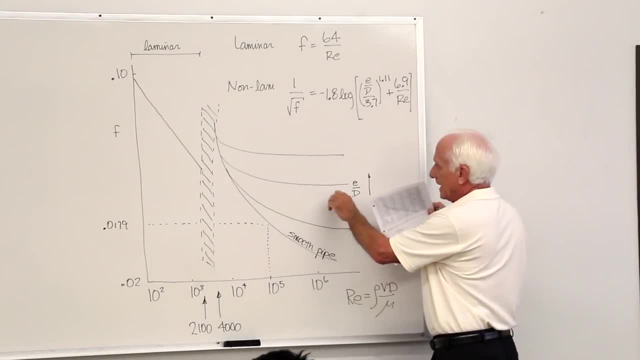 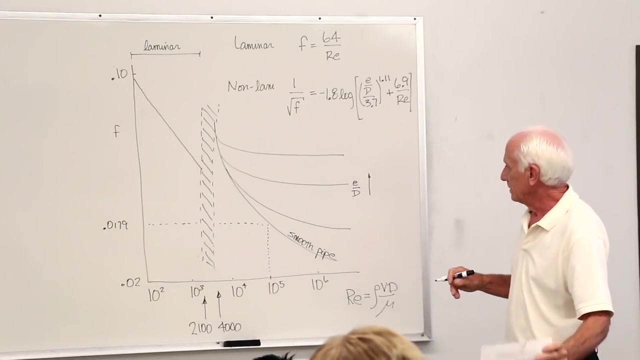 One is called completely turbulent region. That's where these lines are flat, horizontal, Where they curve back up to the left. that's called the transition region. So there's a transition region and a complete turbulent region. The smooth pipe never does end up. 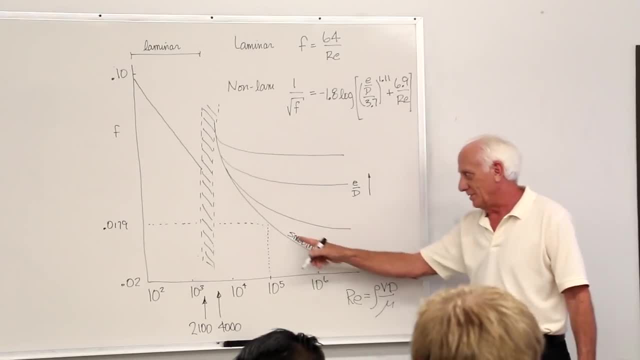 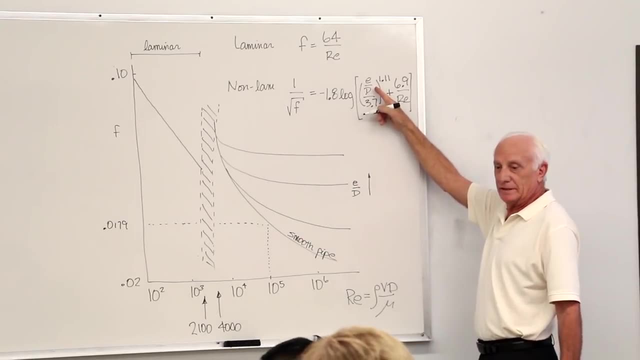 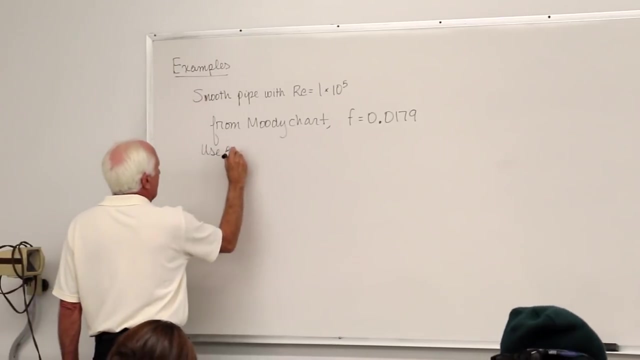 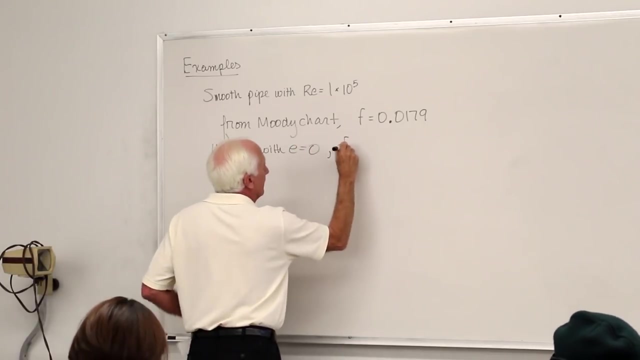 horizontal Never does. It's always coming down this way. Okay, So that's okay. This fits it. For a smooth pipe, put E zero. E is zero Smooth pipe. So use the equation: for smooth pipe, E equals zero. You can back F out of that And I end up with a. 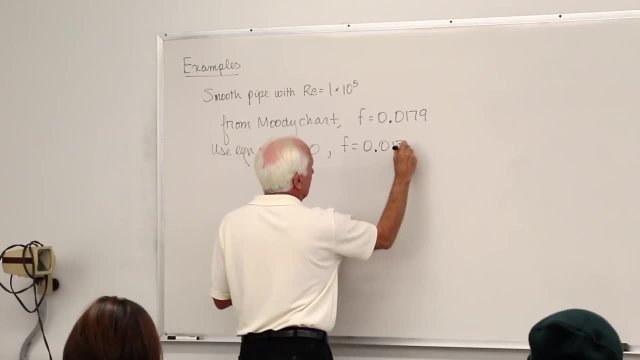 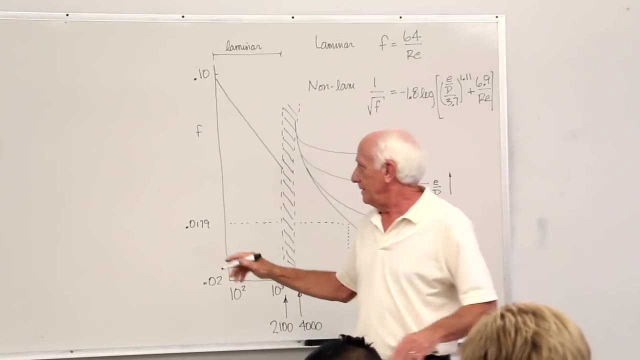 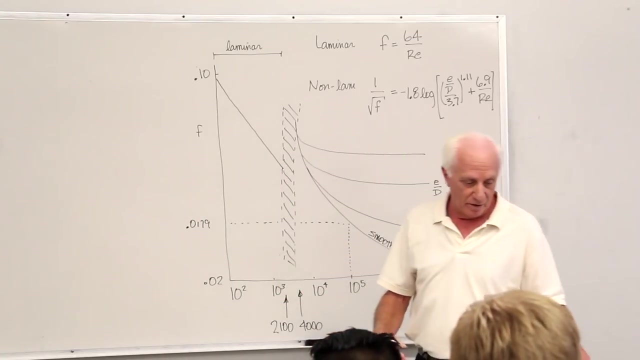 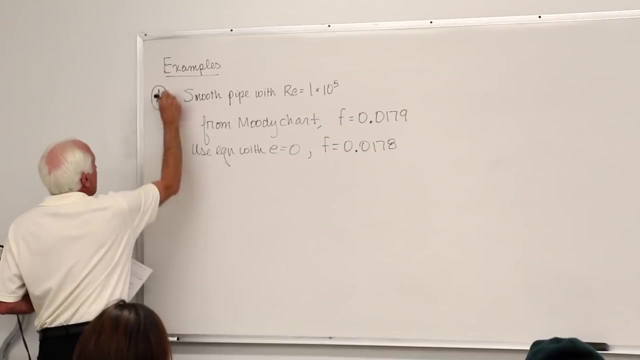 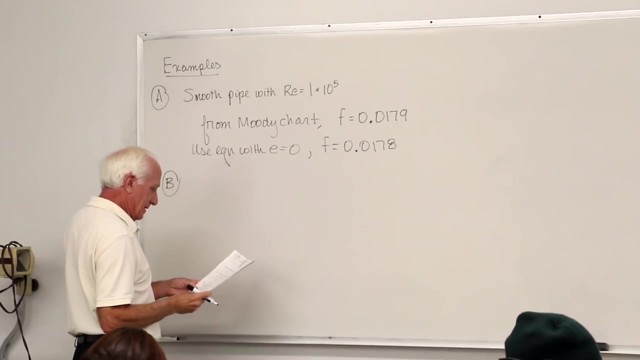 0.0178.. So it's in really good agreement with that. So the smooth pipe curve equation seems to fit really woody chart very well. Okay, Let's take two-inch galvanized iron pipe. Okay, Water, It's water. By the way, this was also. you didn't know it was. 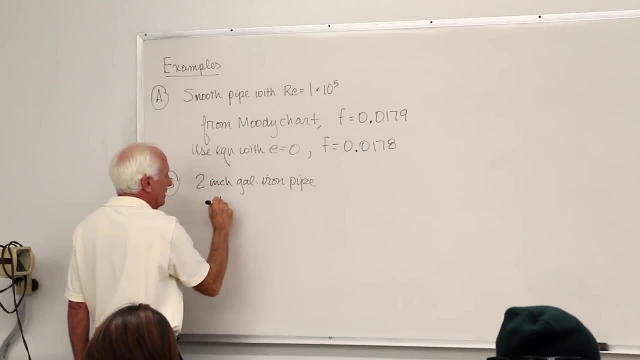 water, That's fine. This is water. You don't need to know that in this one With the velocity average velocity of 10 feet per second. Okay, So this is the smooth pipe. This is the galvanized iron pipe. This is the smooth pipe. This is the galvanized iron pipe. This is the smooth 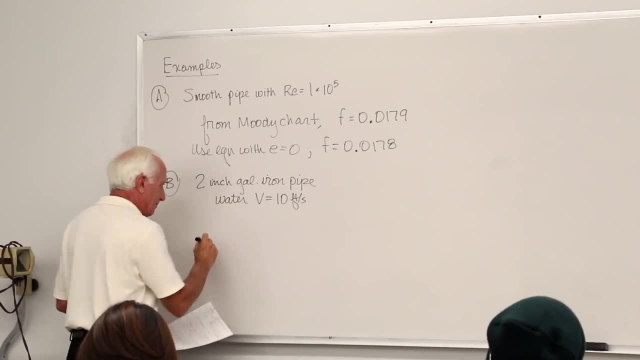 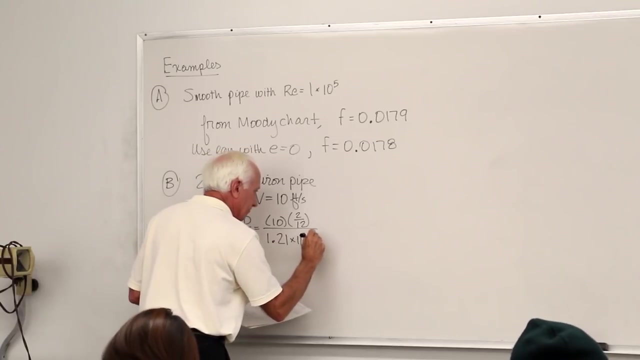 pipe. Okay, Step number one: as we said, get the Reynolds number Velocity, 10. Diameter 2 divided by 12. Kinematic viscosity: in the textbook Reynolds number 1.38 times 10 to the 5th, The value of E over D on the moody chart. in the legend it says, if it's galvanized, 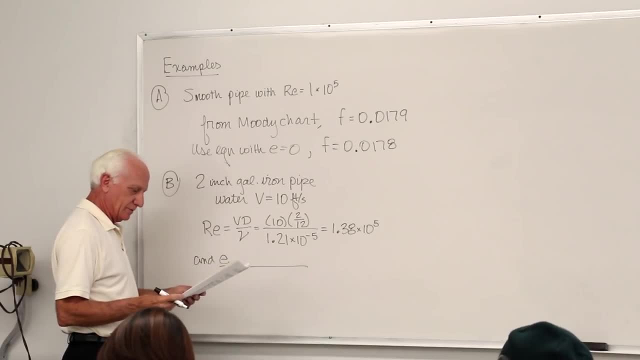 iron in feet E is .0005.. The diameter 2 divided by 12.. 0.178.. Okay, So this is the 0.16667 feet. 0.003. moody chart F equals 0.027.. So I'll go over here. this is E over. D. this is 0.16667 feet. 0.003. moody chart. This is E over D. this is 0.06670 feet. 0.06670 in the legend. this is E over D. Okay, Step number one: as we said, get the Reynolds. number: Velocity: 10.. Diameter 2 divided by 12.. 0.027.. Okay, Step number two. as we said, you can mark in the legend: this is E over D. this is E over D. Okay, Step number three. 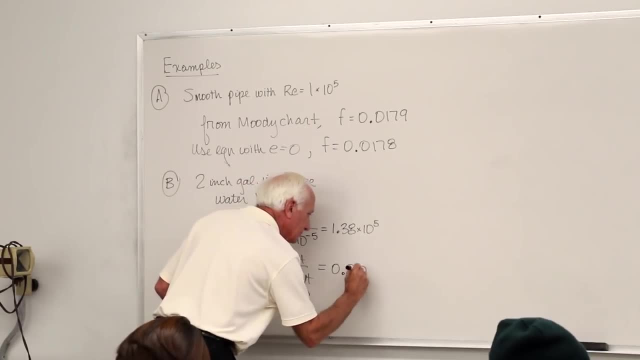 this is E over D. Perfect Step number four. if it's galvanized, this is E over D. okay, Three, four, five, six, seven, six, six seven. Okay, So again the M graph is: 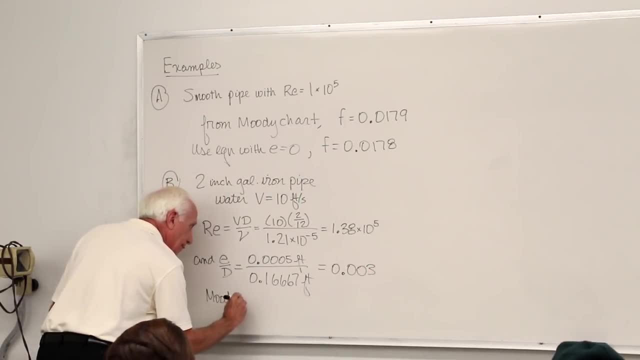 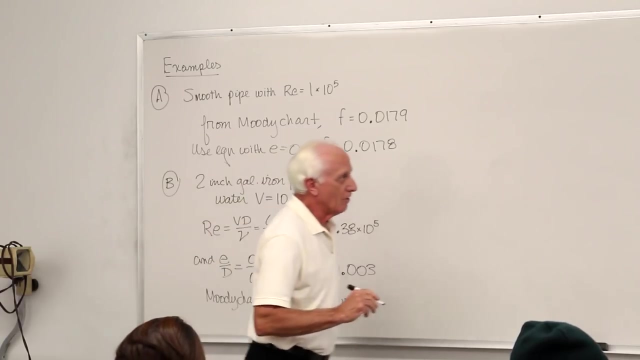 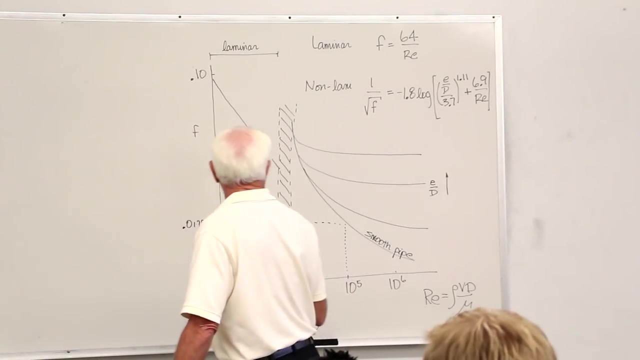 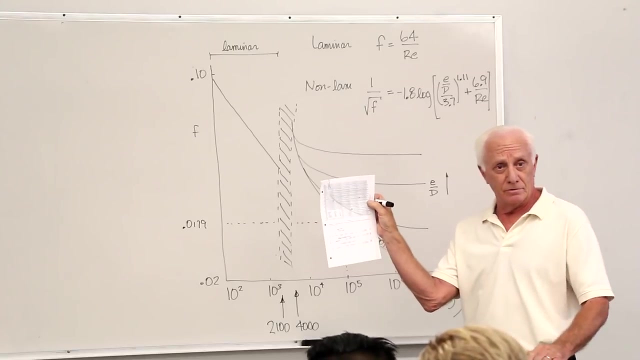 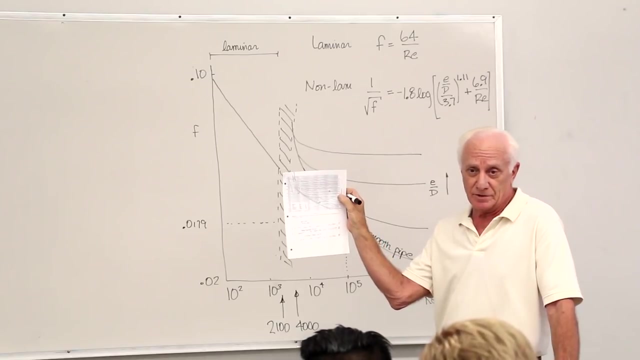 moody chart F equal 0.027. so I go over here. I find the line E over D: 0 0 3, there's a 0 0 2 and there's a 0 0 4 on this graph, which means you have to interpolate okay. 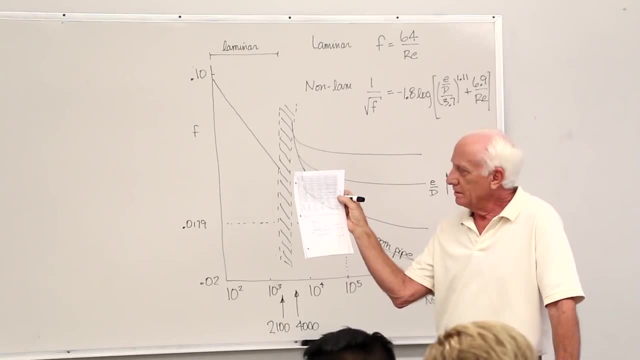 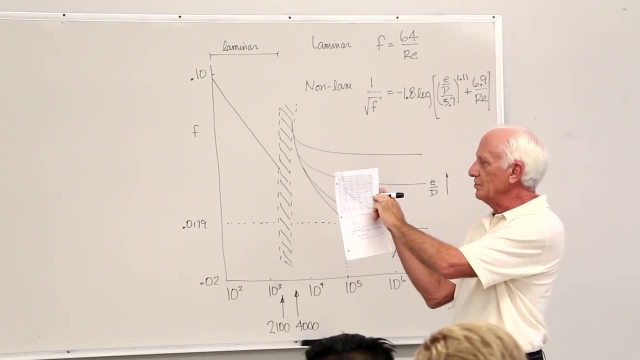 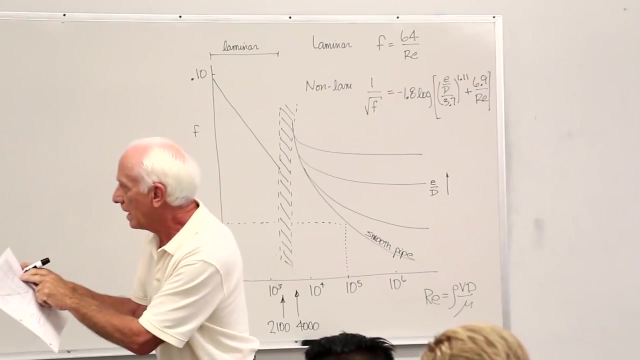 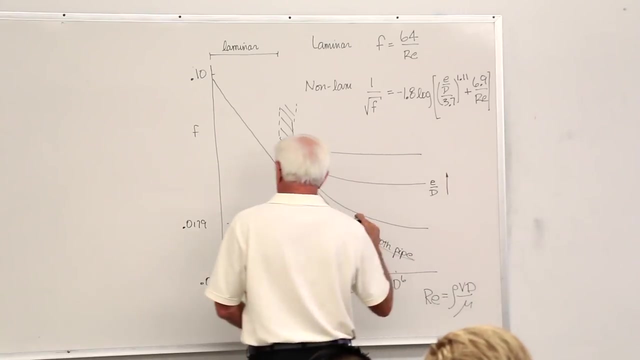 so go half way between is fine, take your pencil. let me draw a line along there between the 002 and the 004. on the E over D, the Reynolds number is one point four times ten to the fifth, so it just started up from being horizontal. so it's right around here. 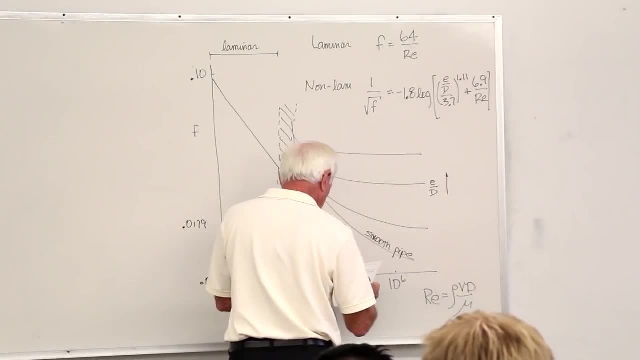 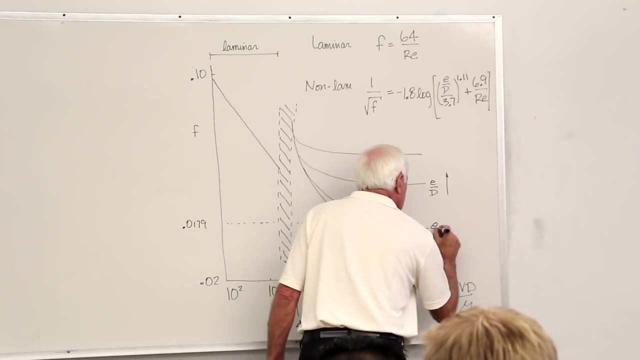 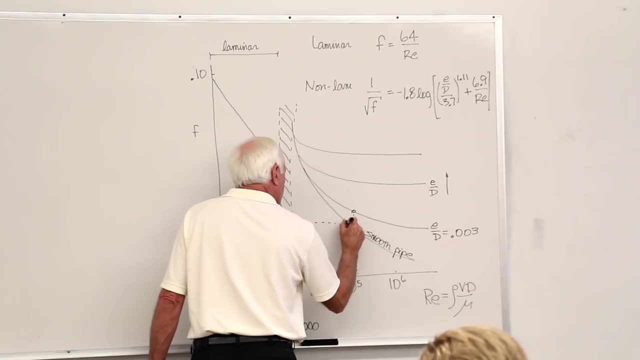 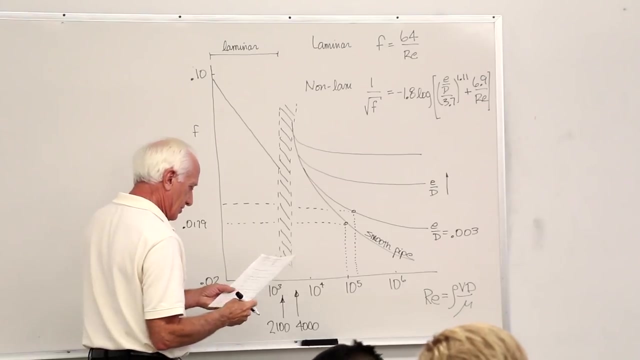 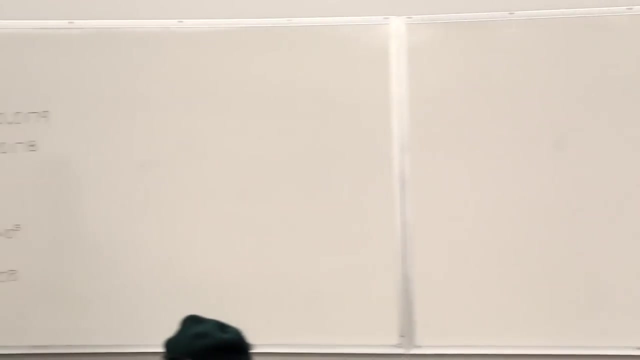 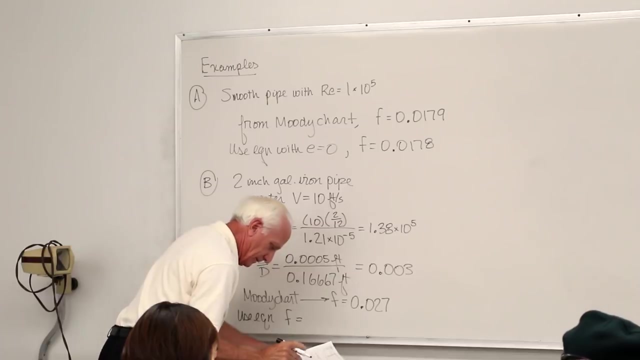 here's E over D, equal 0.003, read across horizontally. and I got, I've got some reading. we chart 0.027, yeah, and if I use the equation, F comes out to be 0.0025. so again, we're pretty close. we're pretty close. 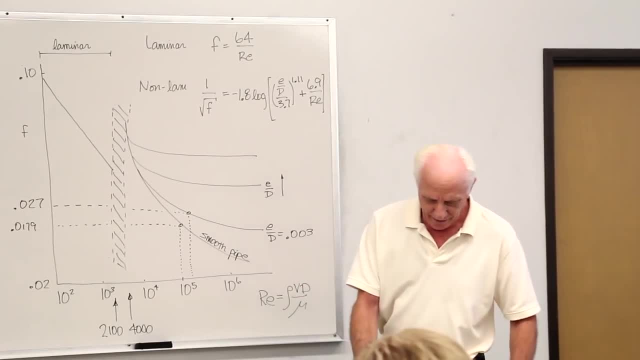 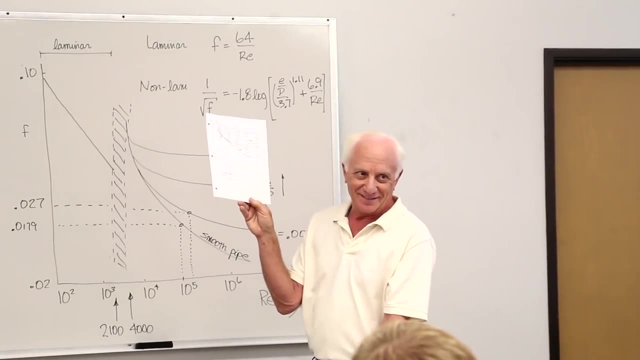 and I've given you three examples on the handout of how to find F. so you've got tons of examples on how to find F for a particular fluid, a particular pipe, a particular geometry. geometry is a diameter, the fluid is kinetic viscosity, the kinematics is the velocity. 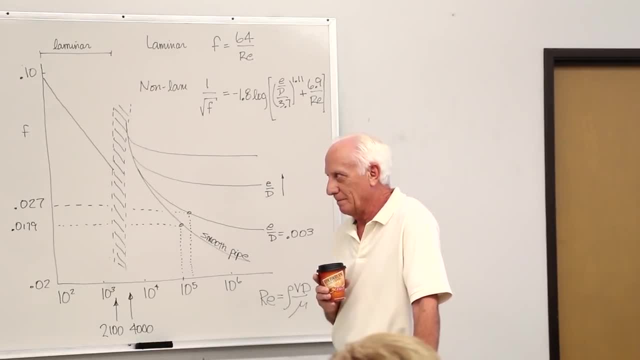 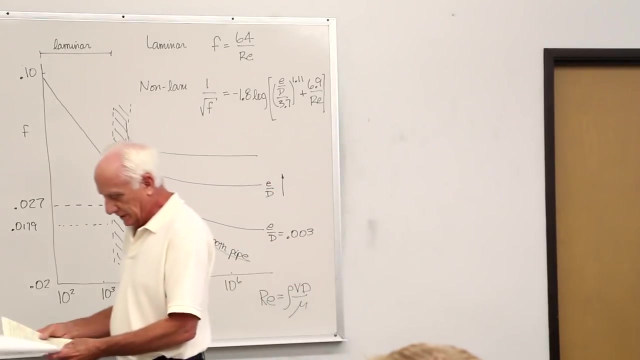 so velocity, diameter and the properties of the fluid. okay, so that's how you, that's how you can use that. now let's take a look at what kind of problems we can have with these pipe flow type problems. this is in the book, but I'll put on the board here also for you. 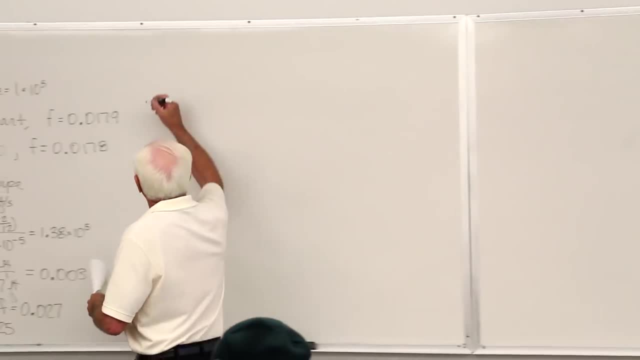 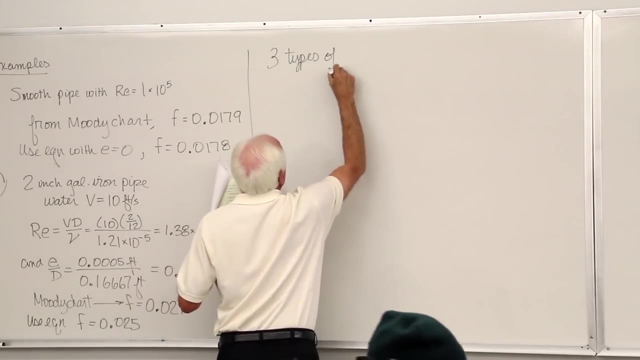 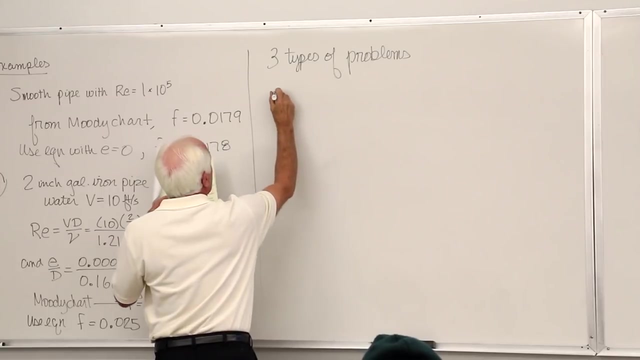 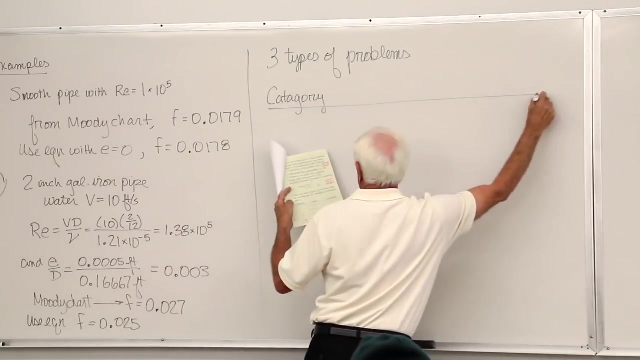 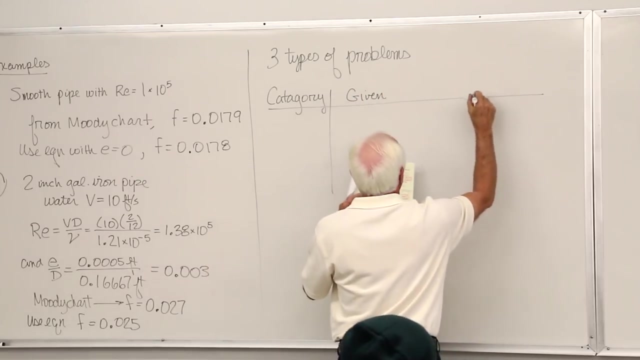 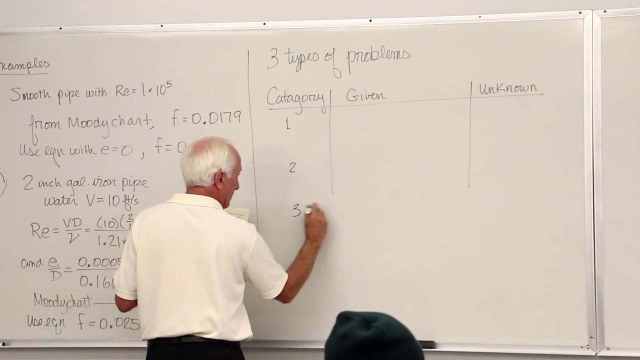 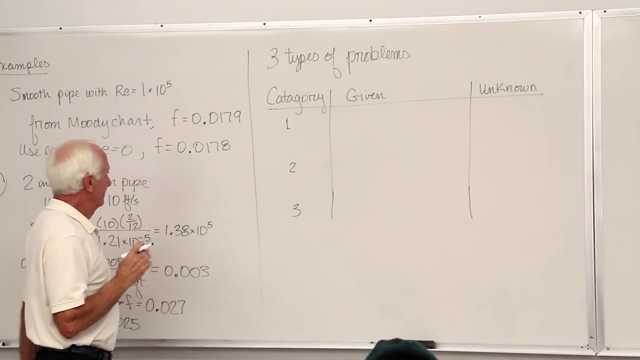 Three types of problems. We'll do category And then we'll do what's given. What's given And what the unknown is. There's a category one type problem, a category two type problem and a category three type problem. Okay, 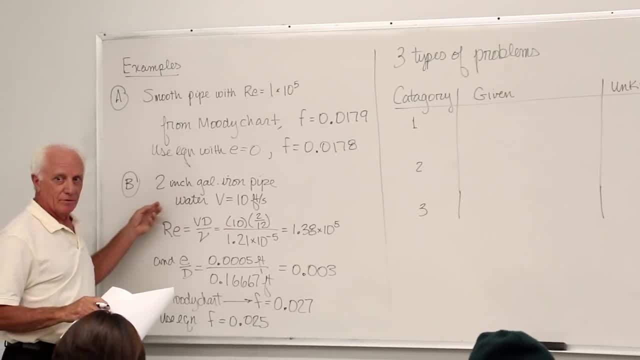 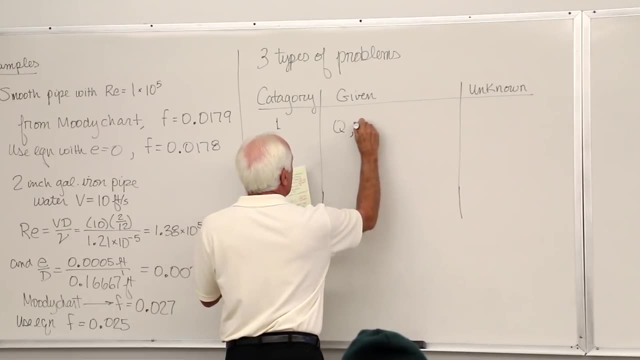 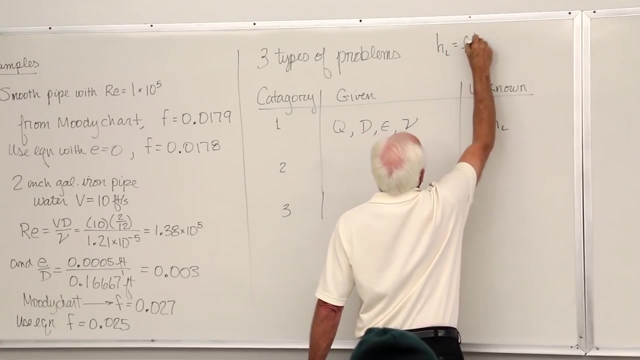 Okay, This is like a category one problem when I worked here. I'm given, for instance, Q, the flow rate, the diameter, the relative roughness and the kinematic viscosity, And I'm asked to find the head loss. 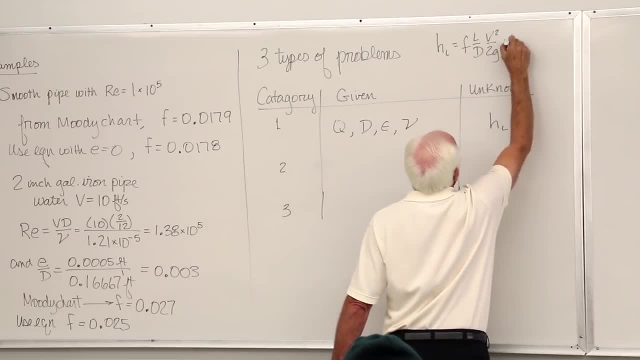 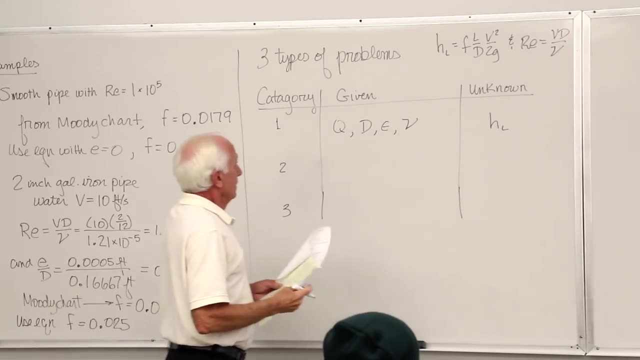 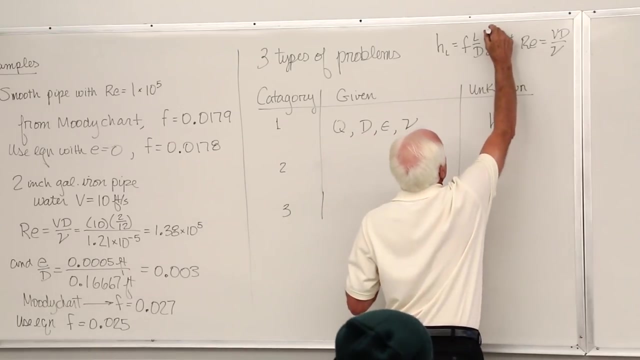 Okay. So what do I do? Well, okay, I take Q and I divide it by the area pi D squared, divided by 4.. That gives me the velocity. So I know the velocity, I know the velocity, I'm given the diameter. 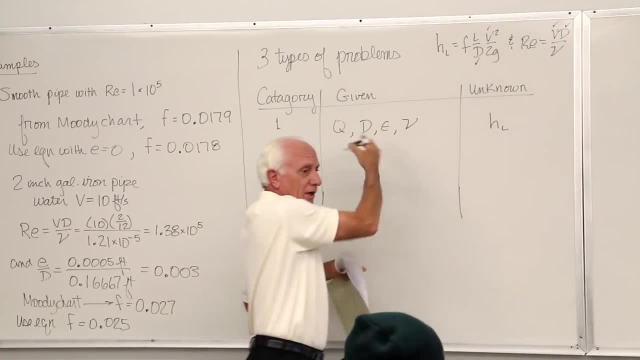 I'm typically given the length too, so I know the length. I know what the fluid is. Let's just say it's water at 120 degrees Fahrenheit. Okay, I know, nu Got it. Do I know the Reynolds number? 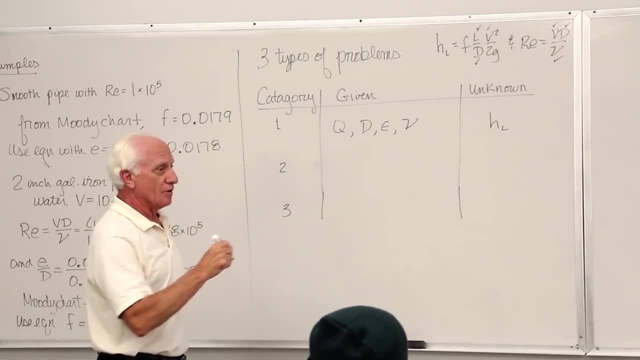 Of course I do. Do I know E over D? Of course I do. What do I do if I know the Reynolds number And E over D? I go to the Moody chart. From the Moody chart, what do I find? The friction factor. 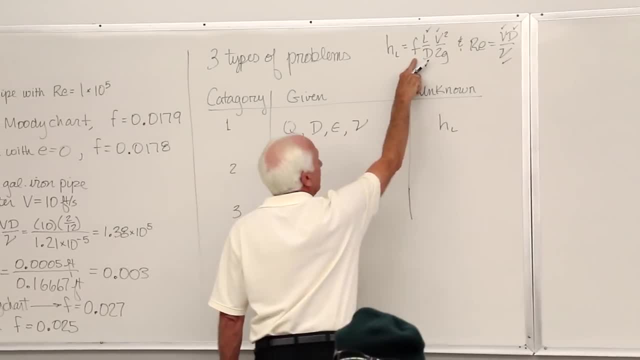 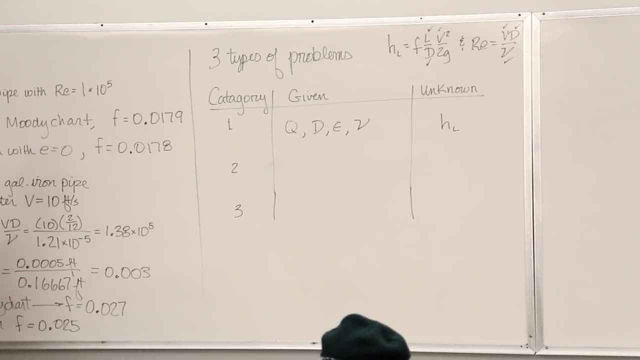 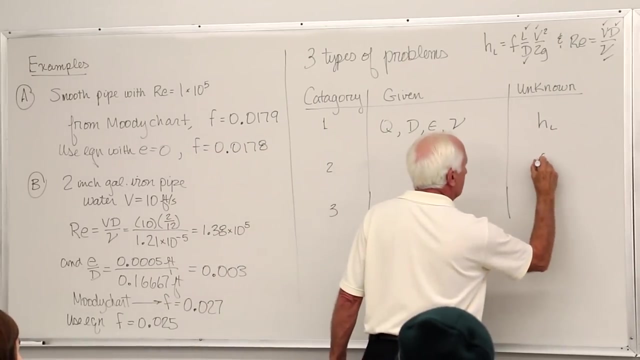 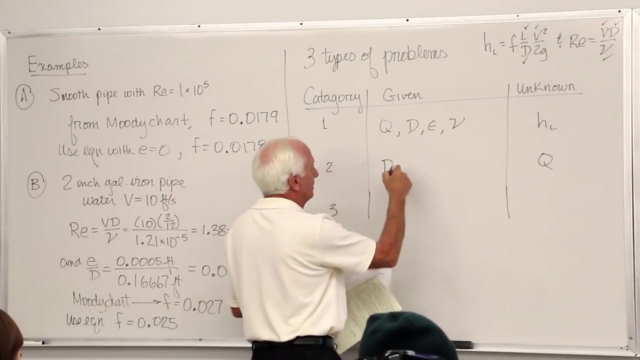 Where do I use the friction factor? I put it up here And what do I calculate? HL, That means the head loss due to friction in the pipe. Okay, Second kind of problem. Now, I don't know Q unknown, But I do know the pipe diameter. 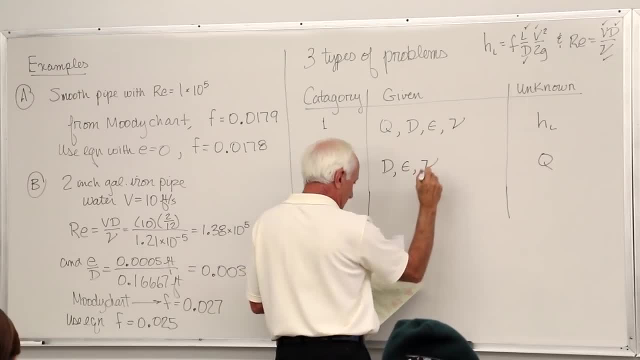 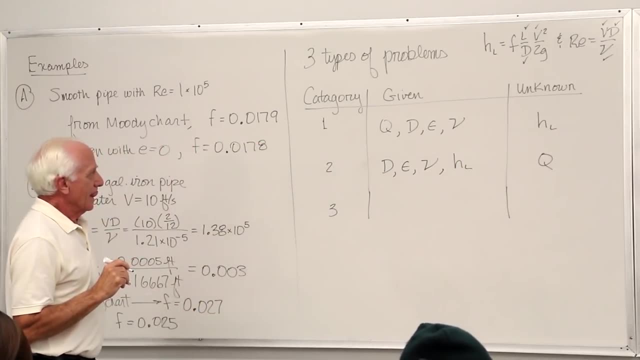 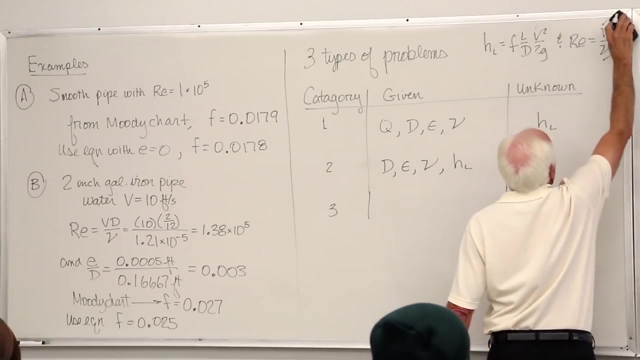 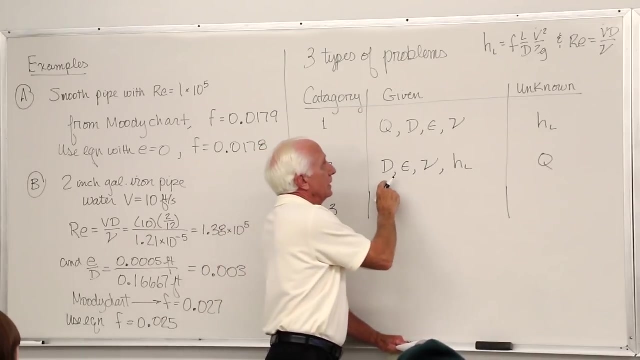 I do know epsilon, I do know nu And I do know H sub L. Okay, So let's put up here again with a check mark. by what we know, I do know diameter, Got it, Got it. I do know epsilon. 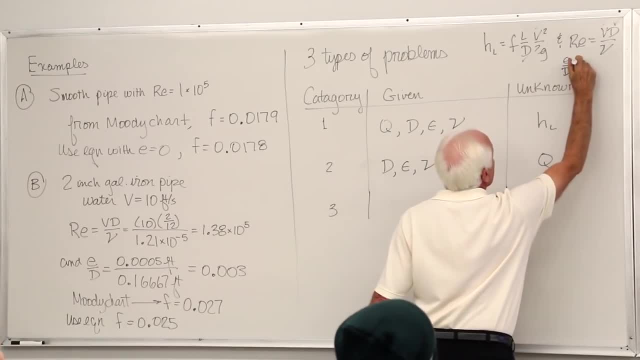 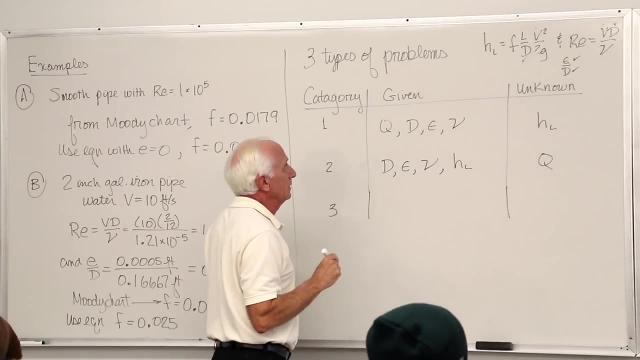 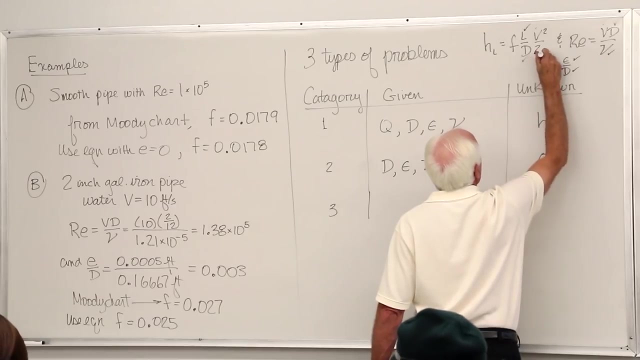 Okay, So I know E over D Got it. I know diameter, So I know the relative roughness. I do know kinematic viscosity. Nu, I know the pipe length, L. Oh, I know H sub L, H sub L. 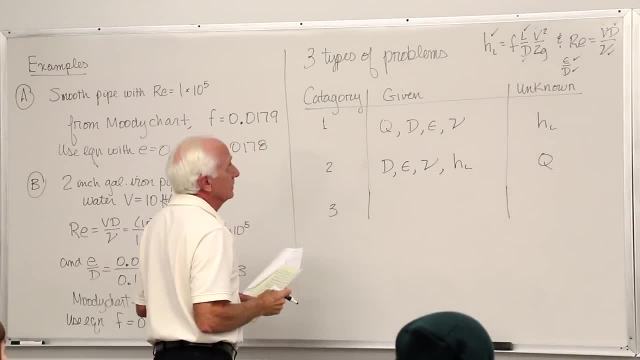 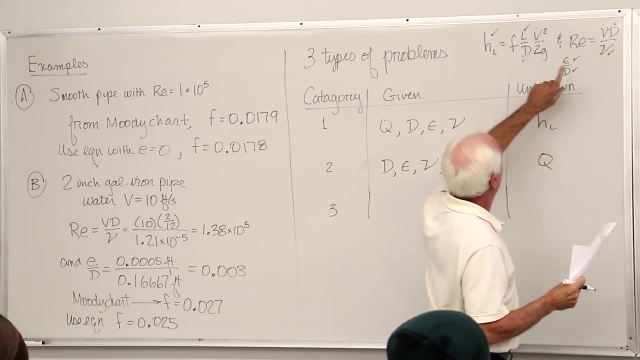 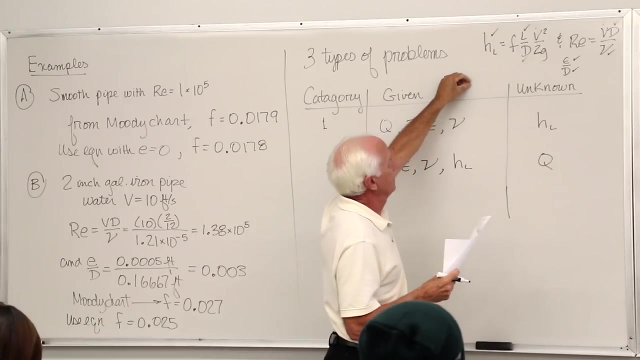 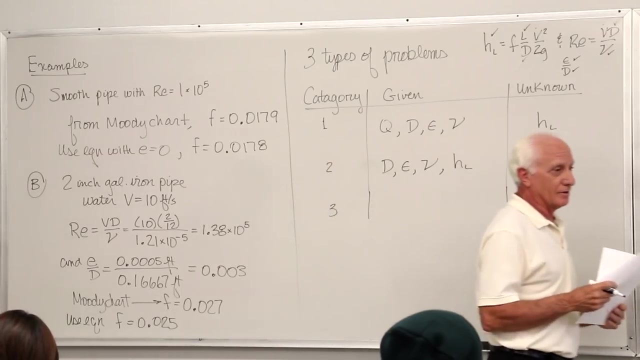 Okay, The Reynolds number. I don't know it because I don't know the velocity Here. The unknowns F and velocity. I don't know velocity. I can't solve for F or the velocity. Conclusion: Uh-oh. 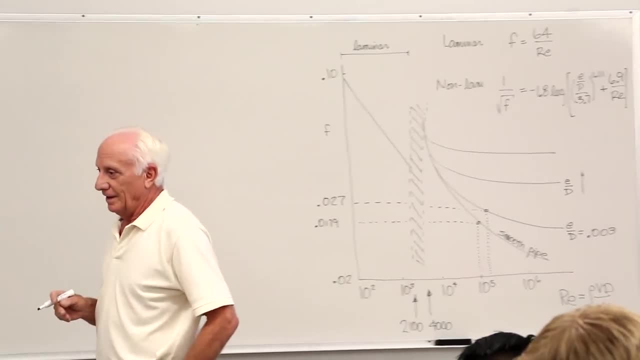 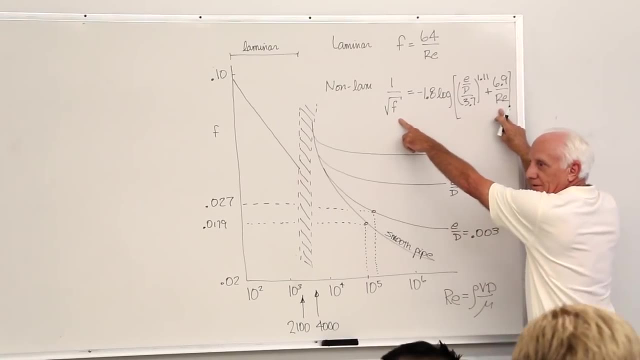 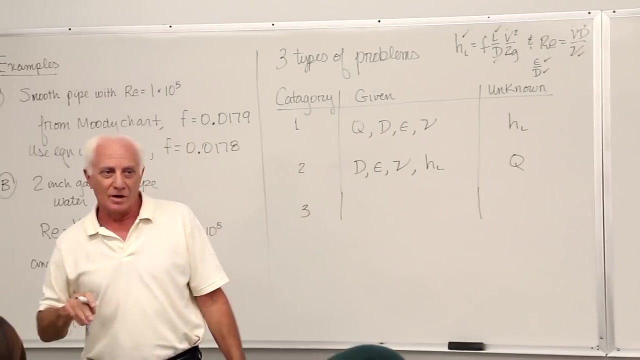 We got a problem. We don't know the Reynolds number. How do I use the Moody chart? or how do I use this if both these guys are unknown Can't solve that one equation. Okay, This is called a guessing game. If you don't know it, guess it and start the calculation, and it will be iterative in the end. 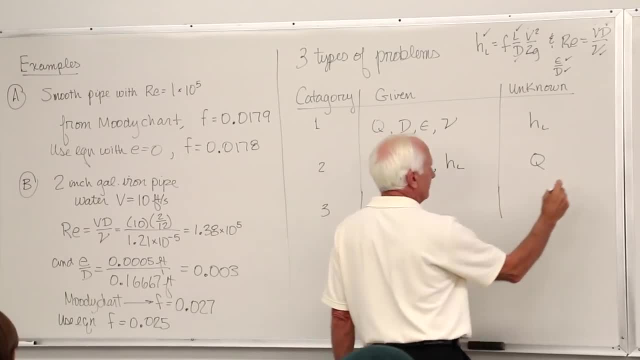 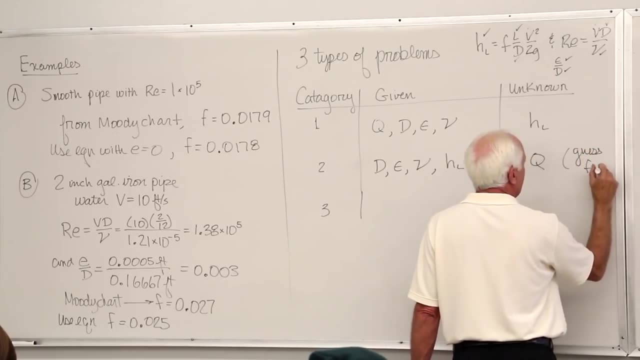 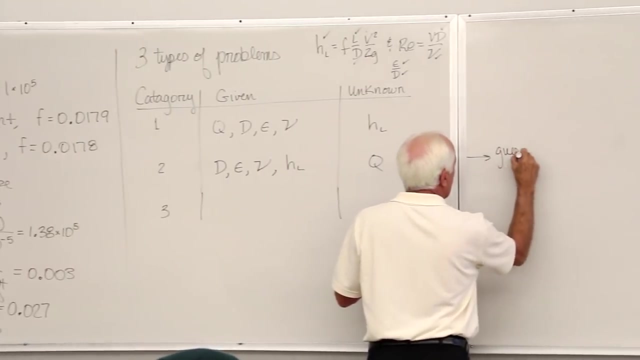 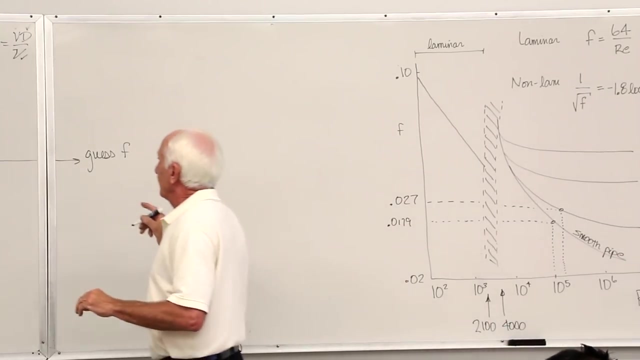 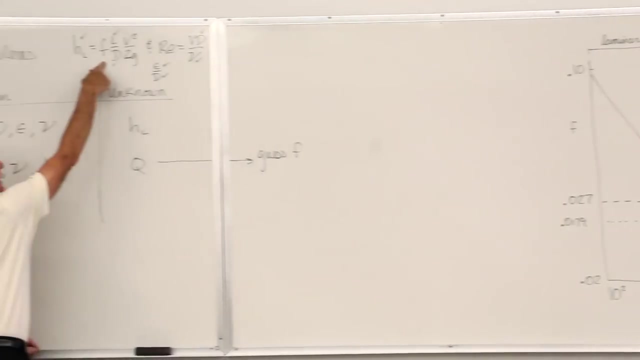 So I guess an F. This problem here is guess F. I'll just put it here over here. All right, I guess an F. If I guess an F from over here, I'll put the F up here. With that F guess, I'll calculate the velocity. 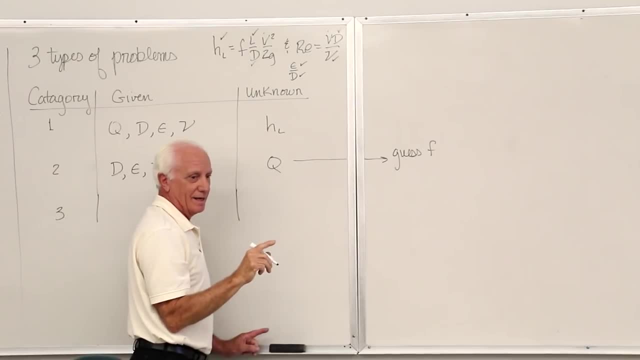 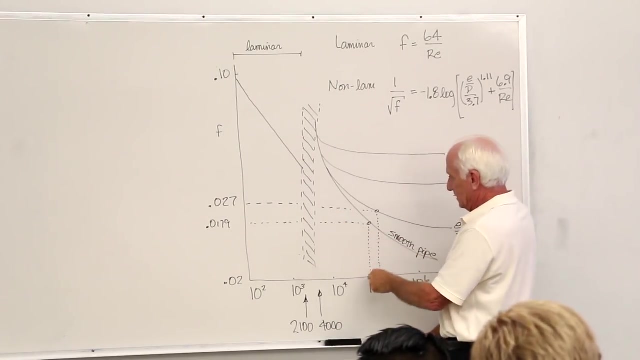 With the velocity I'll calculate the Reynolds number. Okay, I guess the F and I can now find the Reynolds number and F. But take the Reynolds number, Go over here With that Reynolds number you got with the F guess. Go up to the E over D line. 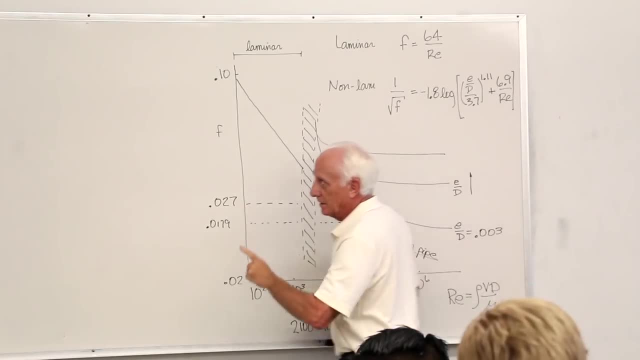 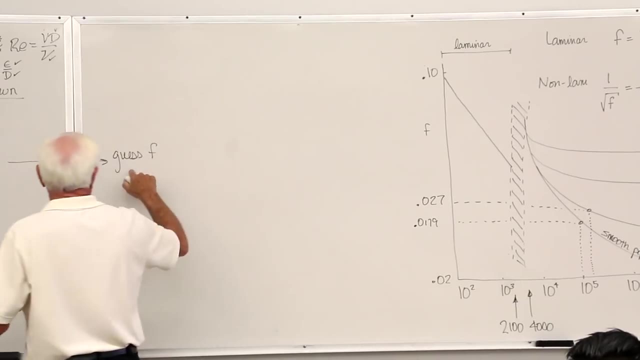 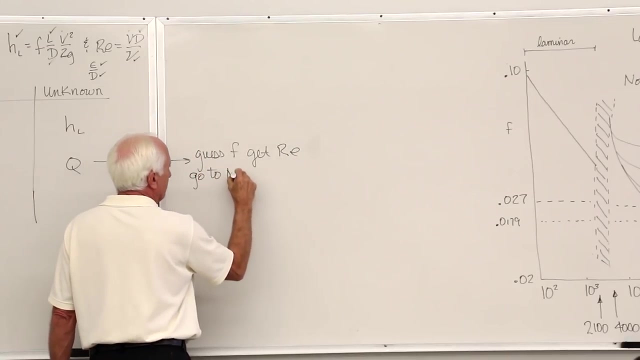 Go across. If the F you get doesn't match the F you guessed, try, try again. Repeat it with that new F. guess F. get Reynolds Go to Moody Find F. If they don't agree, repeat above until F converges. 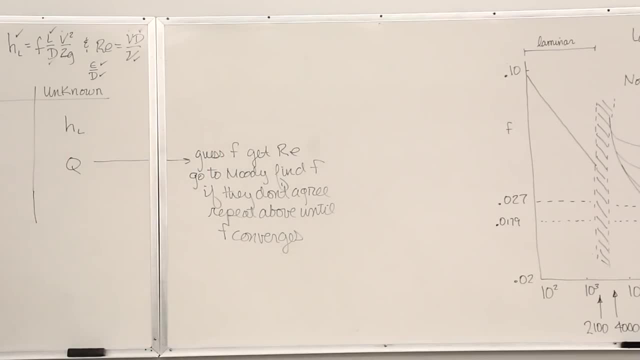 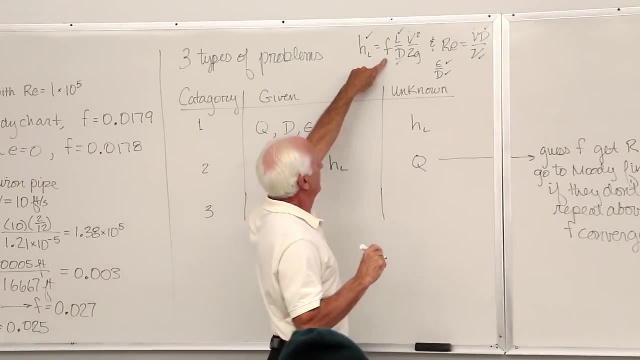 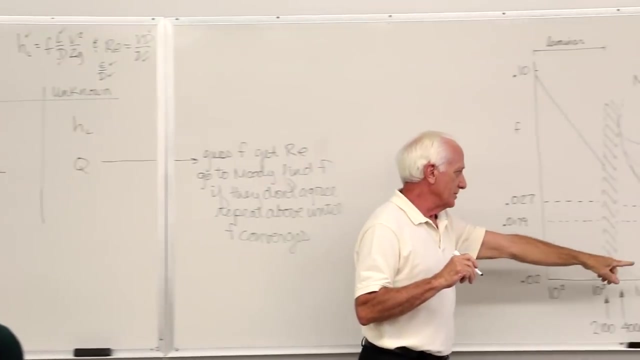 It's an iterative solution. You guess F from the Moody chart. You put the F in up here. You get the velocity. You put the velocity in the Reynolds number. Now go back to the Moody chart with that Reynolds number and that E over D. 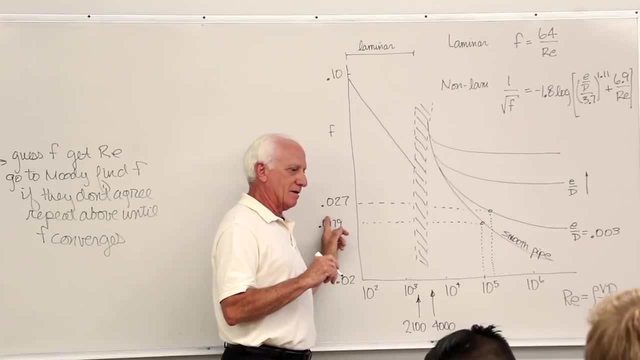 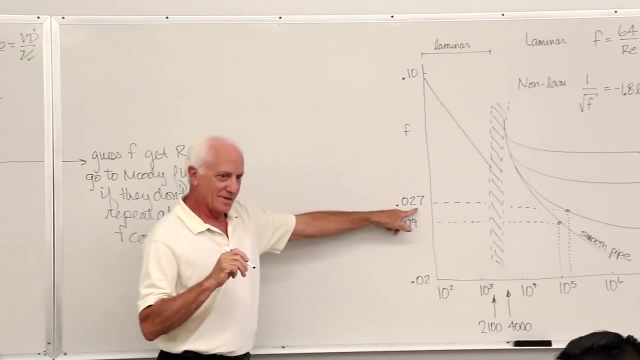 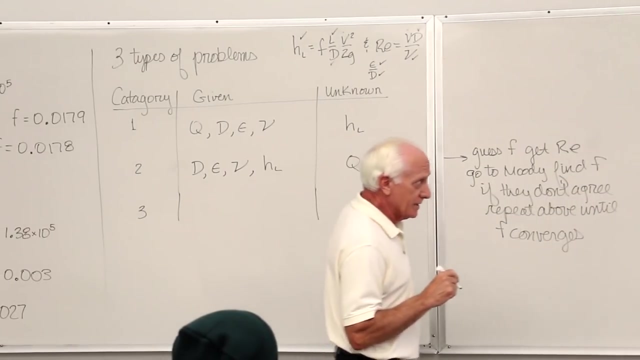 See what F comes out. If the F that comes out of the Moody chart doesn't agree with the F you guessed, repeat the calculation with the second F. The second F you got. It'll eventually converge. Where do you want to guess F? 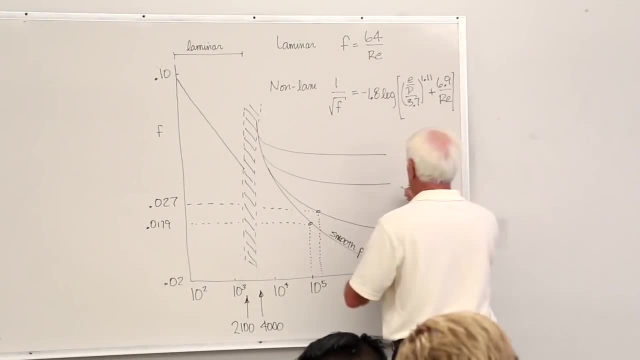 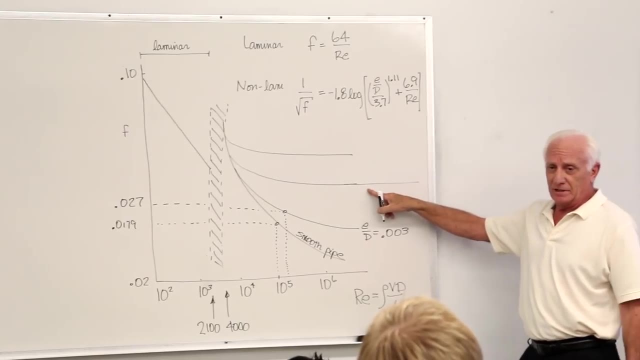 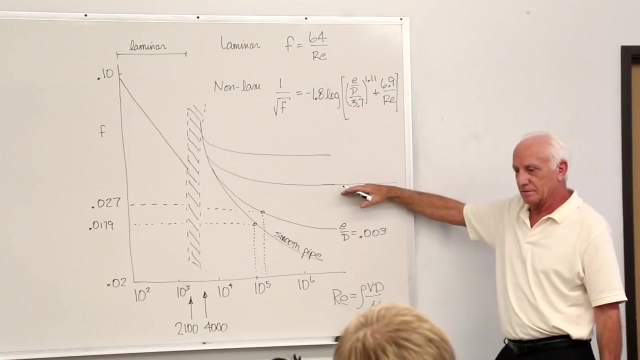 Well, let's say you're on this line right here: E over D. There's an E over D line. What am I going to guess for F? I'm going to play the odds. I think it's really turbulent. I'm going to guess F where that line is horizontal or flat. 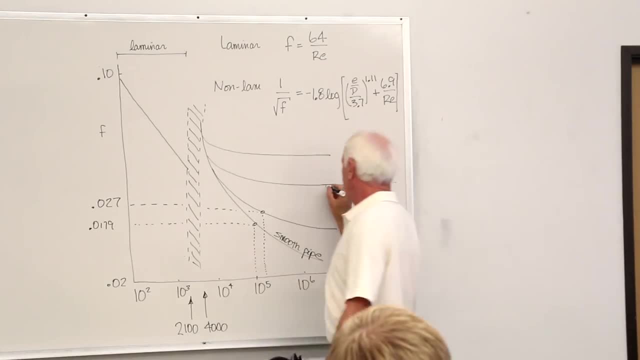 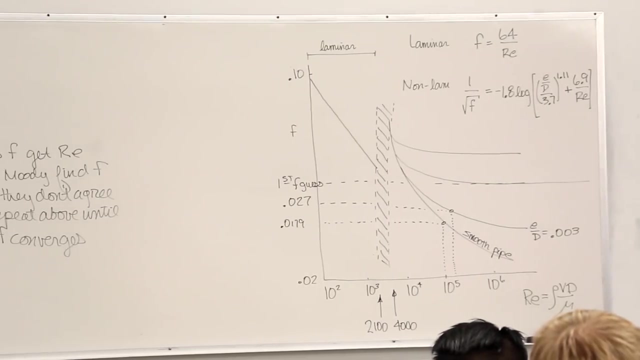 That's my first F guess. So I go back here- And that's my first F guess- Where the E over D line becomes horizontal. You're playing the odds. You think it's going to be turbulent, really turbulent, Why not? 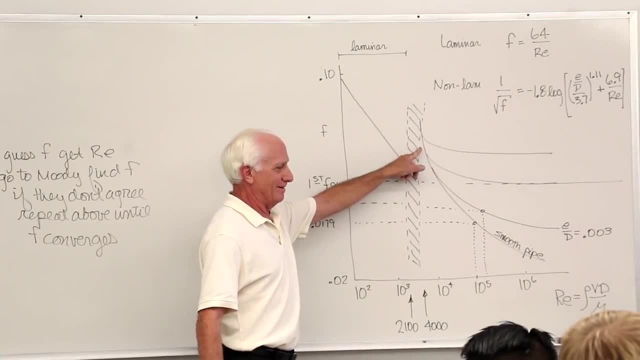 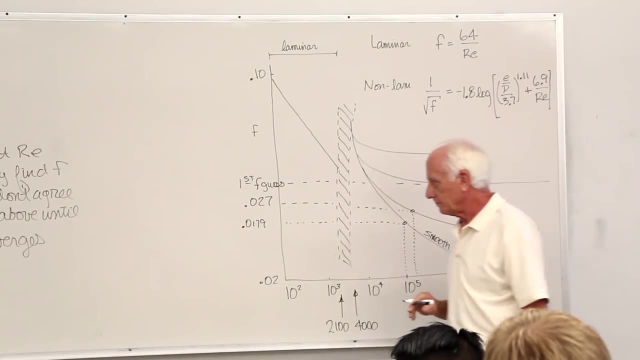 Why guess there? Why guess there? It's probably going to be out here somewhere. If not, that's okay, We'll converge One or two times. We'll converge. What if it's a smooth pipe? If it's a smooth pipe, all bets are off. 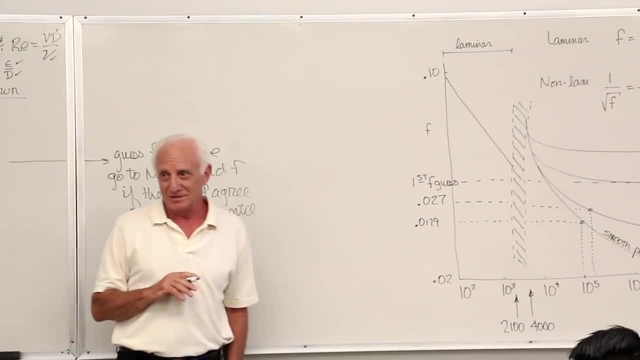 Does it ever get horizontal? No, What's a good F guess? Well, I don't care, You know. lower your eyes and walk up there. There, I think, right there, That's good Conclusion. A good F guess for smooth pipe is probably in the middle from here to here. 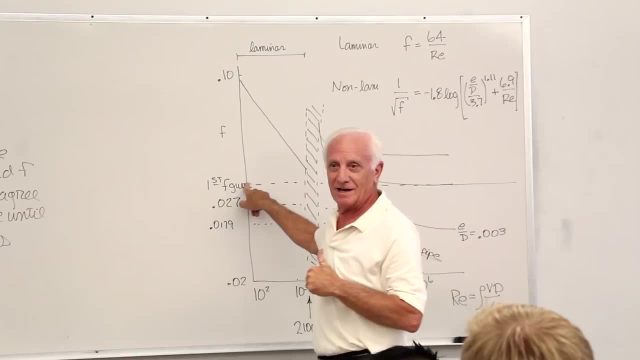 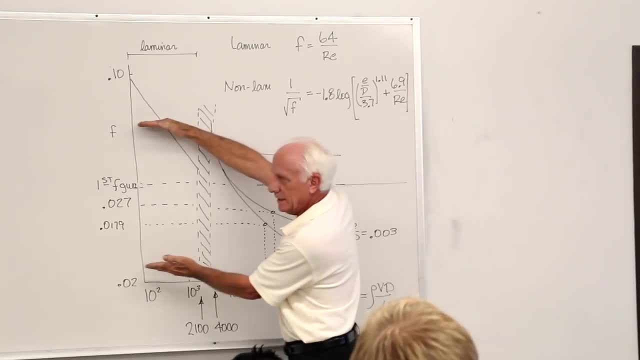 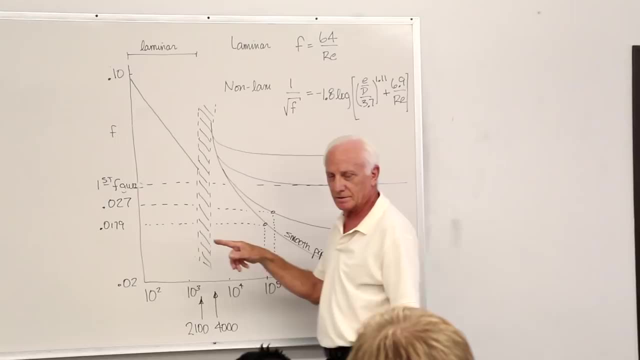 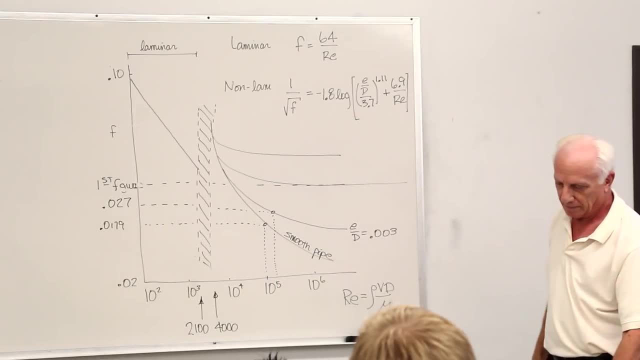 It won't matter, It's going to be your two, It's going to be your two anyway. Yeah, It's like say, on the first try you got lucky and your answer is like really close, Mmhmm, to what it is. 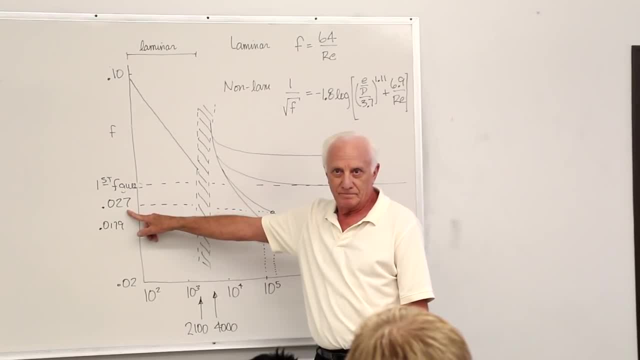 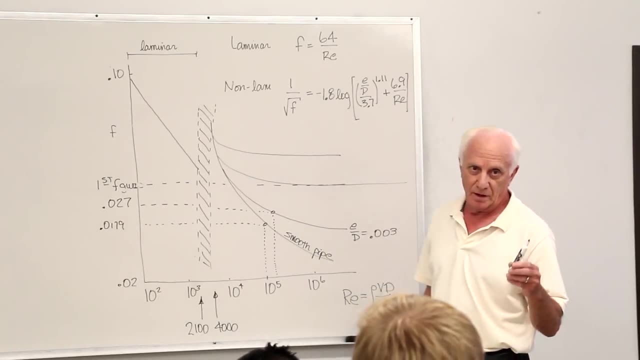 If you're within .001, stop. Okay, .001.. That's the readability of the Moody chart. Okay, Stop. Now here's the deal On an exam situation. I don't want you to get a rating. That's not what you need. 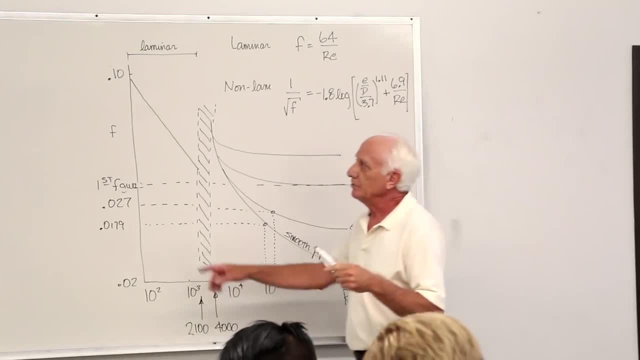 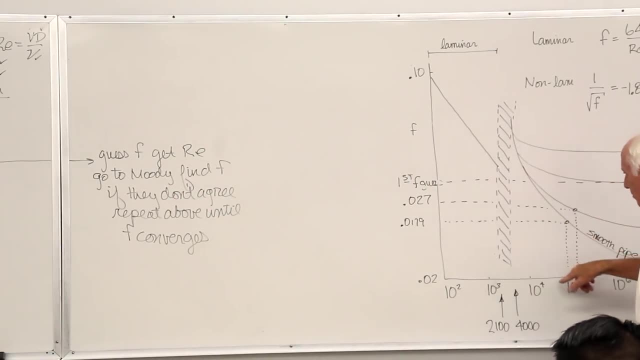 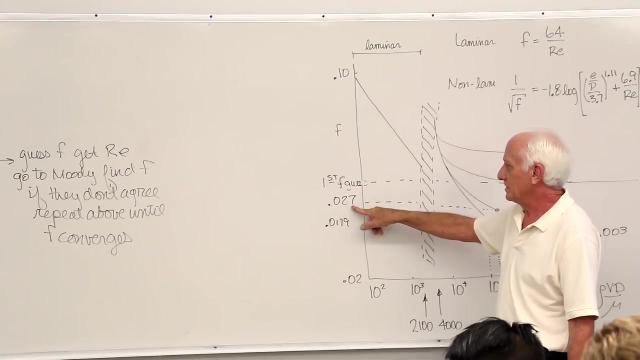 times too much of a factor on exam situation. you tell me what your first guess is. you go through it one time. go to the moody chart. you find out what the F comes out it. it didn't agree with my F guess. you say one, oh two, seven, didn't. 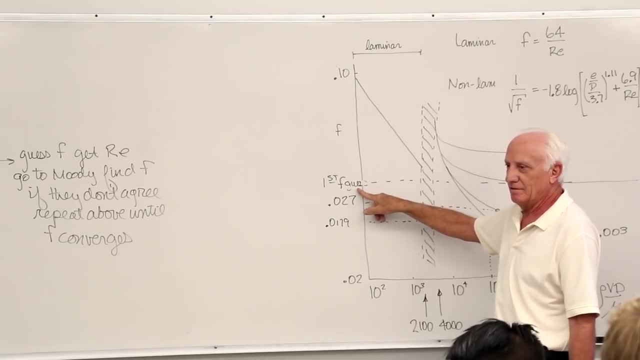 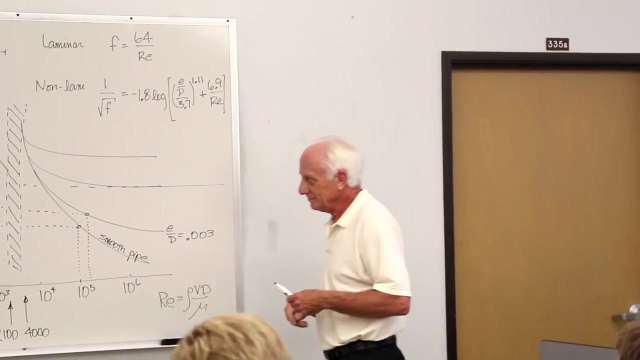 agree with my first F guess, point oh three, oh, I would repeat the above calculations based on: tell me what to do. based on point oh two, seven. but don't do any more work, don't iterate, but go through it one time to prove to me you know what you're doing in the iteration process. okay, all right, let's do the last. 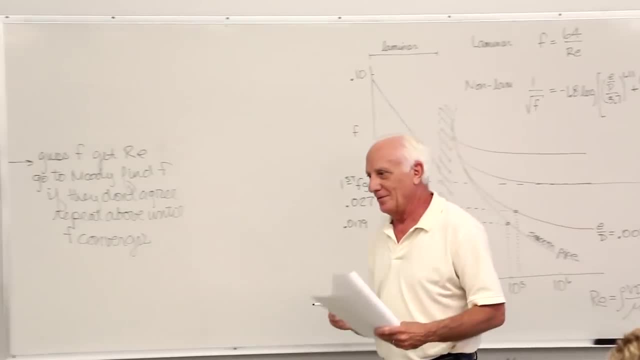 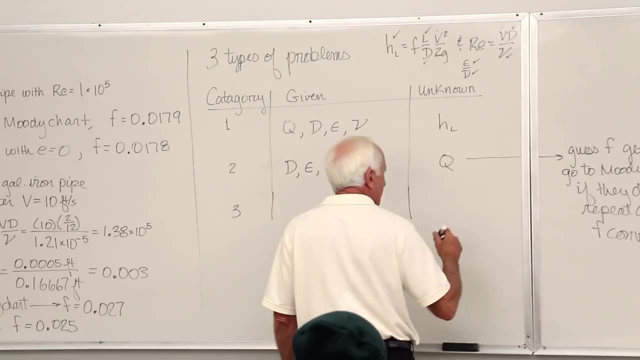 one, then the last one. no, somebody said how big should the pipe be to carry this oil, with a pressure drop of a thousand of pascals per meter. so you don't know how big the pipe gunner is. so what do you know? you know Q. 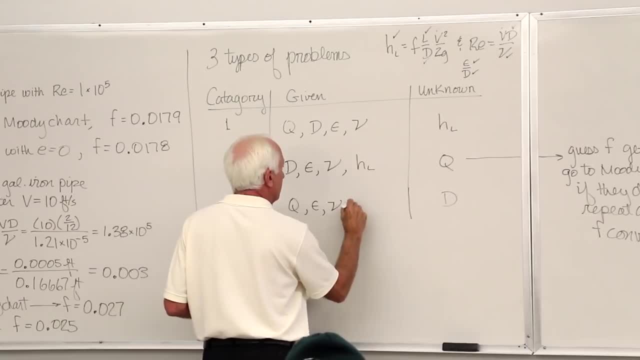 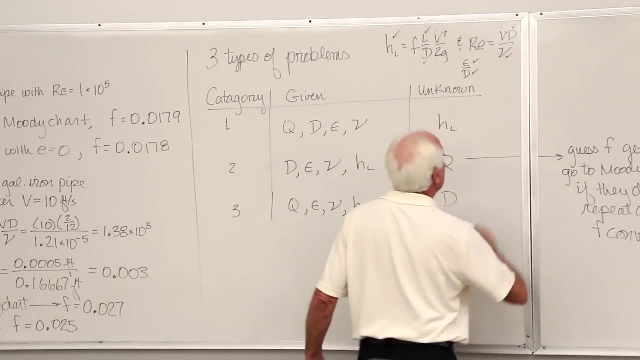 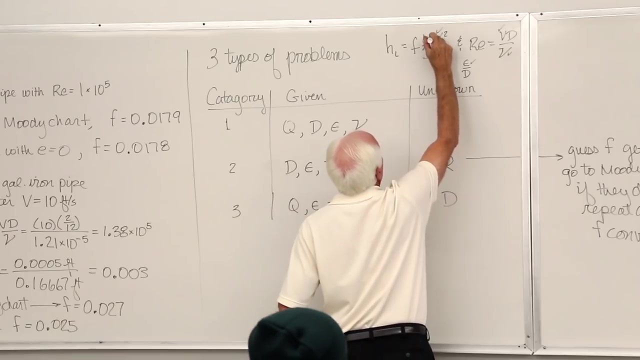 Q, E, NU, H, L. that's it. I don't know diameter. play the game again I. I don't know the diameter, I know E, I know NU, I know B, I know V, I don't know D, I know L, I don't know F. how do you know V? 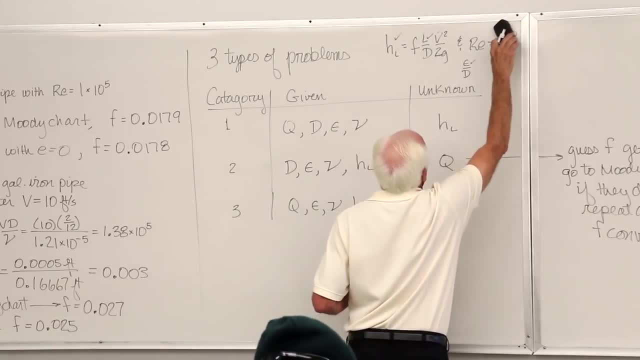 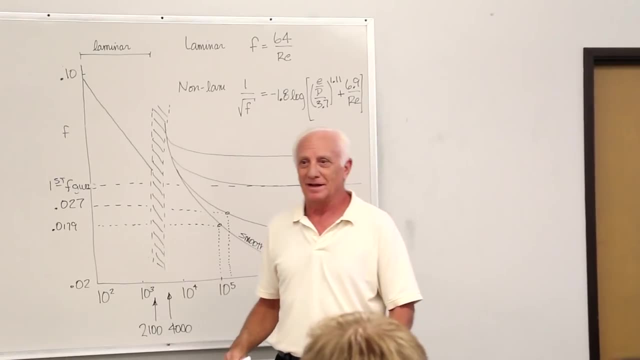 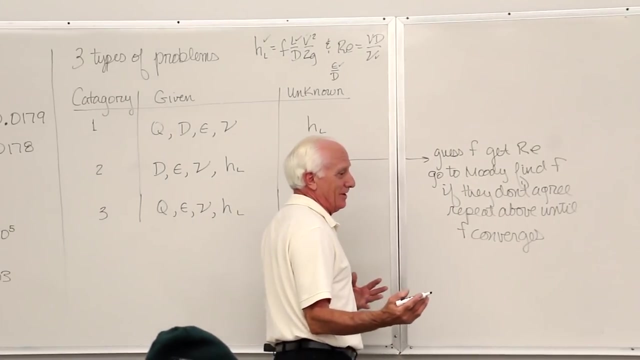 yeah, don't know V things. I need my. okay, now we get to the real guessing game. okay, let's start this thing and you even what you might want to do. you can get deep. any say, you can guess what you want. you can guess. you know what were the. 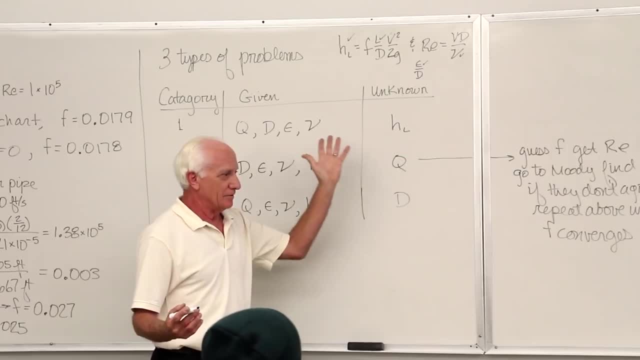 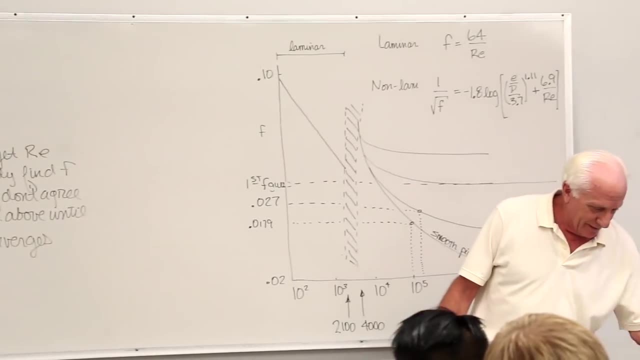 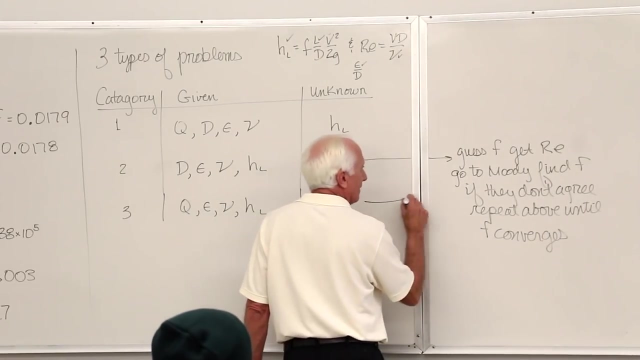 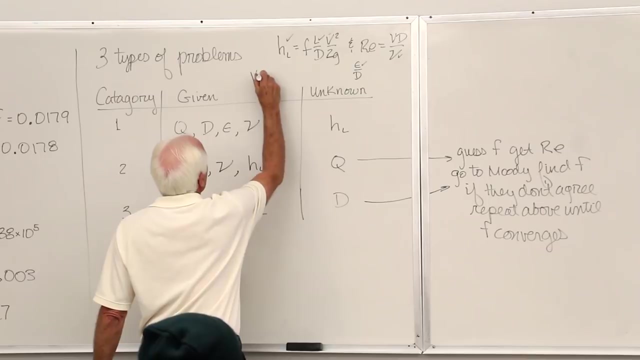 unknowns. before the Q and the F and so on, just guess something in this particular particular case. Let's see what I guessed on this guy. I guessed F again. so there's a reason why Guess D. I've got it. I've got it. Put it in there, Okay, I. 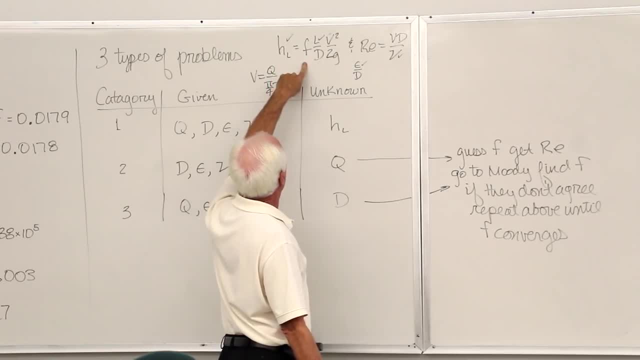 know HL. Okay, I know HL. Oh, I know HL. Okay, So I can guess that On your F, you can guess F again, or you can guess D. What are you going to guess for a pipe? What's a possible diameter? I don't know, Maybe an eighth of an inch to 36. 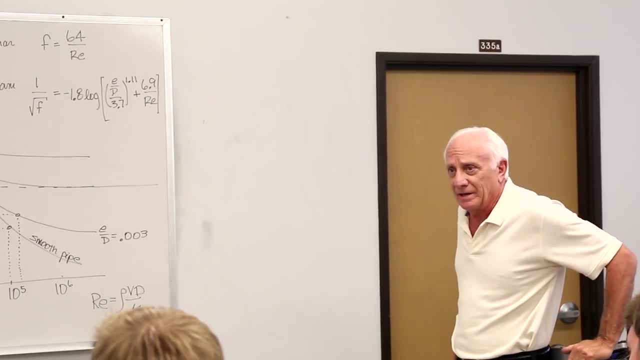 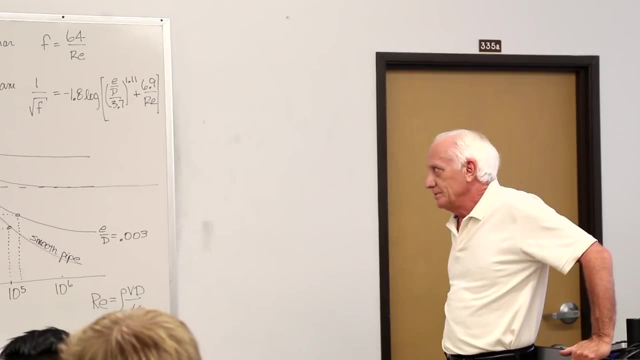 feet. Wow, That's a wild guess. You'd be converging for hours. No, it's easier to guess F on the Moody chart. Just pick a middle value. I don't know what D is. I don't know what Reynolds number is. What's my first guess? I? 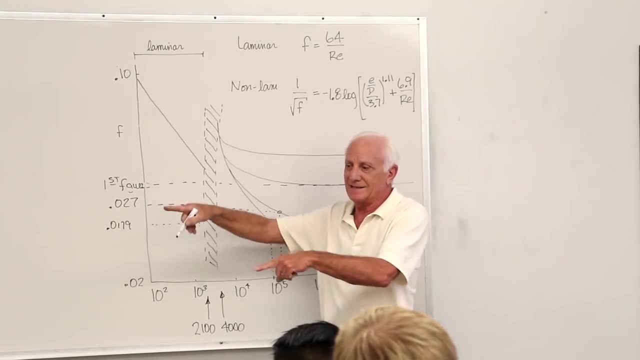 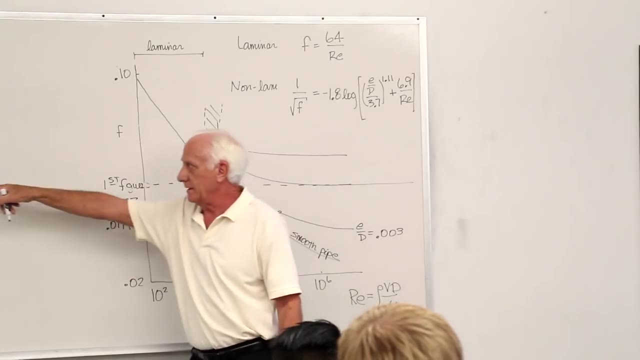 don't know, 0.030.. Fine, Once I guess that I can come back to the Moody chart. get a Reynolds number, get an E over D, come up here, go over there, get an F and check it against my F guess here. So that's a little more difficult iterative. 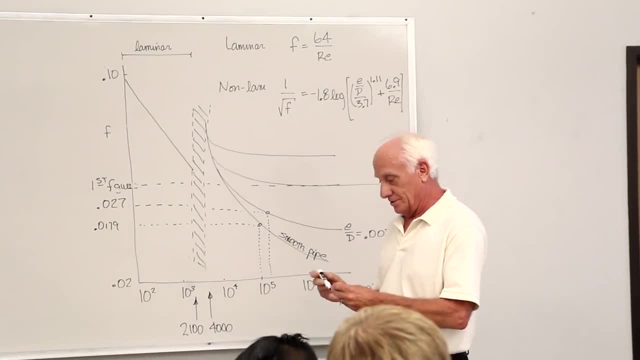 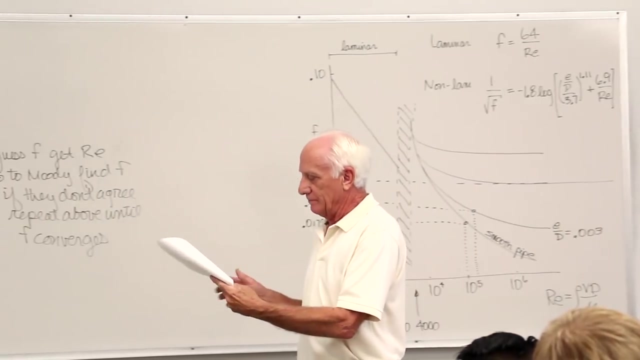 process, But one that occurs, you know, it occurs in the real world. How big a pipe should I specify for that job? Okay, So anyway, that's the part two of what I gave you. So here's what I gave you last time On the handle. I gave you Example. 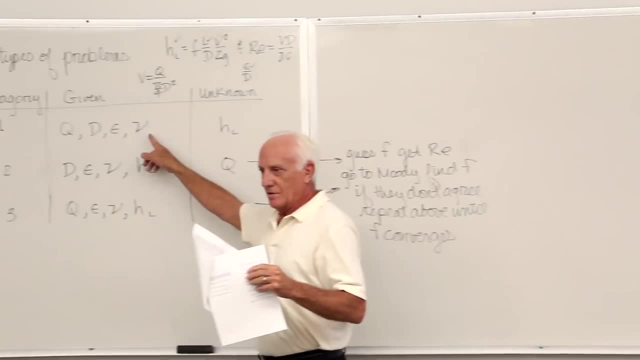 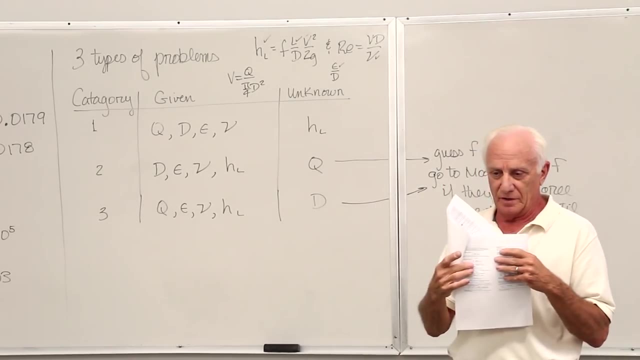 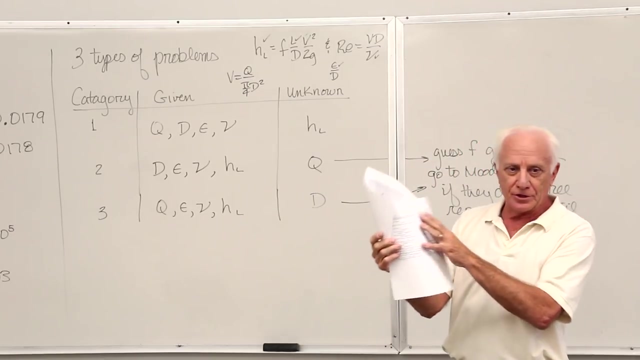 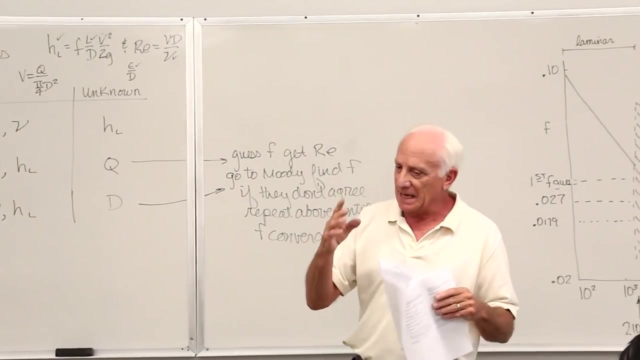 711 is category one problem. Example 712 is a category two problem, So I'm going to give you an example. Example 713, on the handout, is a category three problem. So you have an example of every one of these three problems to follow. Now here's. 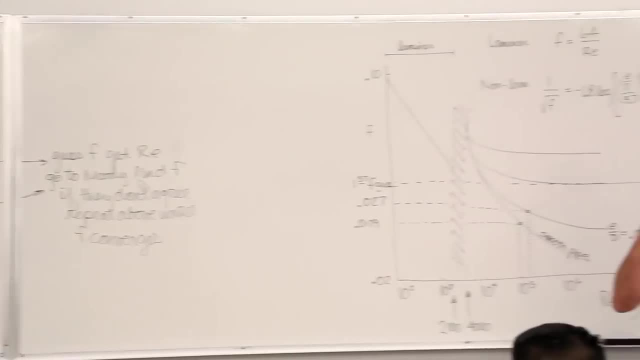 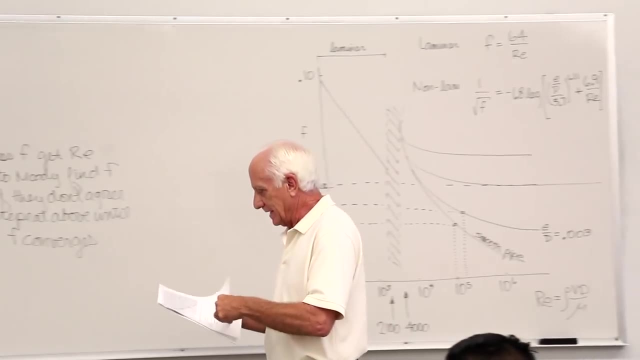 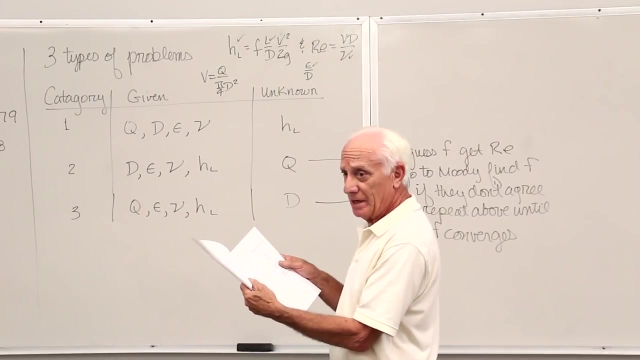 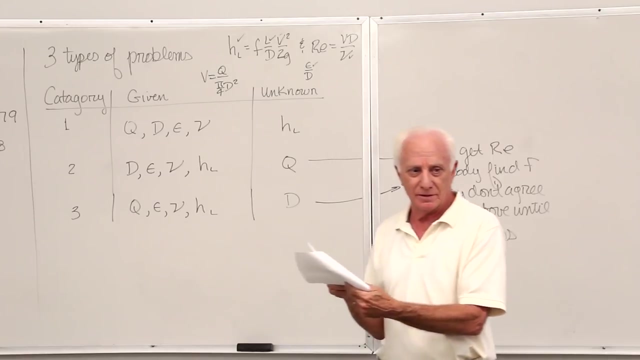 the good news On F, page two, on the right left-hand column. ooh, read it here. An alternative to using the Moody diagram that avoids any trial and error process is made possible by empirically-derived formulas. Now empirical means comes from: 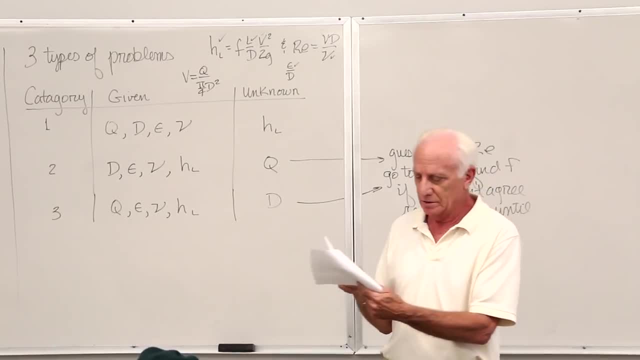 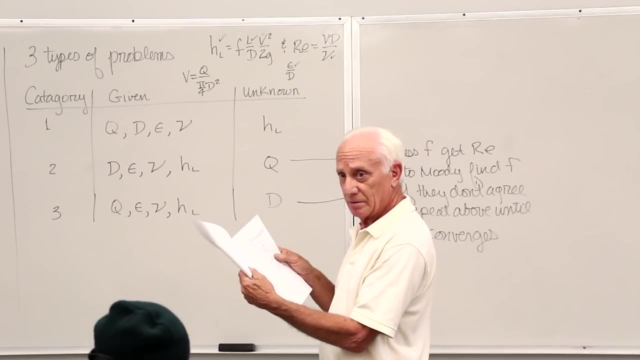 observation, They're not derived theoretically Empirical, Presented by Swamy and Jane 1976.. And this appears in our current textbook. It's a long time ago but they still work For pipe flow, an explicit expression of the. 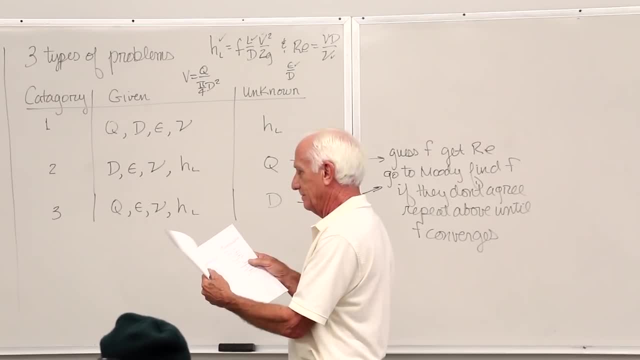 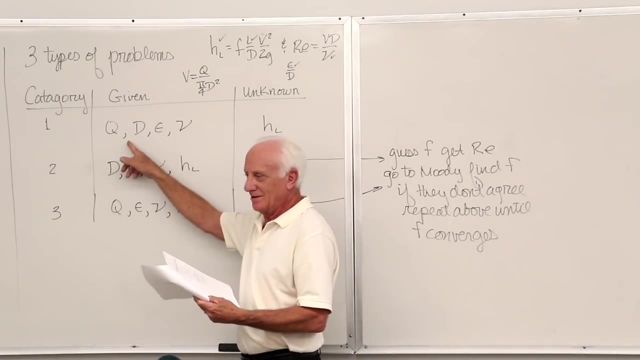 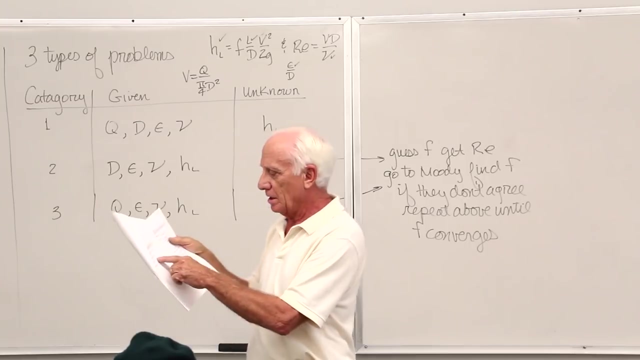 expression that provides an approximate value for the unknown in each category problem. So you've got three equations: One equation that works for category one, One equation works for category two, One equation works for category three And it tells you when they work. Category three problem E over D must be between 1 times. 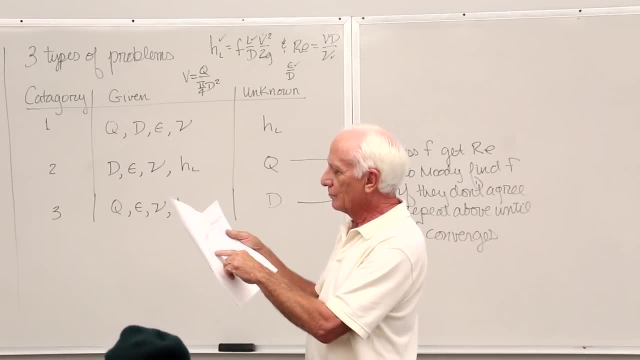 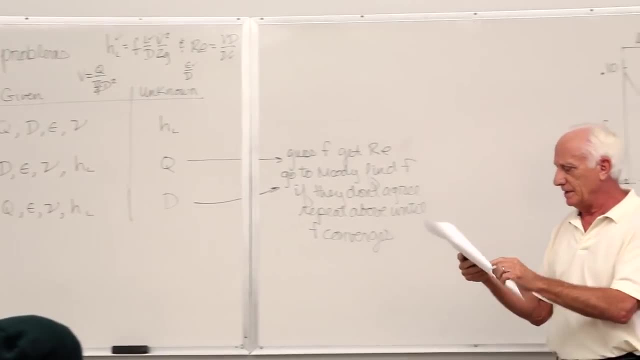 10 to the minus 6 and 1 times 10 to the minus 2.. Reynolds number must be between 5 times 10 to the 3 and 3 times 10 to the 8.. Ooh, that's a big region, That's a big. 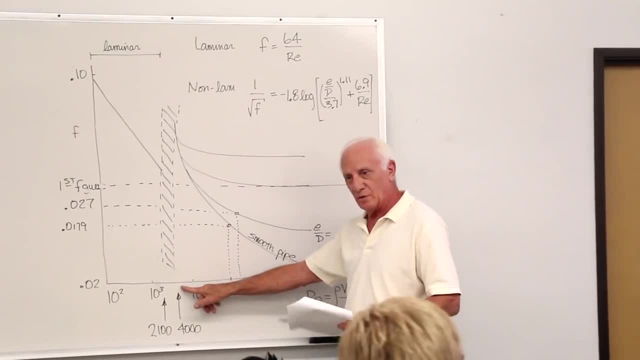 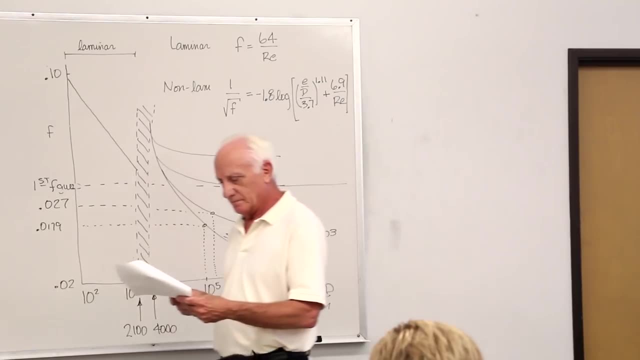 region: 5,000.. 5 times 10 to the 3rd, Right here, All the way where To 10 to the 8. Way out here. That's a good, that's a good thing. And it says below that. it says: 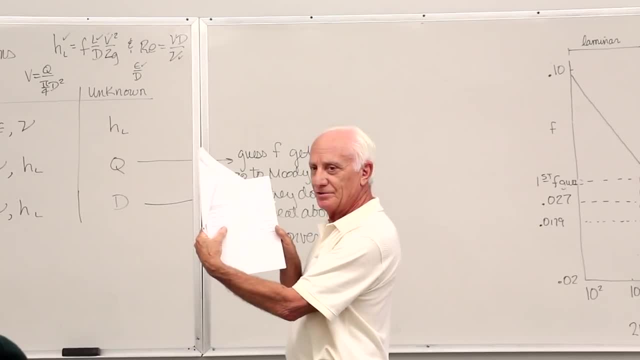 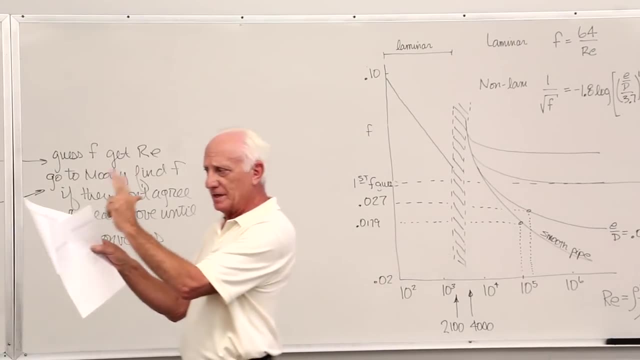 and, by the way, you can use either English or SI in these equations. You can use either English or SI in these equations. And then the examples I gave you. I told you, I gave you three examples. First of all, they work it by guessing and the Moody. 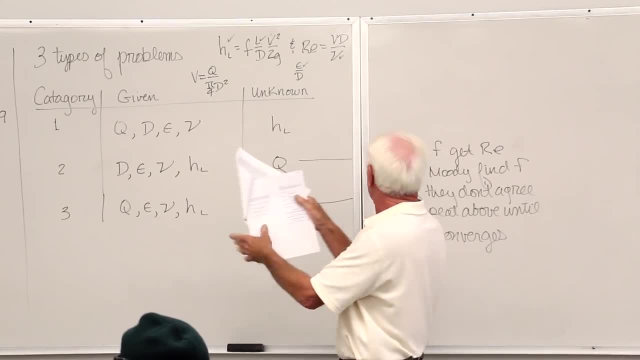 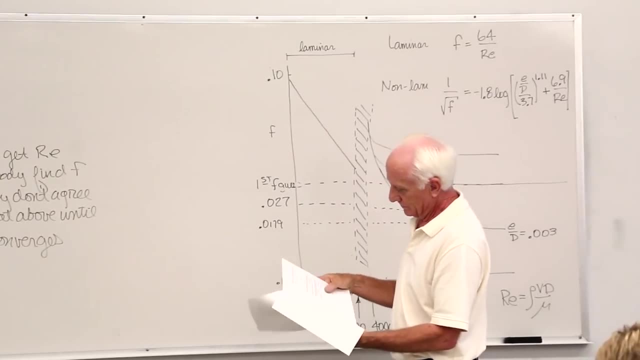 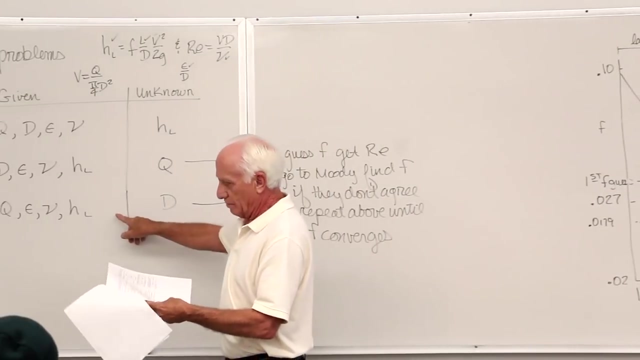 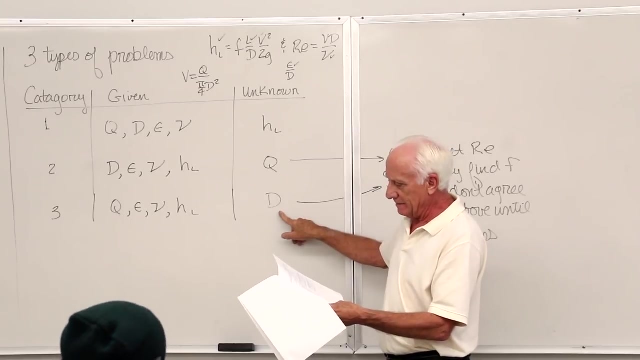 Chart. Second of all, they work it by the equations on here, This category problem, for instance, this example 7, 13.. They solve for what Diameter? If they do the guessing game on that, Their first guess guess what? 0.03.. What did I say? 0.03?. 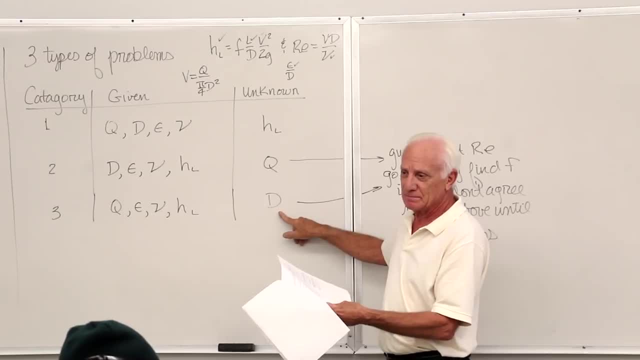 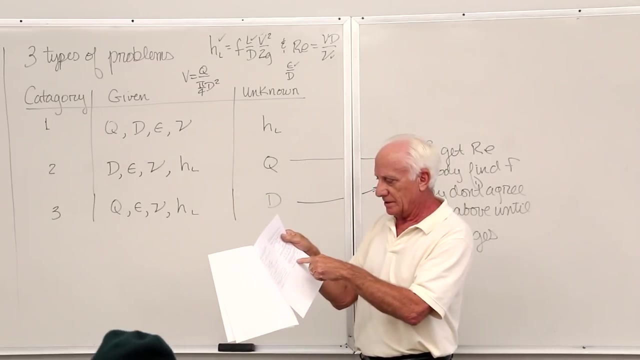 That's a good guess. You don't know anything. guess 0.03.. They guessed 0.03.. It converged in two iterations. It's on the handout. It converged in two iterations. What was the diameter? Four centimeters. Now put it in the approximate equation. 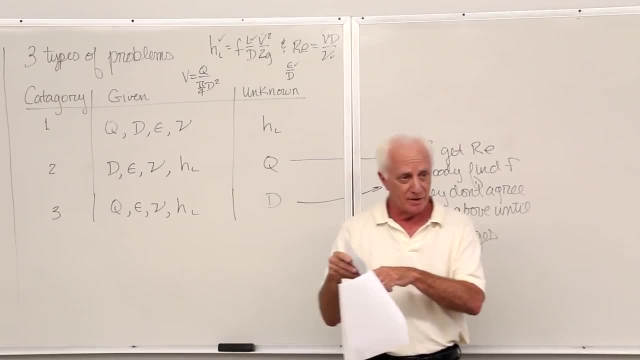 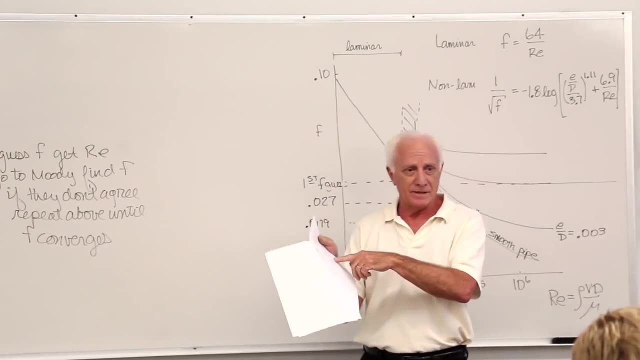 Guess what they get? No iteration required, 3.9 compared to four centimeters. Oh, of course it's close. Which one's right? Neither one's right. It says: right there the equations are approximate And we know the Moody chart's only accurate. 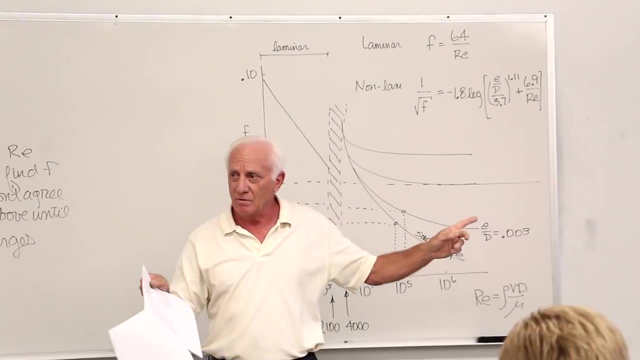 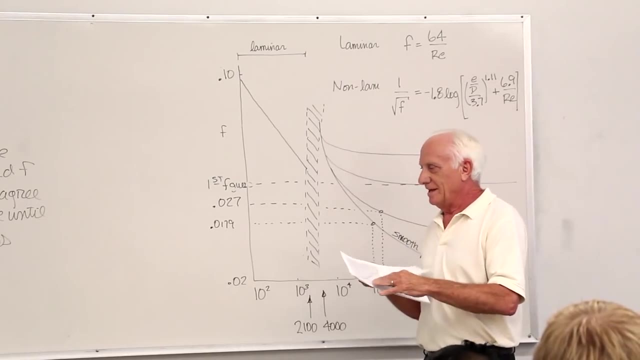 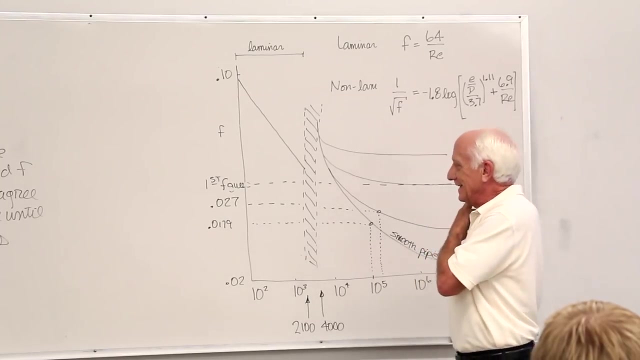 to 10%. 10% of four is what? 0.4? Wow, wow. So yeah, these guys are right on together. It gives you some confidence that in the equations will work with the iterative procedure, Okay. So you've got those possibilities okay. 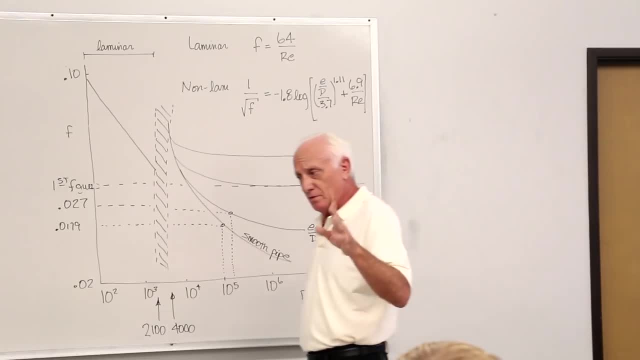 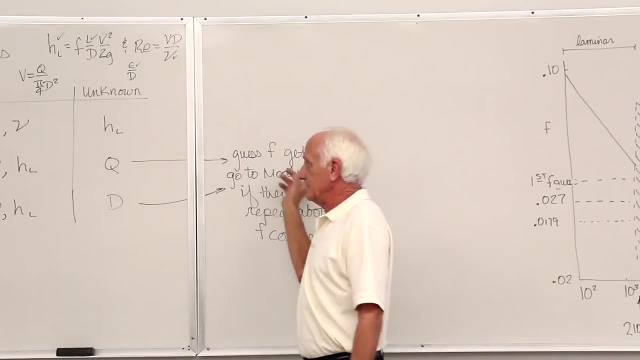 If I give you an exam problem like that, you can do one of two ways. You can use the equation, which is pretty complex, but you can use it, Or if you want to make one guess and then go through it one time and tell me what your next guess for F. 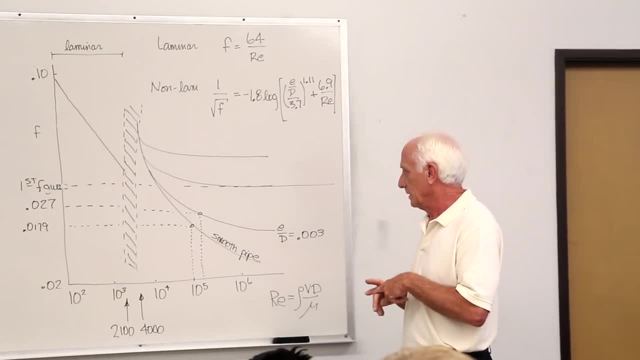 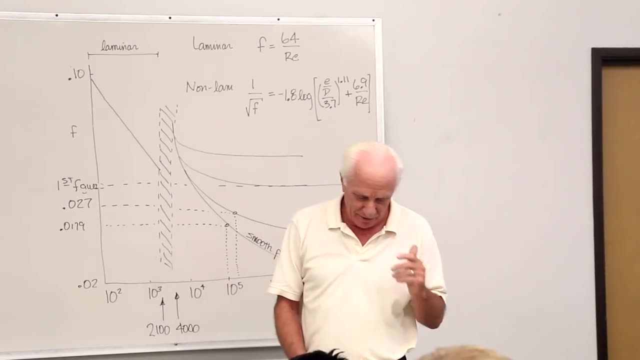 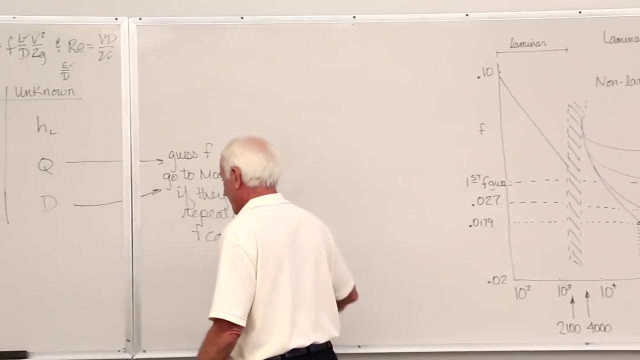 would be. that's fine, too, Your choice. Okay, Now, if you didn't get the handout last time, see me after class. I've got a couple extra copies here. All right, Now let's go back and see where we use this information. Okay, And you know, we use it. 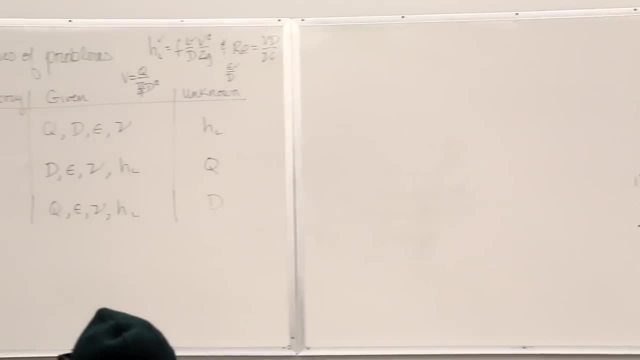 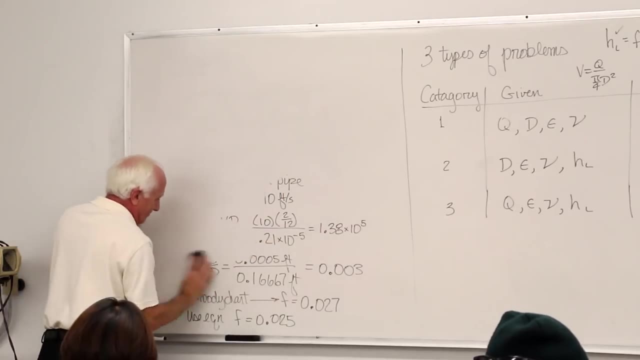 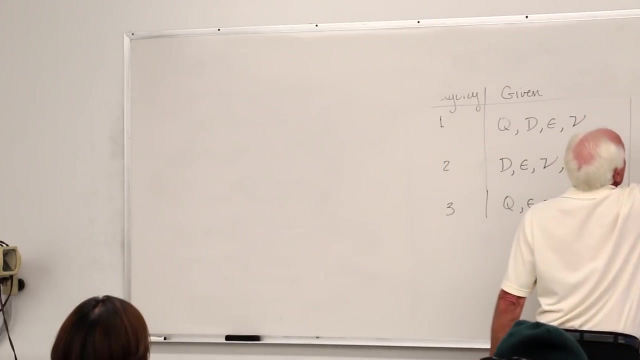 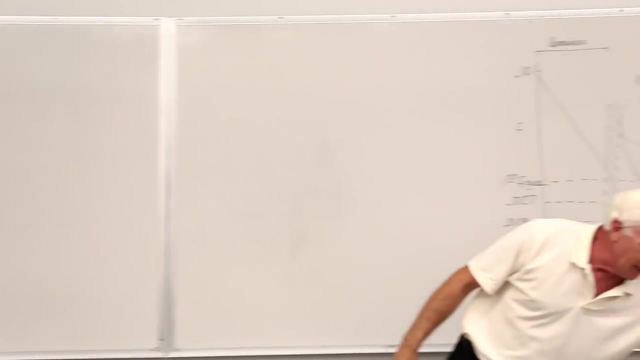 in the energy equation, So I think I'll put that over here. All right, Let's write out the head form of the energy equation one more time. All right, So we have our left-hand side energy added to the system, our. 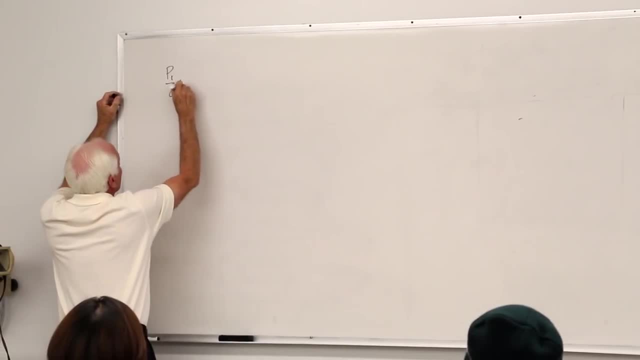 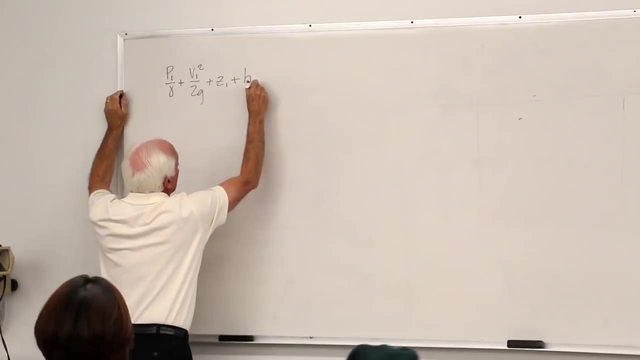 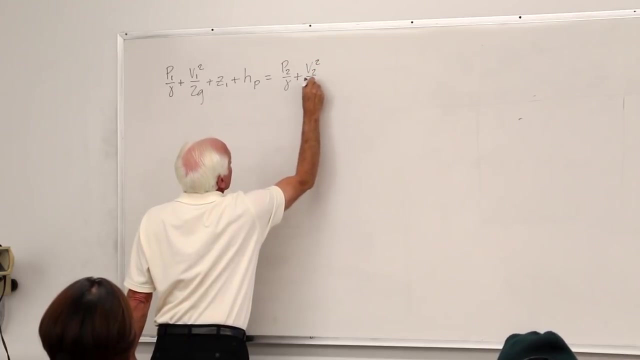 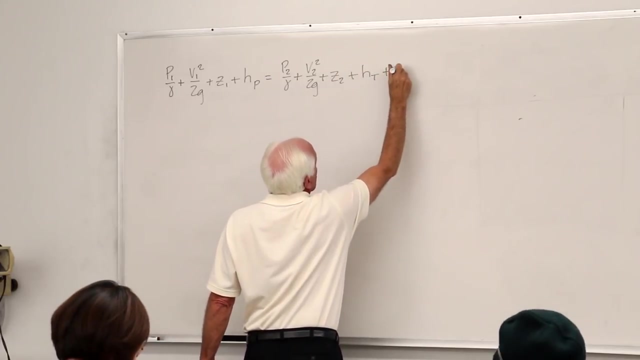 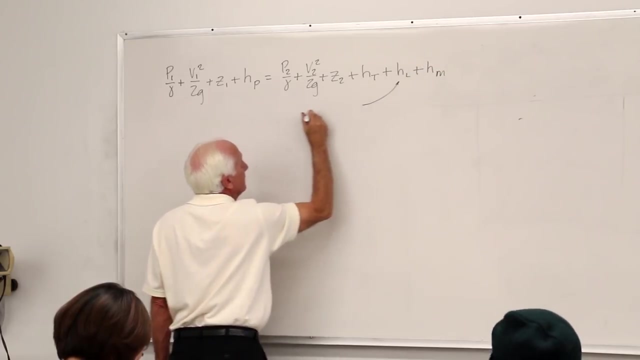 control line. So we have P1 over gamma, V1, squared Z1 plus the head divided by a pump subscript, two Turbine. if there's one Straight pipe, friction losses and minor losses. Just to remember again, That guy of course works for laminar or turbulent, Of course. 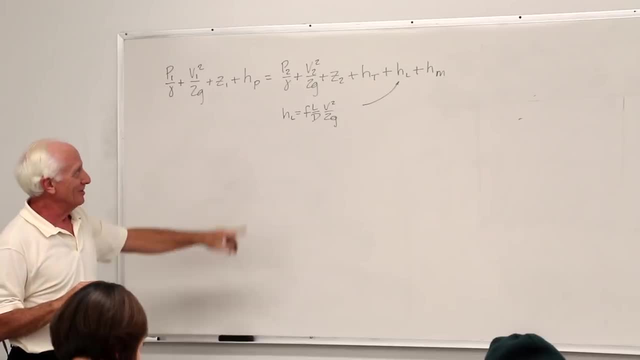 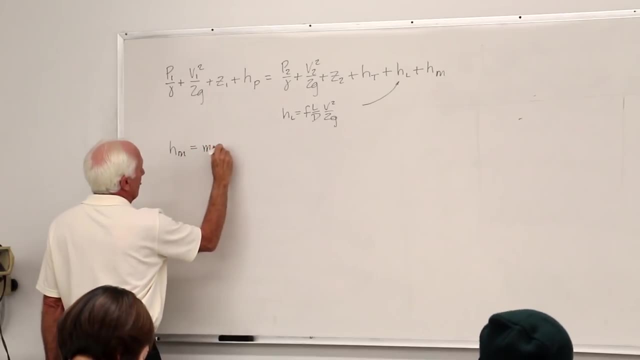 VF depends on laminar or turbulent, but the equation works for laminar or turbulent. Okay, We haven't done H. Okay, We haven't done H. HM. HM stands for minor losses. The reason why it's called minor losses is: 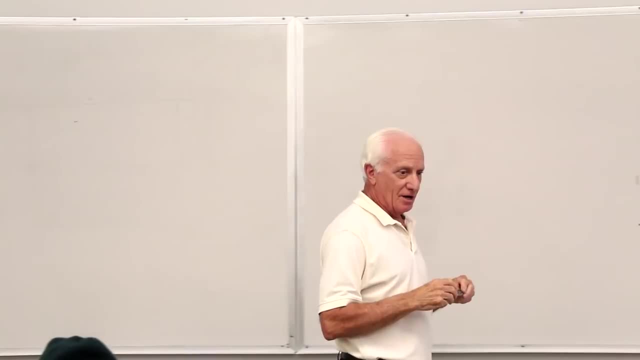 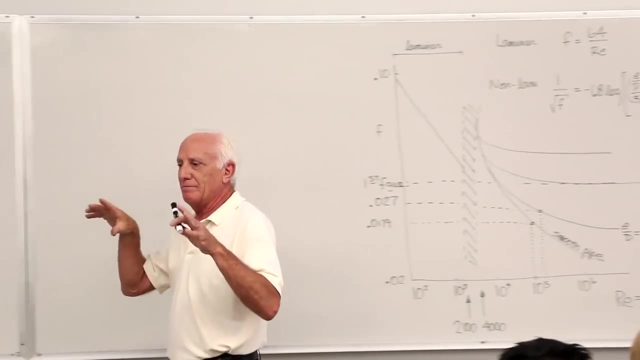 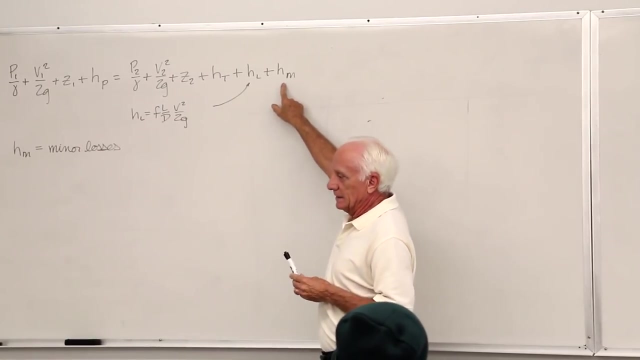 because for most large piping systems those losses are somewhat minor compared to the straight pipe friction losses. H sub L. Normally in a big pipe network, maybe a petrochemical plant, maybe a steam power plant, these guys are much, much less than H sub L. 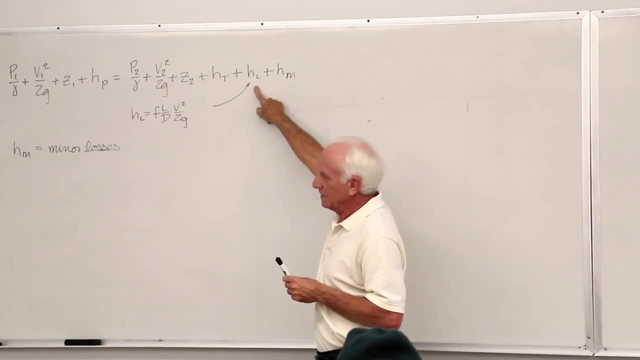 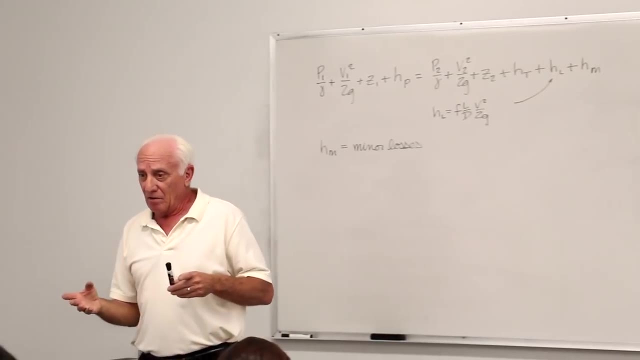 H sub L, Normally in a big pipe network, maybe a steam power plant, these guys are much, much less than this guy. This guy is a straight pipe friction loss. This guy is the loss due to fittings in a pipe: an elbow, a tee, a valve, things like that. So we'll 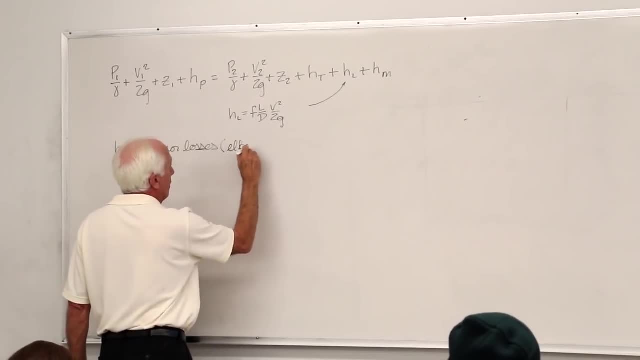 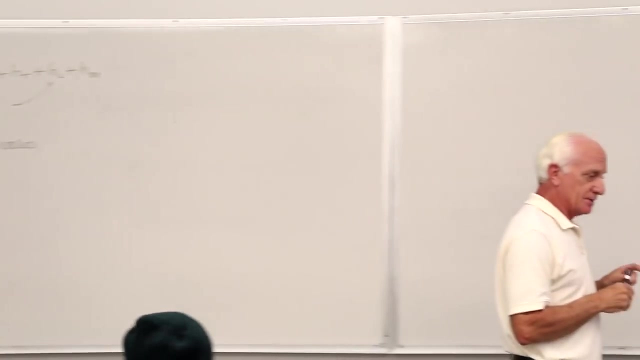 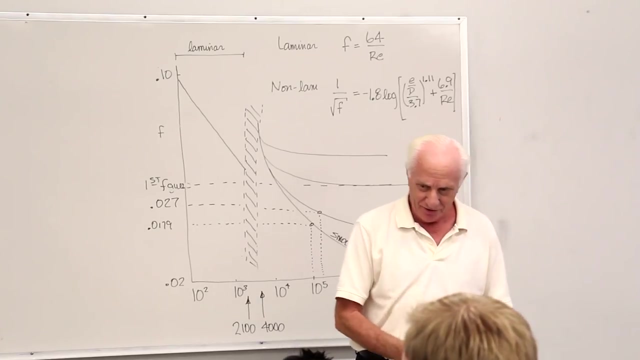 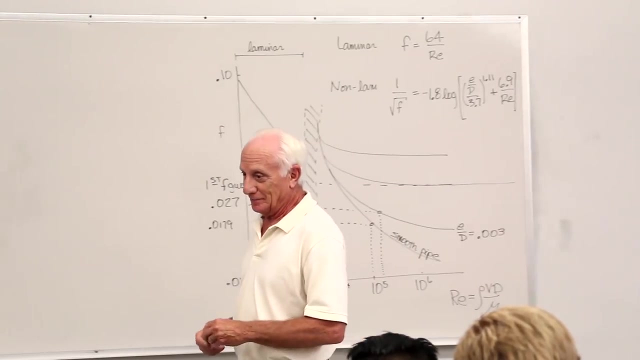 put down elbows, tees, valves, etc. Those are all components of the piping network which do add some resistance to the pipe flow and they're called the minor losses, which is a misnomer because many times they're pretty big, But because this stuff is done for larger. 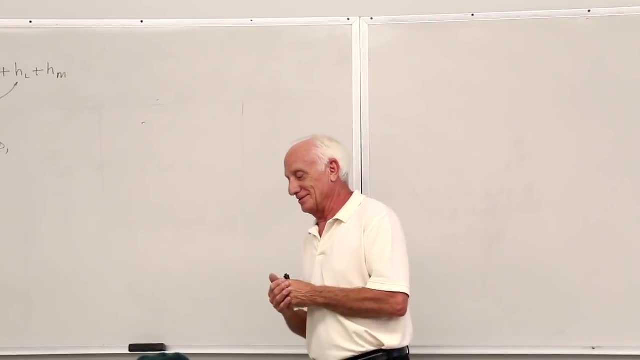 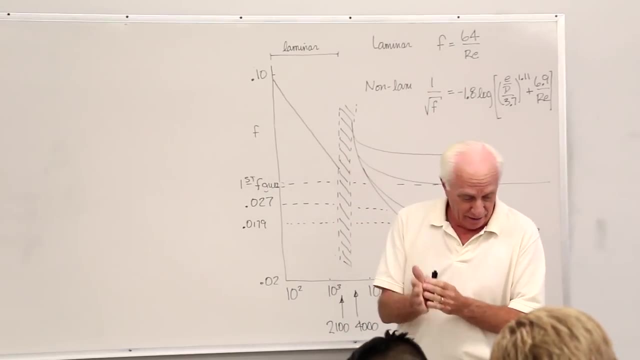 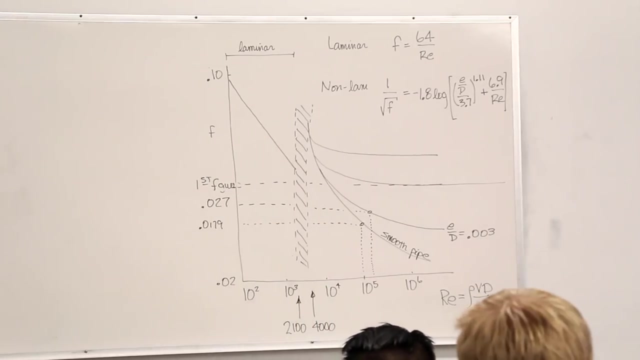 plants. typically they're minor losses, but they can be as big as HL. They can be as big as HL. Okay, Where do they come from? Okay, Well, here's a handout that shows you some of these guys. They're in your. 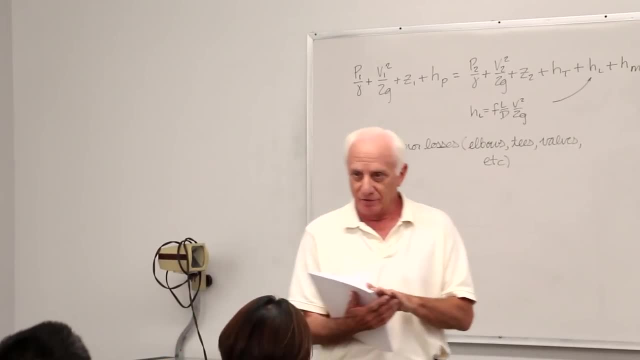 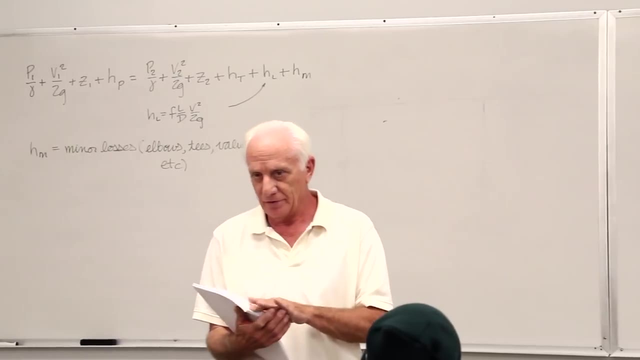 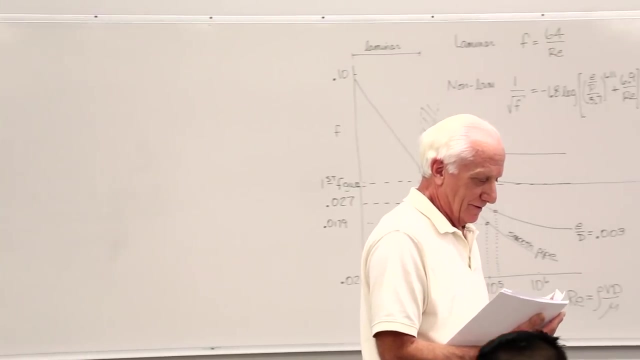 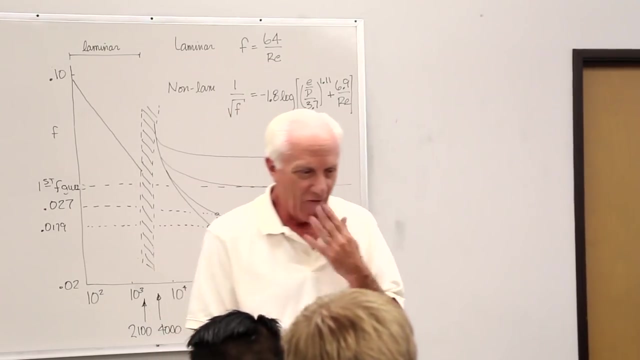 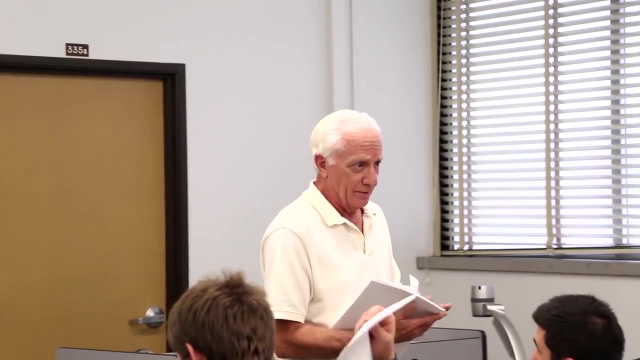 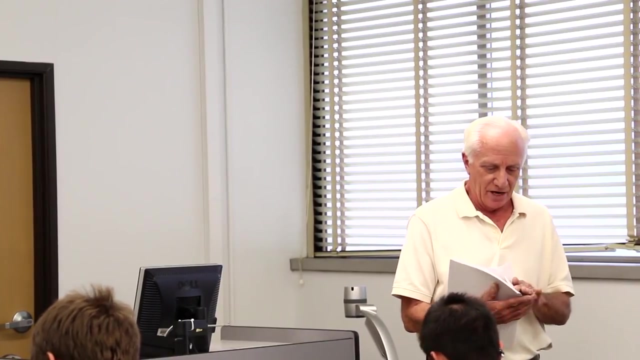 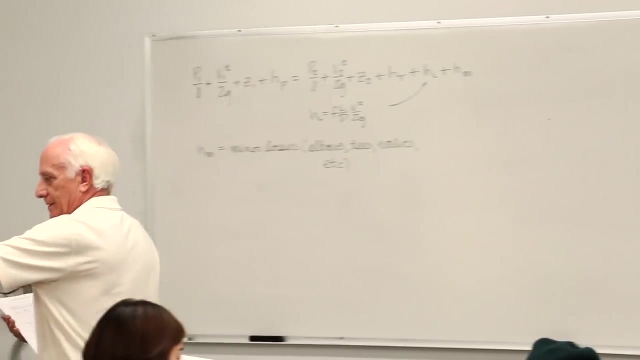 textbook. of course, too, You'll have them on the final exam. They're in your equation package I give you So they're available for you on the final. Don't put them on your equation sheet. One minute, Okay, I'll be back in a minute. I don't think this is the same table as in your textbook. I like this one better, but the one on the exams handout equation package is, I think, on your textbook. Let's see One more over there. We're going to work the example of 715 just a minute. 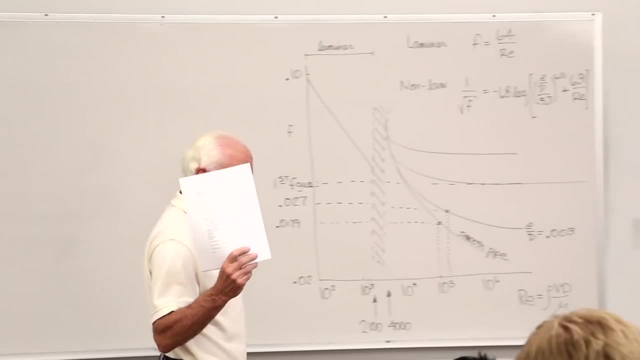 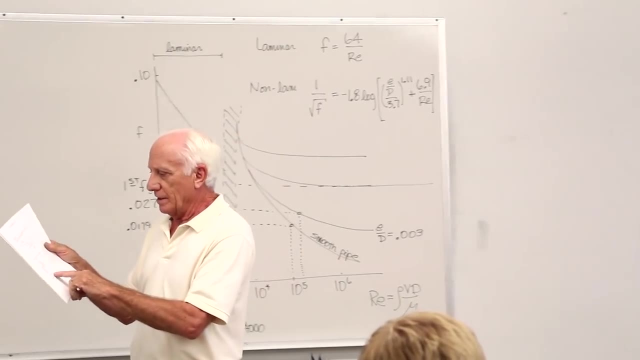 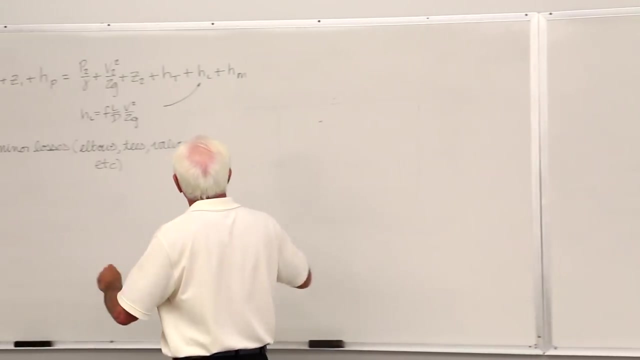 Okay, Okay, Okay, But so drop down the middle of the page. The middle of the page gives you a table which lists various type fittings in a pipe network, along with their K value. Now let's get the K value done. The minor losses are expressed as the summation. 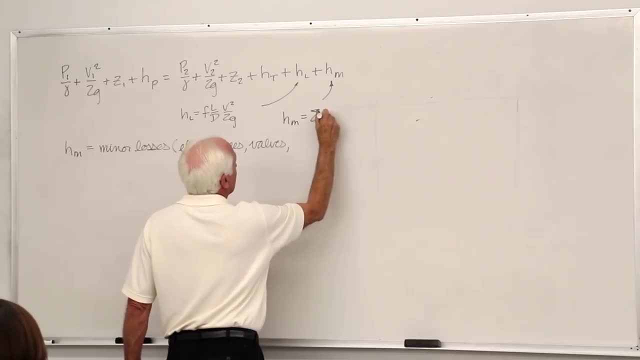 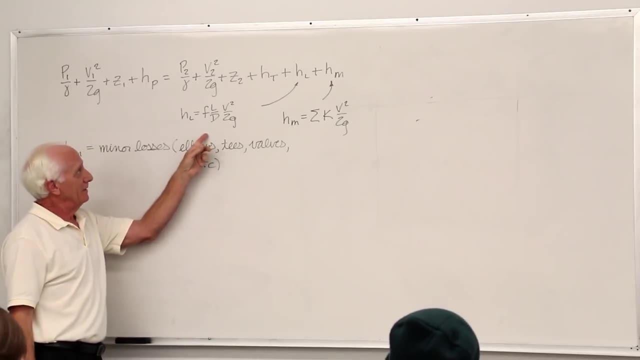 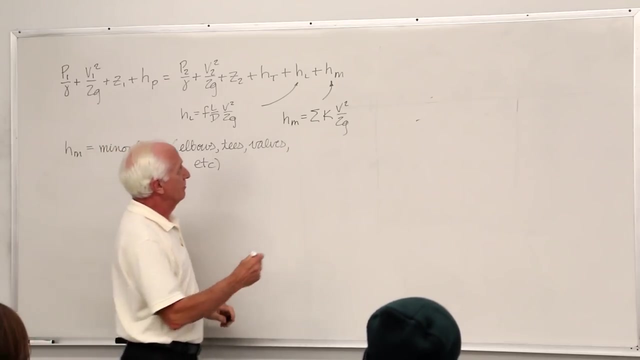 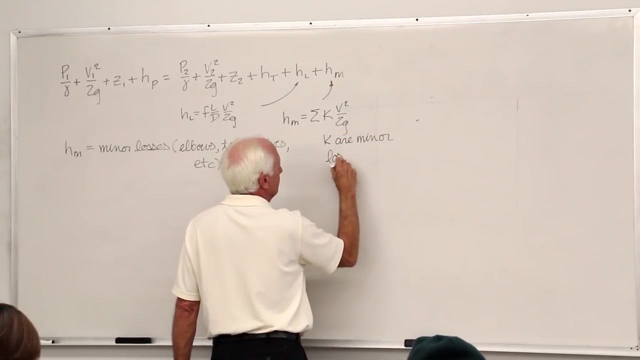 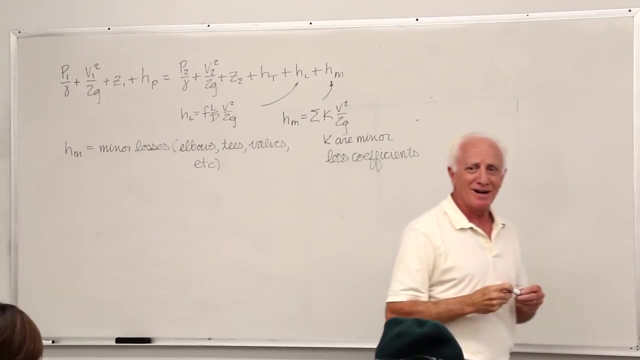 of K times V squared over 2G. It looks a lot like this guy, except in front of the V squared divided by 2G. we have a summation of Ks. The Ks are called the minor loss coefficients. They're pretty much constants. 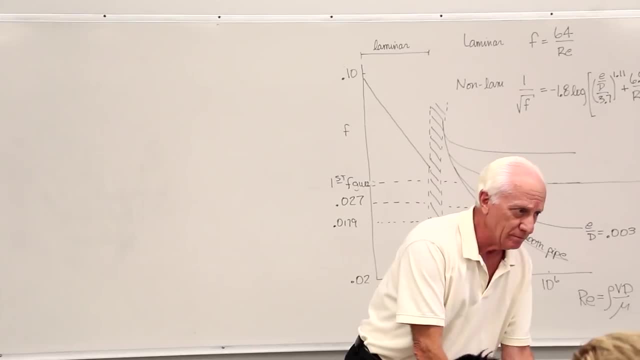 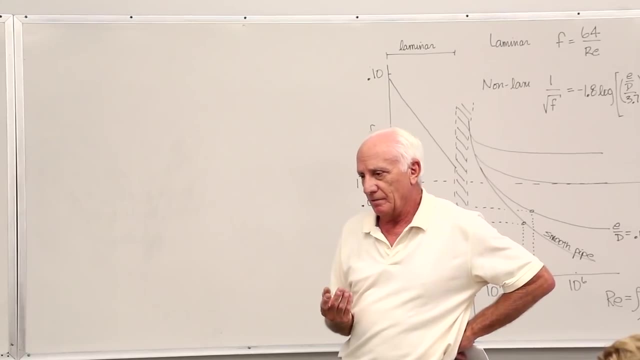 They're constants. You search them out and find them and add them together in the pipe network: From where to where, Typically from 0.1 to 0.2.. Wherever you write the energy equation, go from 0.1 to 0.2. 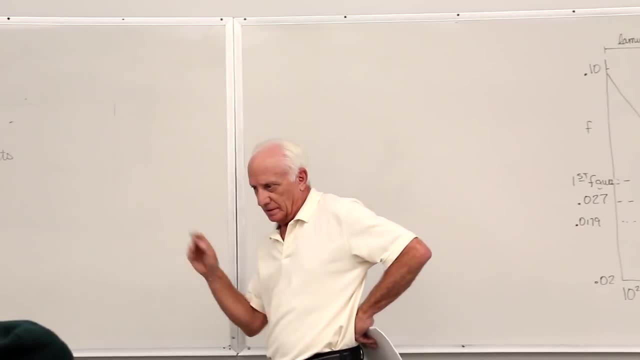 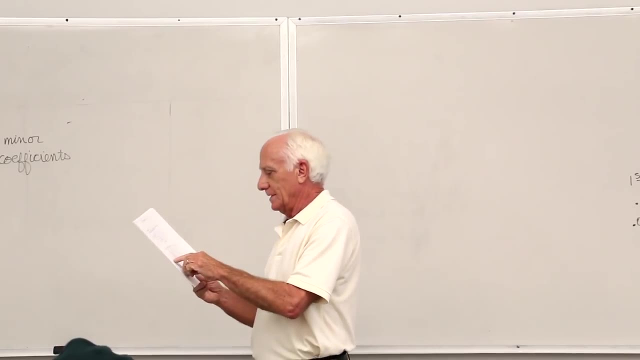 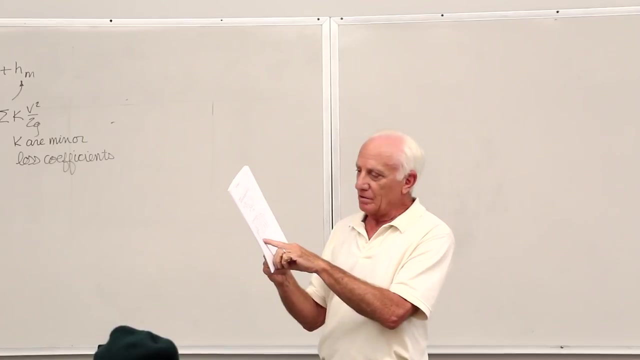 and find all the minor losses in that path. Okay, Well, here we are. Let's go down to an elbow. There's an elbow. There's a standard elbow, a long sweep elbow, a 45 degree elbow. then there are two kinds. of components. Under the connections: a screwed connection for a pipe or a flange connection for a pipe. Under the screwed connection, the diameter 2.5, 5, 10.. Under the flange, 5, 10, 20 centimeters. 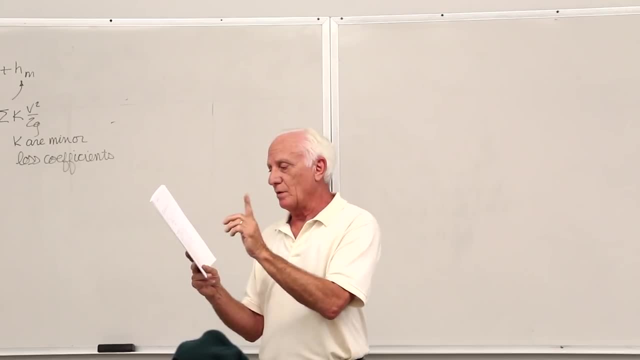 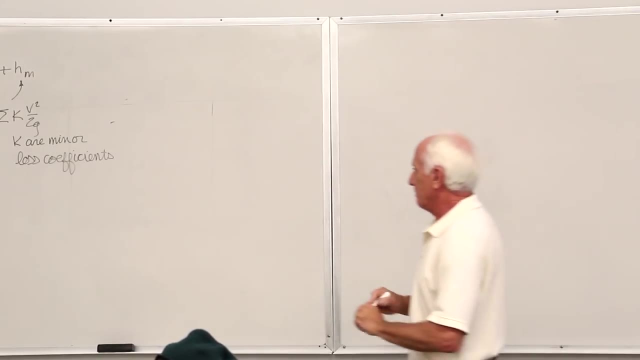 Then you have different kind of valves, By the way. there's a T, two Ts, a branch and a line, A branch and a line. Here comes a flow into a T. Here's a flow into a T. Here's a flow into a T. 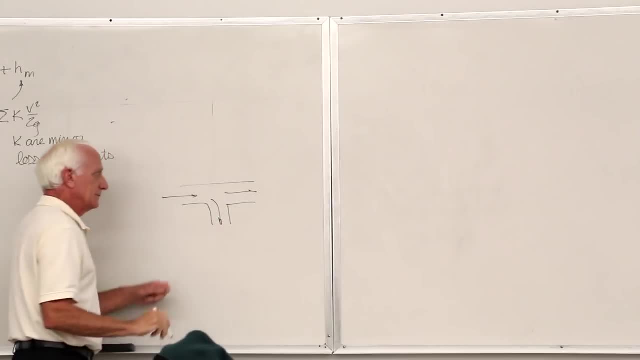 Some of it goes that way, some goes down that way. If the flow goes here to here, that's line, the main line. So railroad track, that's the main line. The branch railroad track makes your right turn, that guy. 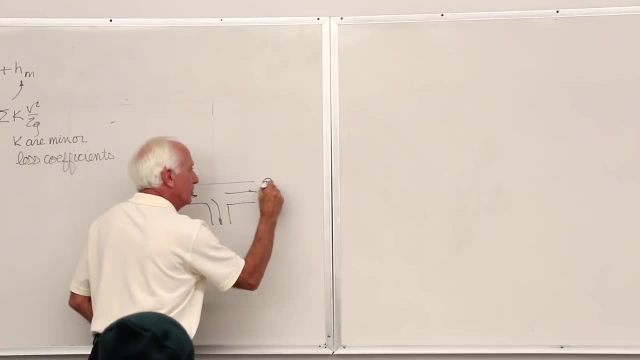 So if your point here is 1 and your point here is 2, you use the line value. If your point 1 is there and your point 2 is here, you use the branch value. Okay, Where do these things come from? 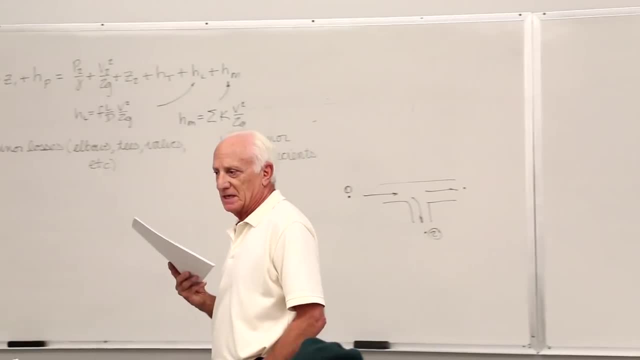 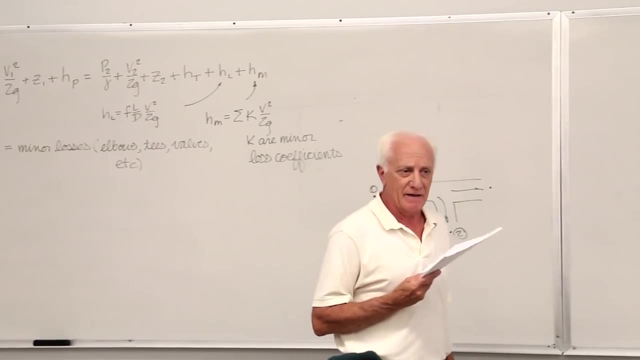 Oh, they came from experimentation. We've got a whole setup in the fluid mechanics hydraulics lab. You can go down there and put anything you want in our pipe network and find the K value. Matter of fact, that's one experiment. 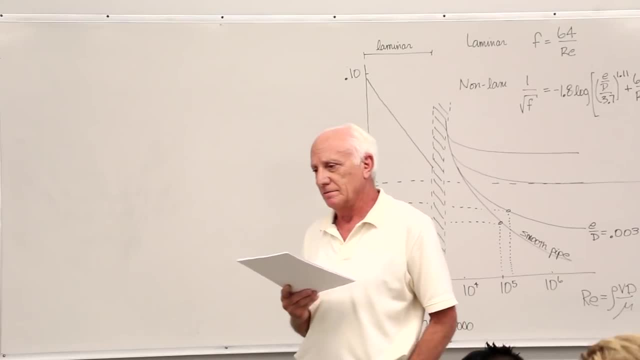 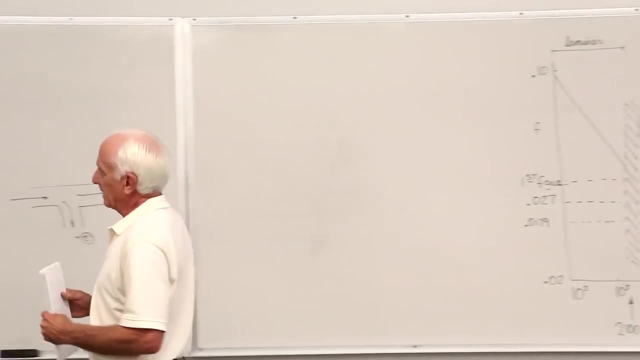 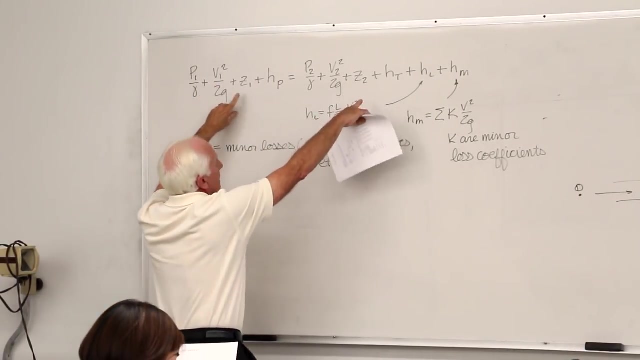 A globe valve, a gate valve, a swing check valve, a filter, all those things. you can find the K value. What do they do? Take a piece of horizontal pipe. Okay, These two guys cancel out. These two guys are zero. 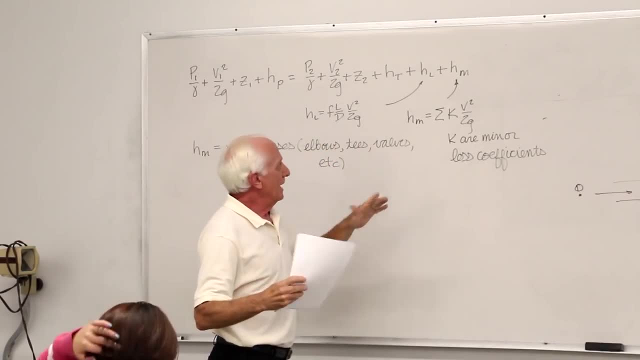 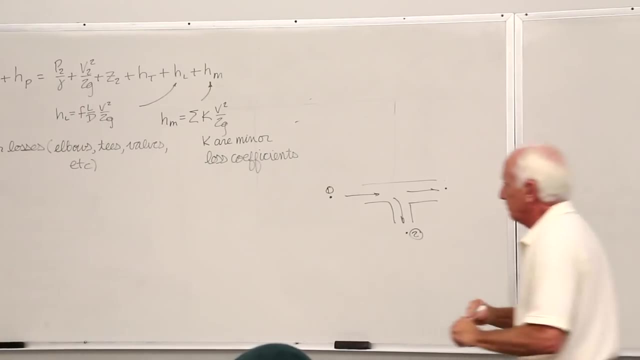 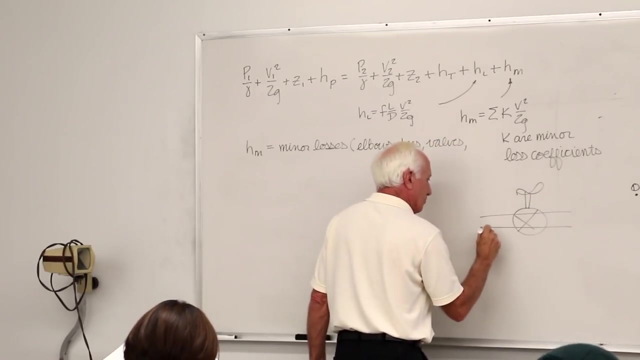 There's no pump, There's no turbine. Account for the short piece of pipe between your two pressure taps. So if this is your two pressure taps here, here's a valve. You put a pressure tap in here. pressure tap in here. 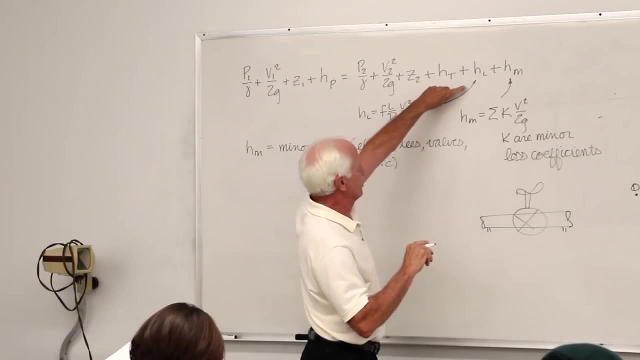 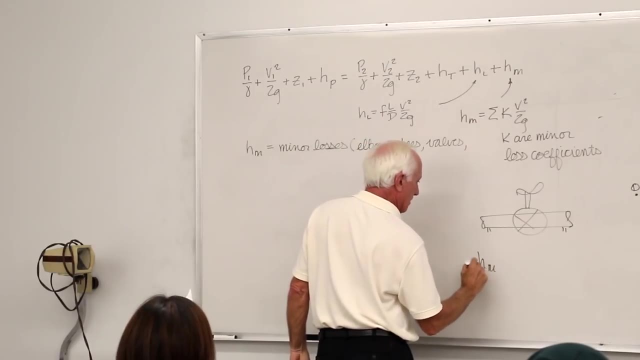 If the pressure taps are close to the valve then there's really no straight pipe. So he's gone. he's gone, These guys are gone. That says HM is equal to P1 minus P2 divided by gamma, and HM is equal to KV squared over 2G. 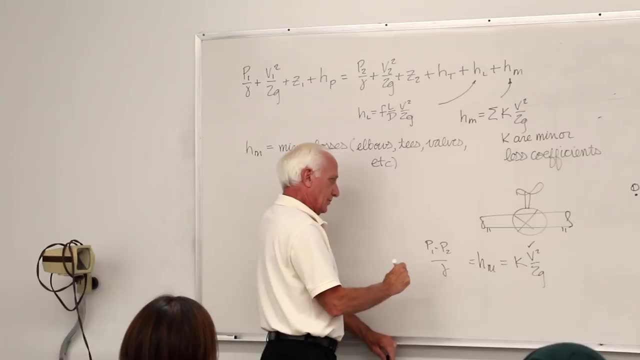 You measure the velocity with a flow meter? I've got it. You measure delta P with a pressure transducer- I got it. You know what's water at room temperature? I got it. What do you solve for K? K values in that table came from that method. 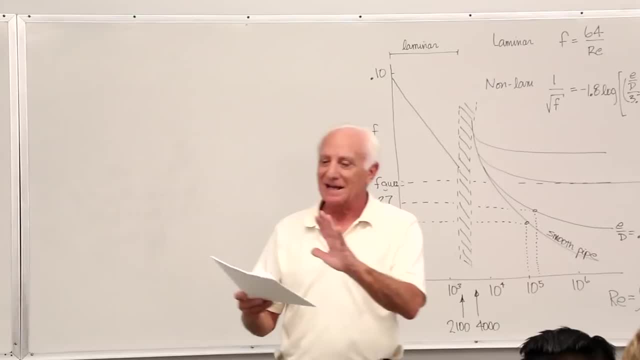 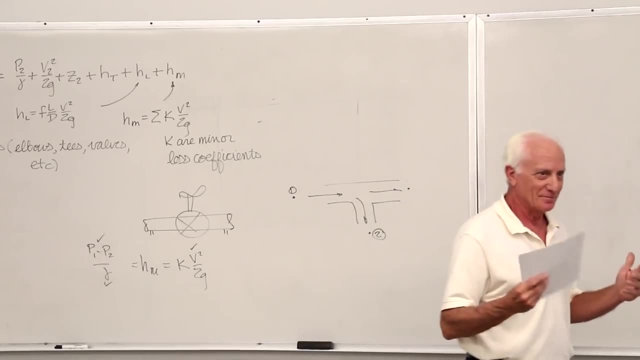 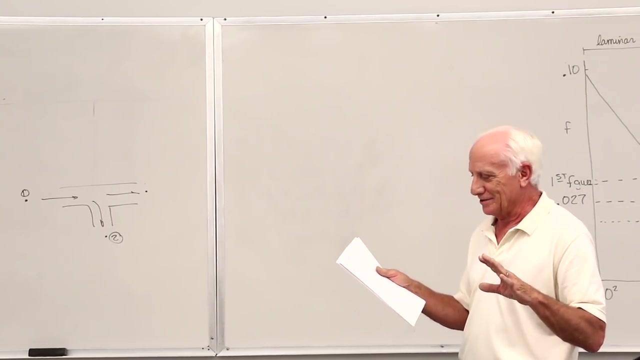 of experimentation, Okay. So anyway, they came from experiments. There They can vary dramatically, you know, plus or minus 30,, 40,, 50 percent, Because everybody makes things a little bit differently. Valve manufacturers. filter manufacturers. 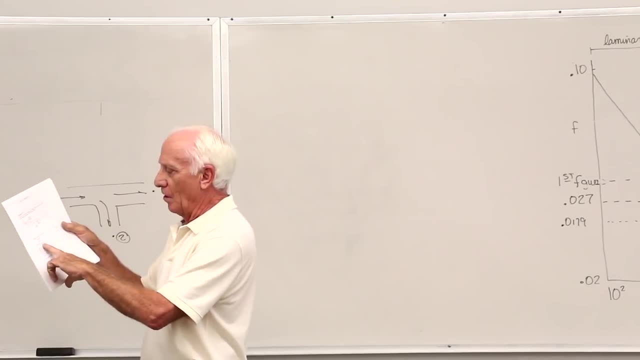 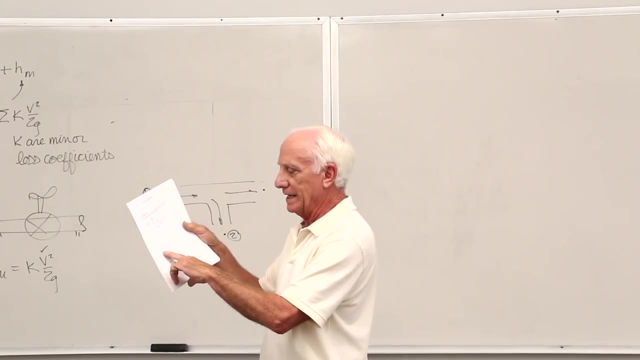 Anyway, back to here Globe valve. Is it fully open, Half open or one quarter open? An angle valve fully open, A swing check valve fully open, A gate valve fully open, A return bend where it makes a 180.. 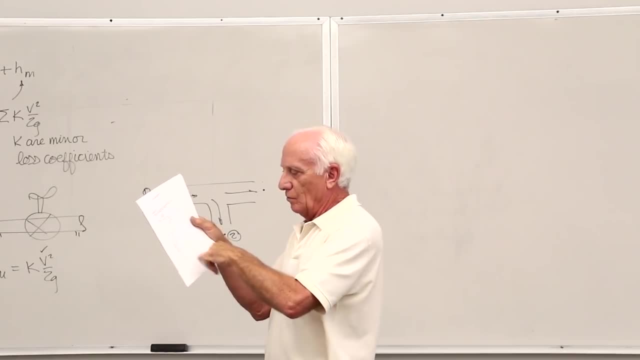 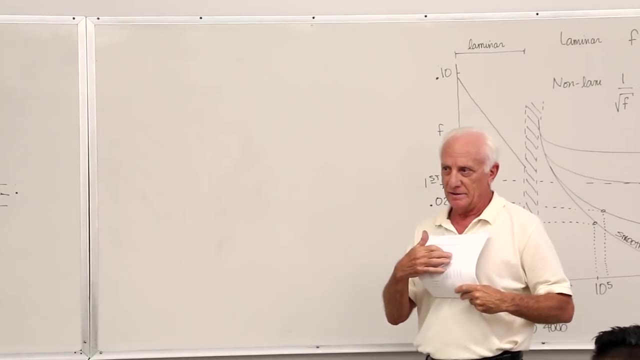 Return bend is in there. All those things are what? if you can't find it here, Well, go search it on the line on the internet. Go search it, you'll find it somewhere. Search it out. If it's not in here, you're the engineer. 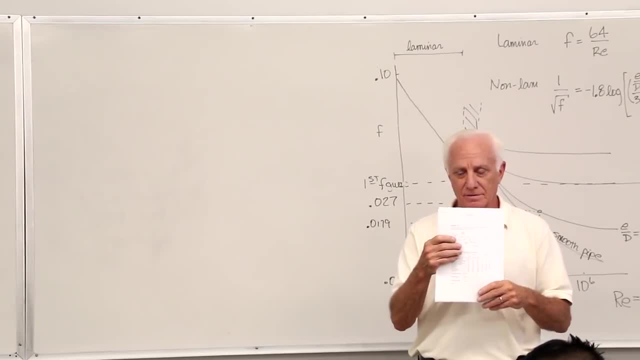 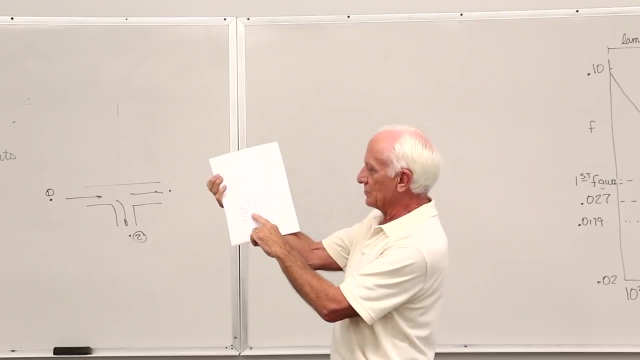 You go out and find what the K value is for. If you can't find out, you might draw a test on it and see what the K value is, But you'll probably find it. Oh, a square-edged entrance from a reservoir to a pipe: 0.5.. 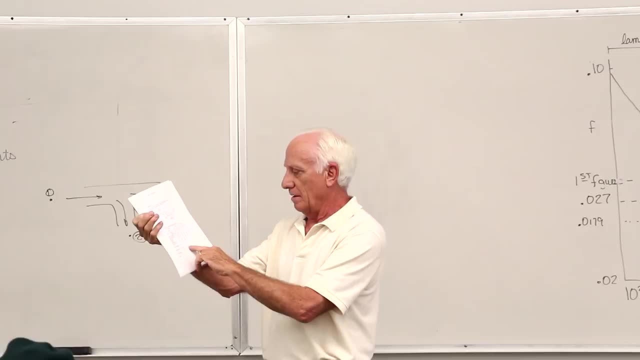 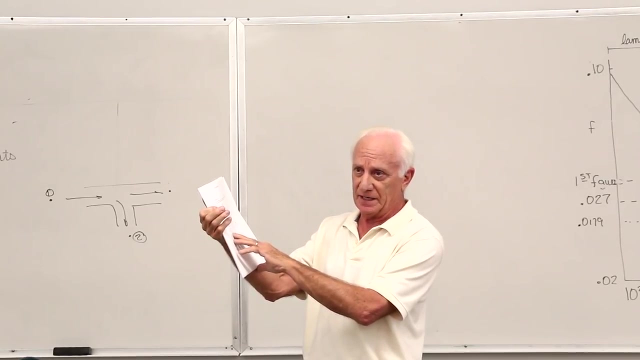 A reentrant entrance where the pipe sticks into the reservoir: 0.8.. A well-rounded entrance, very smooth. K 0.03, really low. Look at the K for a globe valve: one quarter open. Wow, 50, 50.. 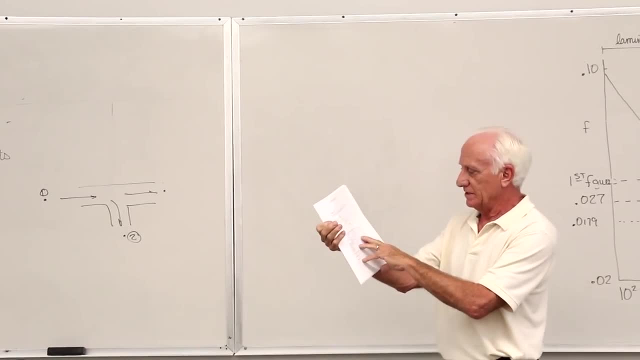 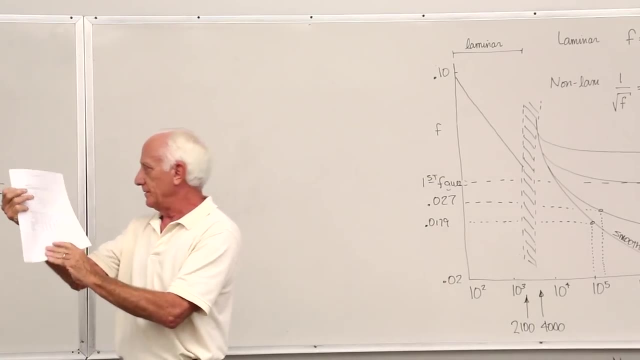 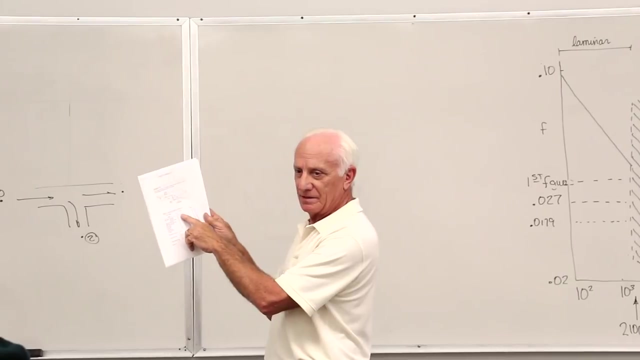 Big time Pressure drop. okay, 60 for a flange one, 60. Okay, all these things are here. okay, What if your diameter is, by the way, it says screw 5 inches. that's a misprint, that's centimeters. 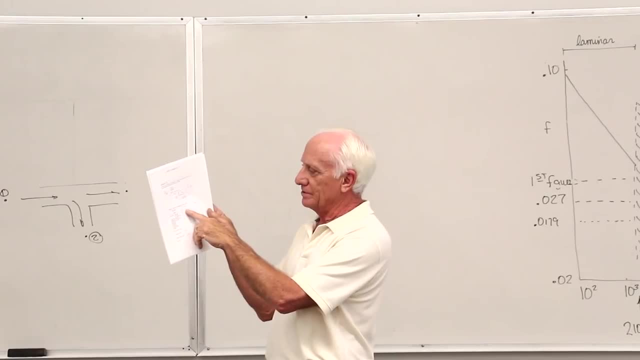 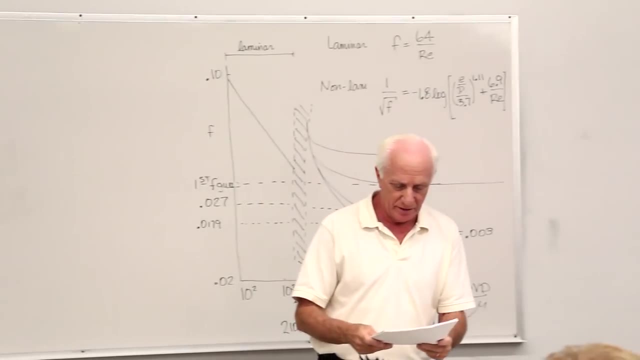 So I'm going to change that to centimeters Under screw connections. 5 inch should be 5 centimeters. What if you've got something that's 7.5 centimeters And you say, well, it's not on there? 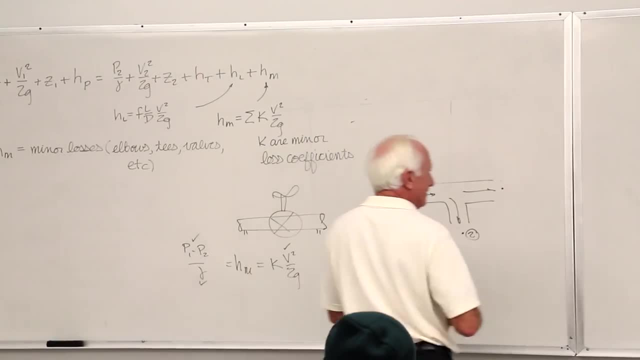 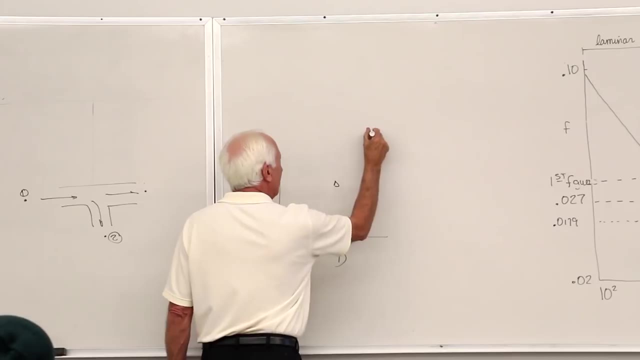 What you do is you plot K versus diameter. There's three values given there here, here and there. Take your best guess on Excel, Draw a line through it. There you go. Now find 7.5.. Don't interpolate literally unless you know it's linear. 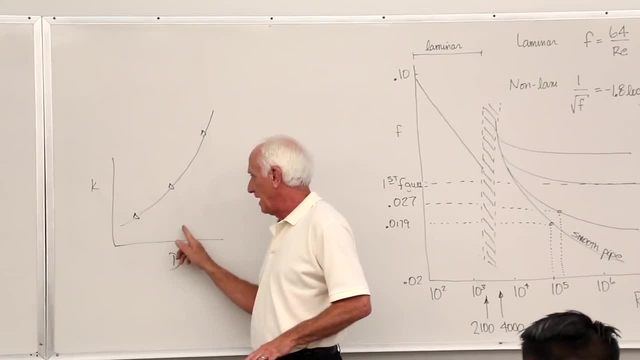 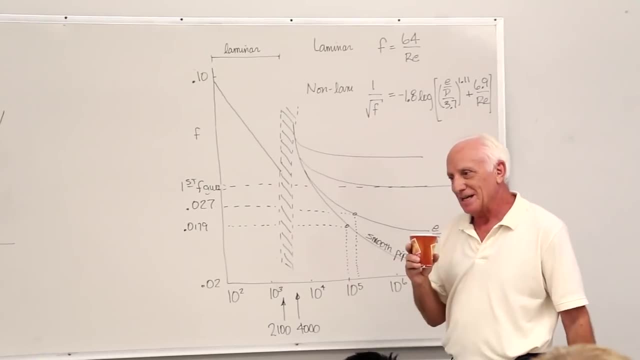 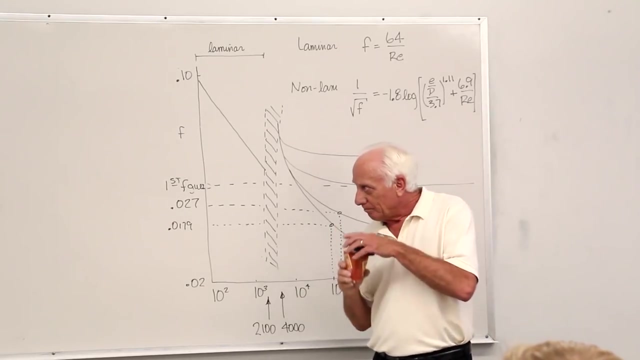 No, no, no. Plot the values and then go to the dime you have and read it carefully, Because you'll find out they're not linear. They're not linear. Okay, so that's how you find the K values for different diameters on that sheet of paper. 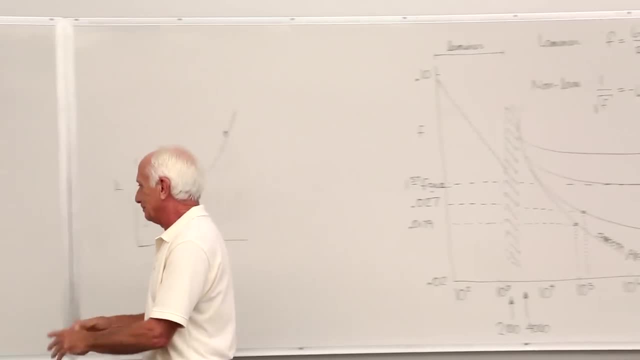 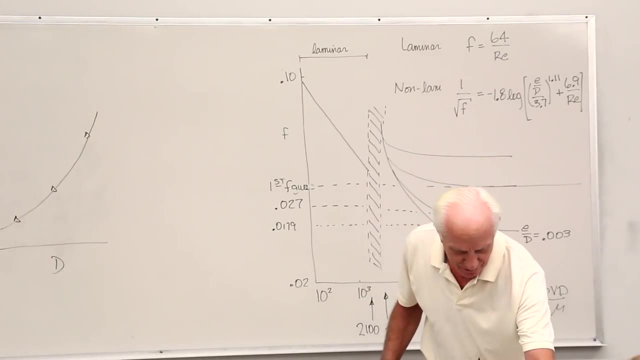 Okay, so that's what we do with that. Now let's take a look at the example problem I've got there, which is the one that's above it, So you can- this is just so I don't have to write this on the board and have you copy it down. 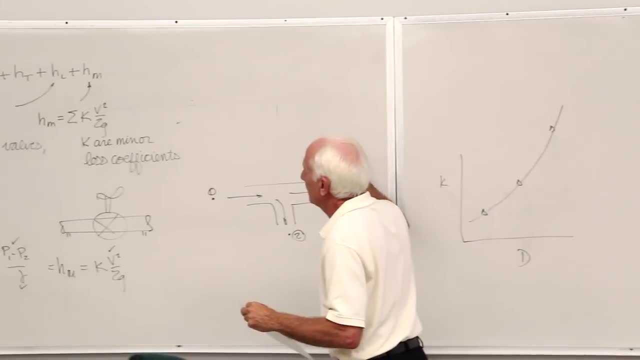 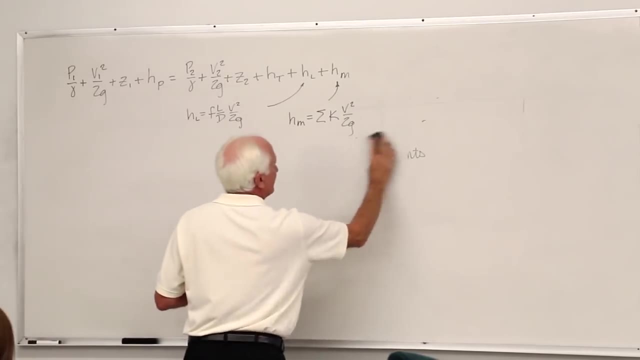 But I'll put a little more of it. You don't need to copy it down. Let's leave that equation up there. Okay, let's get rid of this, Let's get rid of this, And I'll draw the picture of it just so that we can follow. 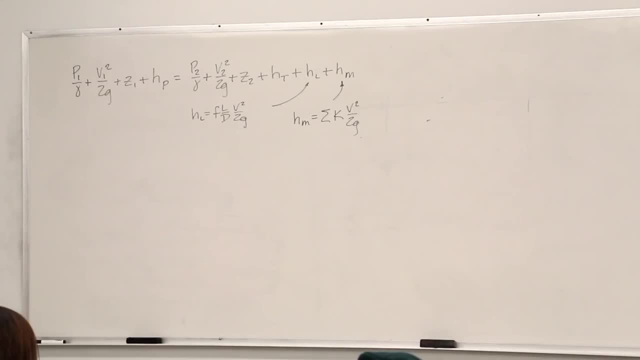 on the board We have two reservoirs with water at 20 degrees C. Okay, so reservoir one is up here, Water at 20 degrees C, So this is going into a pipeline because this makes an elbow down here. elbow here ends up down here. 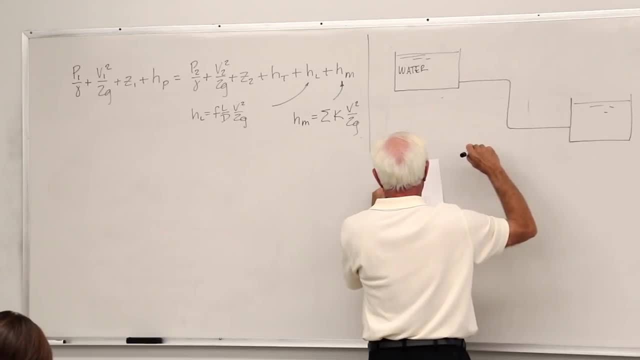 This is H Capital H. Okay, there is a screwed blow valve fully open right here. I'm not going to put all the details on it. it's fully open 20 meters from here to here, 10 meters from here to here. 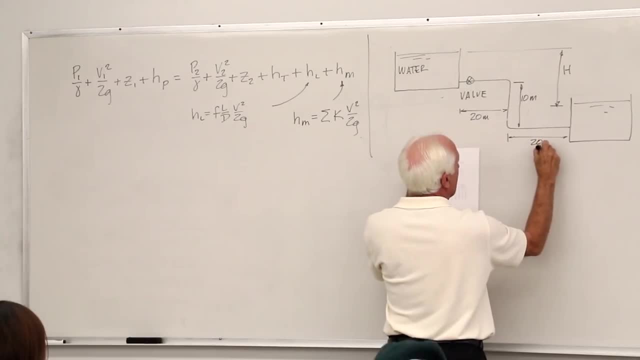 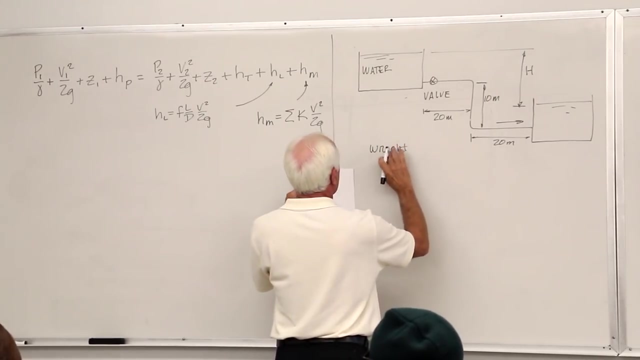 and 20 meters from here to here. Of course, the water is going to be flat. It's going to be flowing down from the upper reservoir to the lower reservoir, so the flow direction is like that. The pipe is wrought iron. It has a diameter of 10 centimeters. 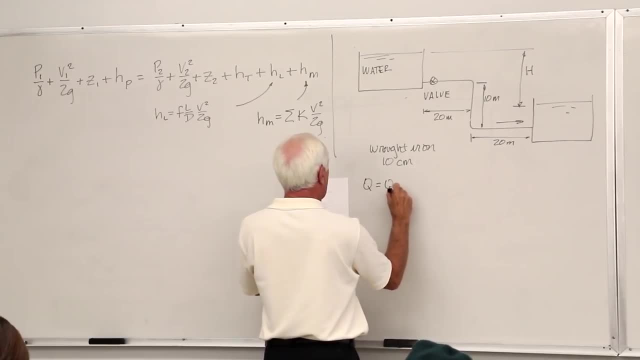 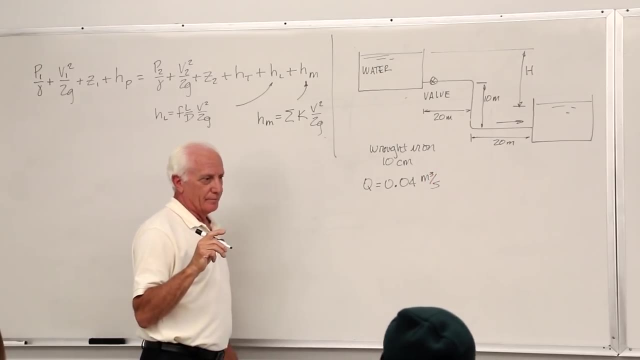 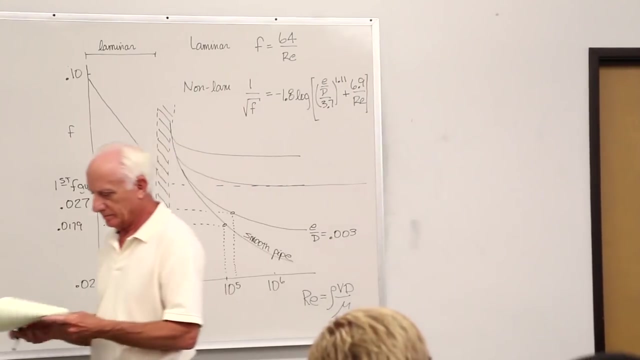 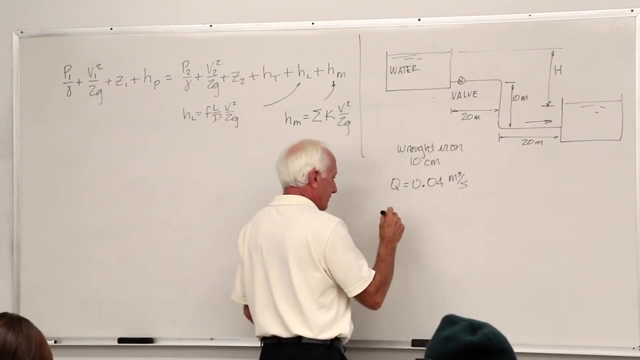 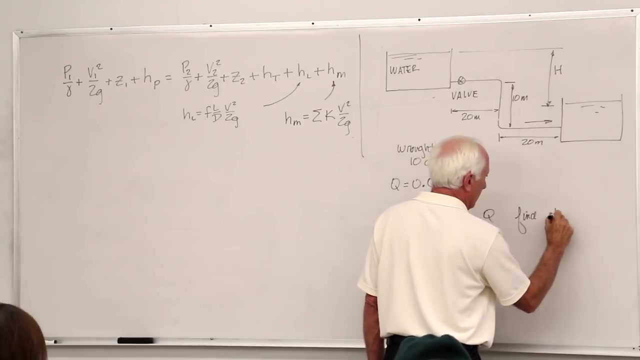 The flow rate Q is equal to 0.04.. Okay, Okay, Okay, Oh, and let's see, Yeah, find H, Okay, so we're supposed to then find H, Given, Given, Given, E, D, L, Q, Find H. 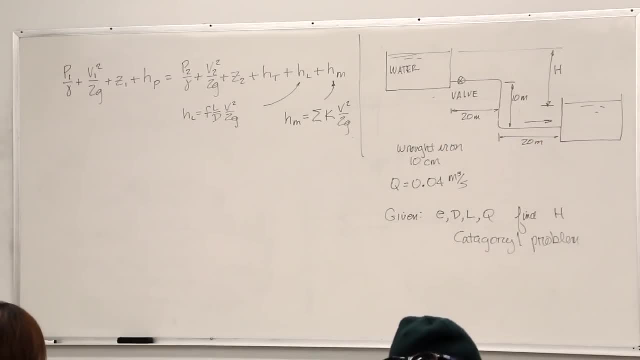 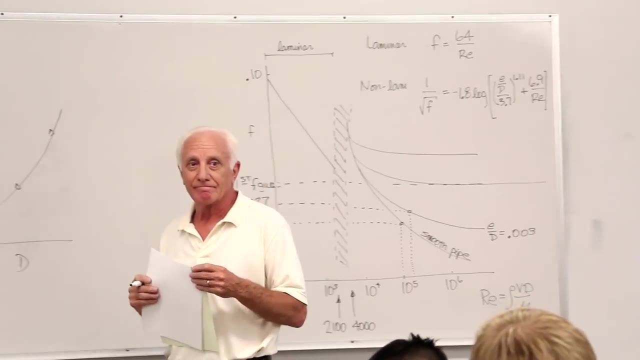 Okay, I know I'm running away. That's a Category 1 problem. I don't need to iterate. I don't need to iterate. I don't need to iterate. What's E again? What will we? I'm sorry. 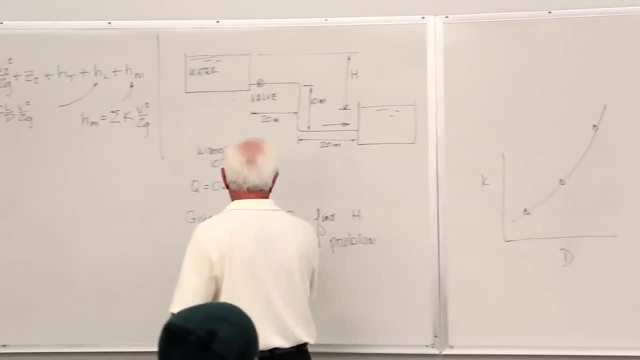 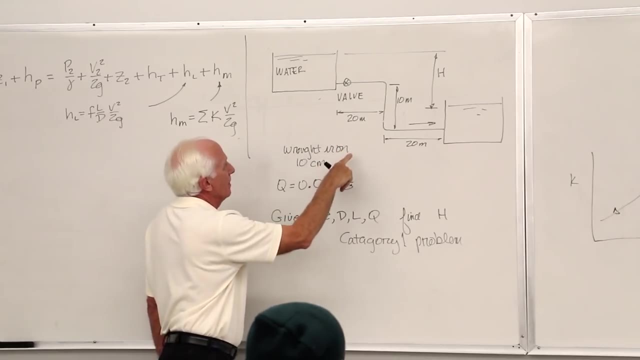 What's E? again? This one, Yeah, That That Wrought iron. tells me that's that All right. That tells me that. That tells me that. That tells me that. So when somebody says I'm giving you the pipe machine. 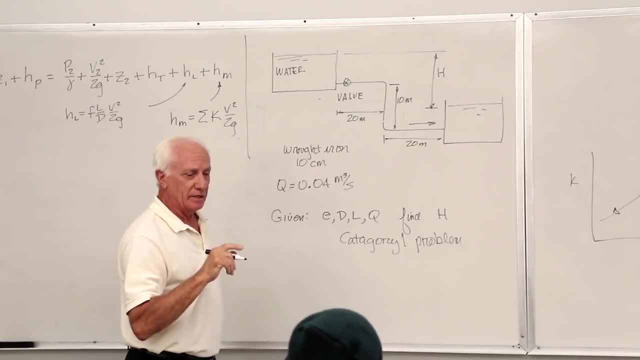 I'm going to tell you what's going to happen. Okay, Okay, you, the pipe material, you know, they're saying I'm giving you E. If somebody says to you I'm giving you the volumetric flow rate with the pipe diner, they're telling you I'm giving. 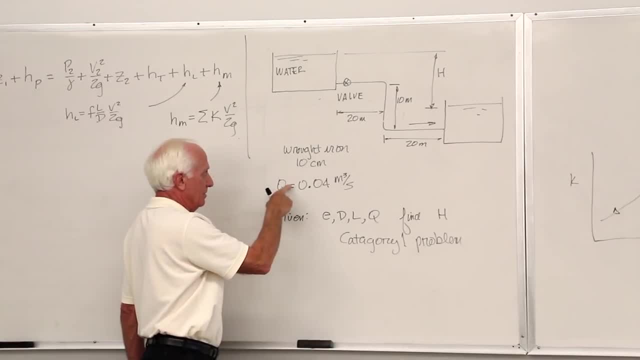 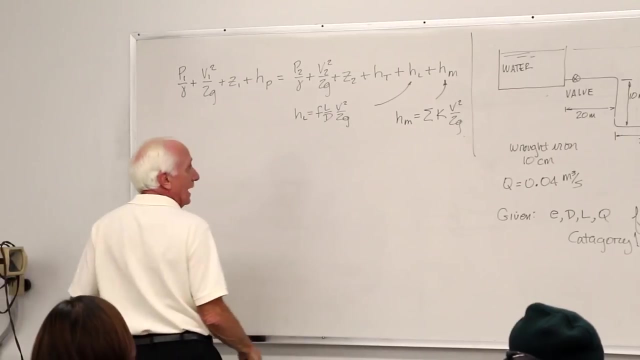 you velocity B? Do I have Q? Yes. Do I have diner? Yes. Can I find B? Of course. Okay. Now let's go back to here again. I'm of course don't put 0.1 down there, No, no. 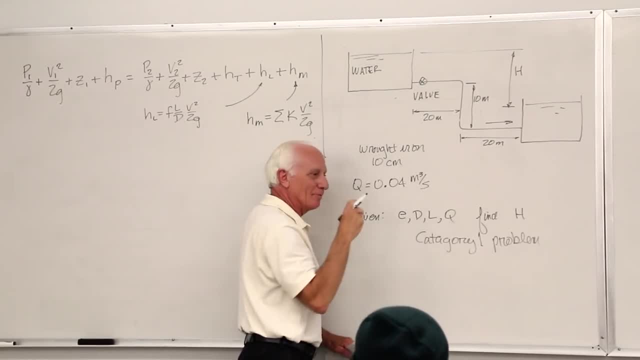 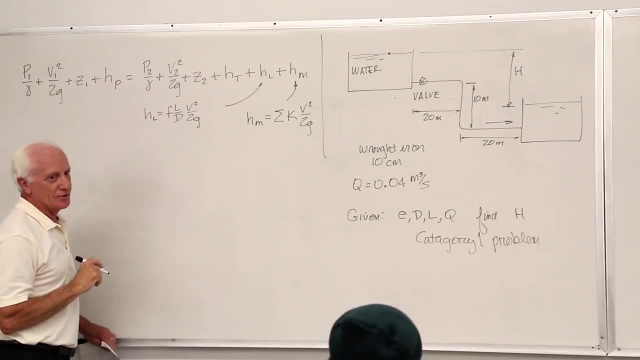 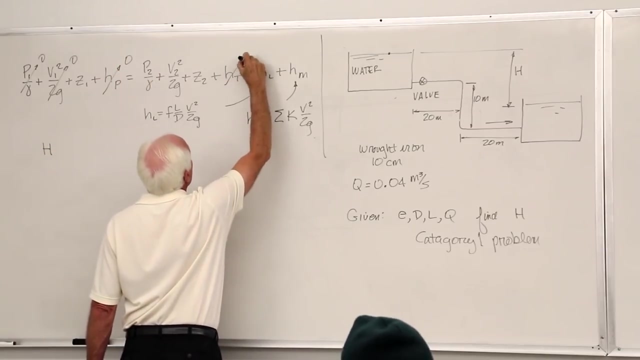 bad choice. bad choice. Put 0.1 where you know the most stuff. The pressure is zero, The velocity is zero And the elevation is capital H- Okay, Zero, Zero. Capital H H- Okay. Is there a pump? No Zero. Is there a turbine? No Zero. Is P2 zero- Oh, by the way, 0.2. 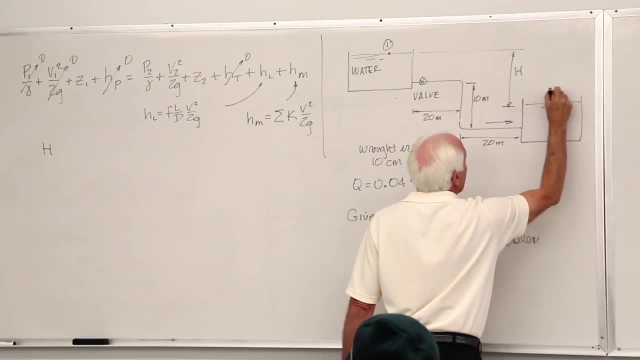 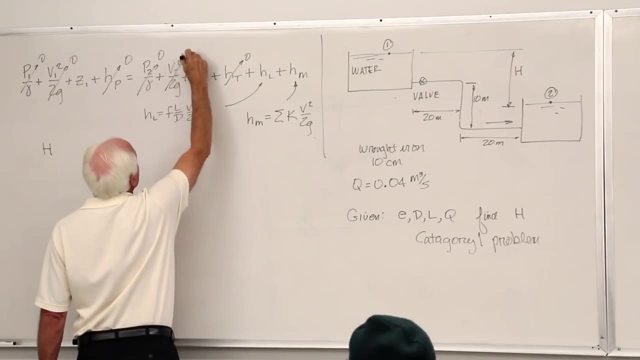 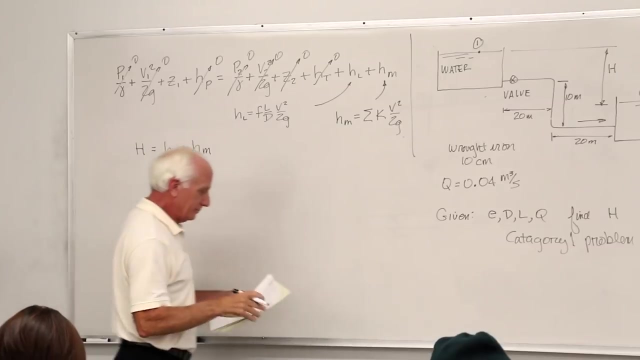 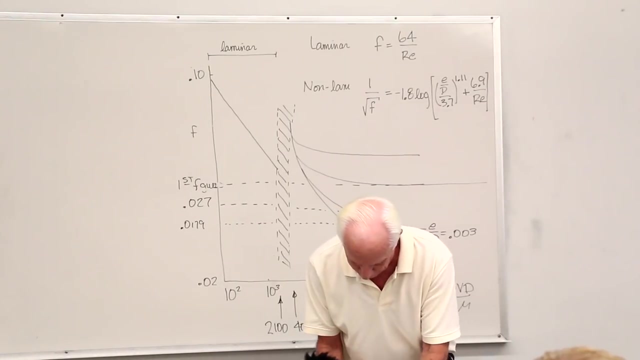 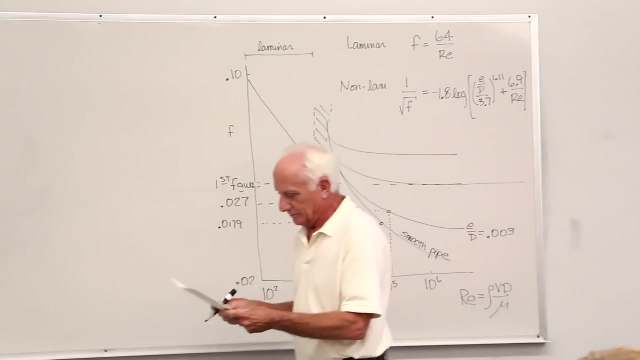 is over there. Where's it going to end up? Zero Is B2, zero, Yeah, Is Z2 zero? Yeah, Okay, So our H is equal to there's H, right there, H, H, H is equal to HL plus HM. Okay, So now let's see. Oh, there, we are All right, Let's. 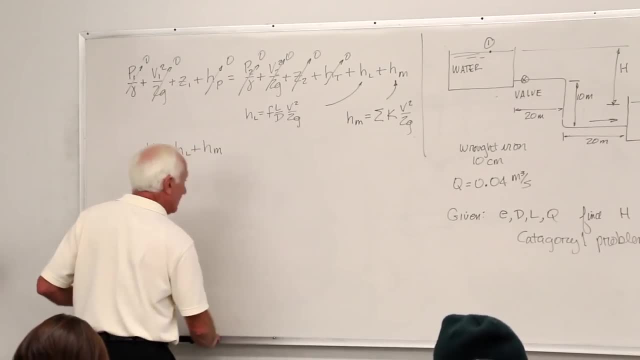 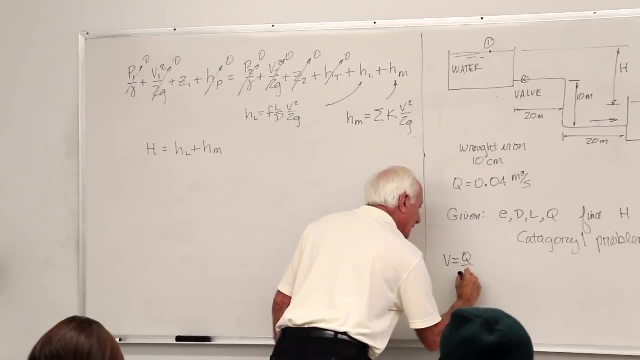 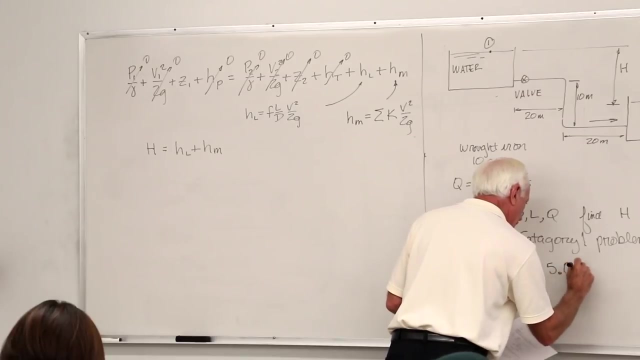 get the velocity. All right, I'll put that right here. Velocity equal Q over A, 0.04, divided by pi over 4.. Diameter is 10 centimeters, Pipe velocity: 5.09.. You see, there's three velocities in the energy equation. 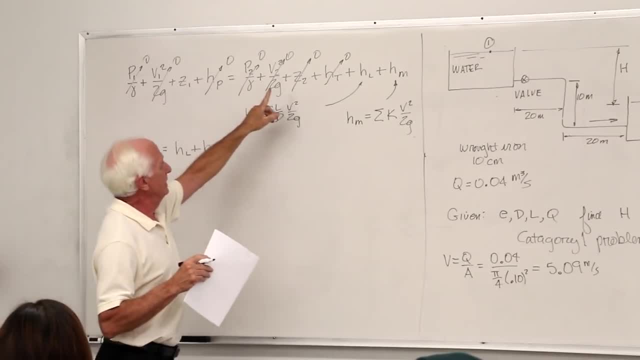 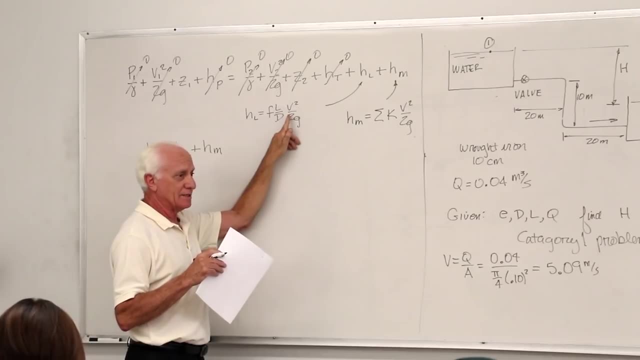 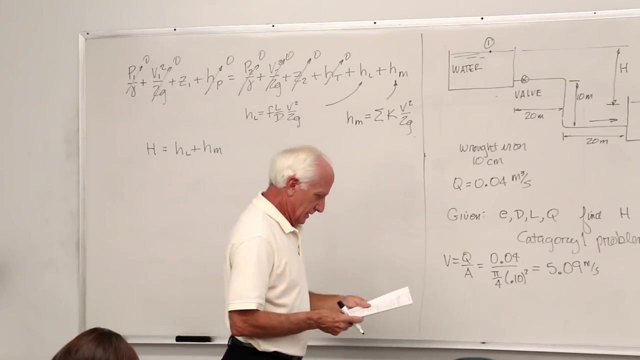 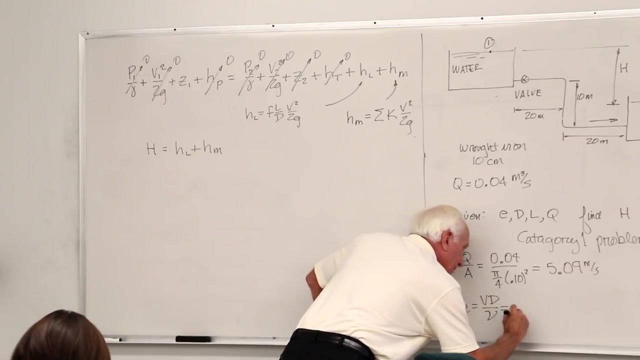 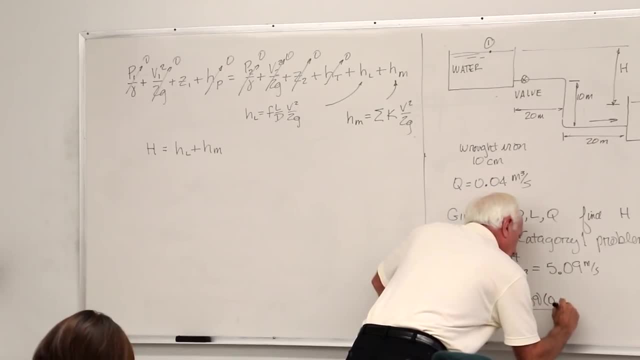 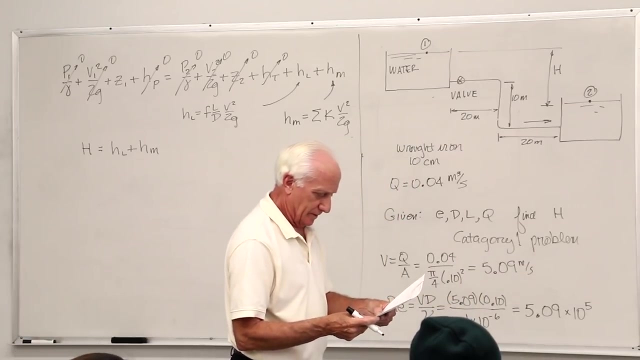 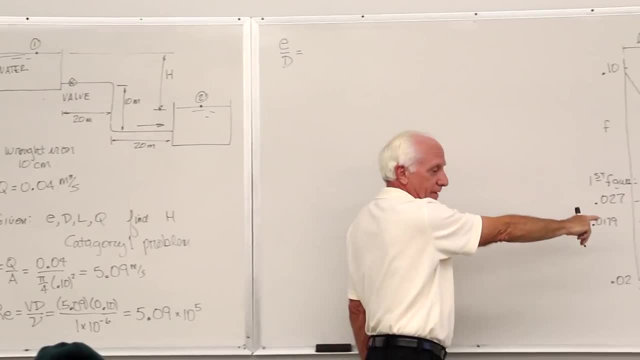 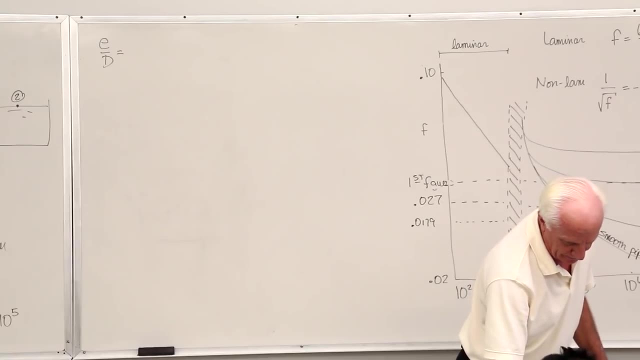 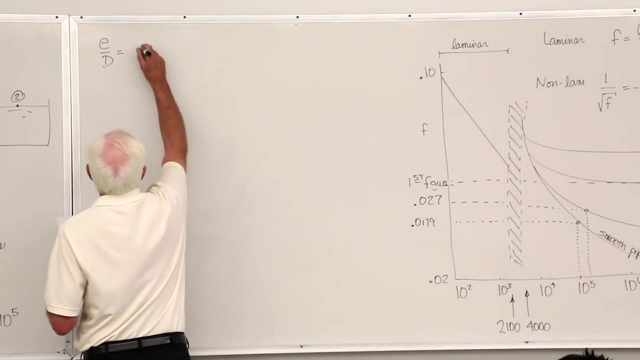 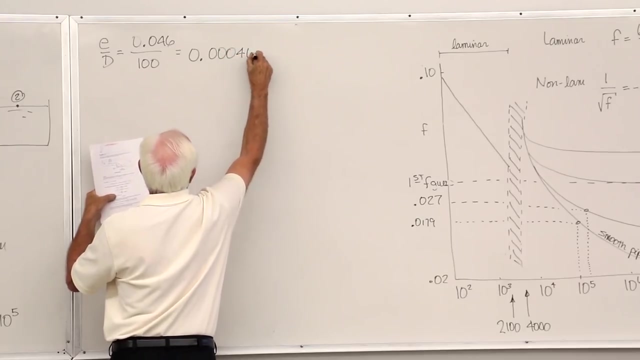 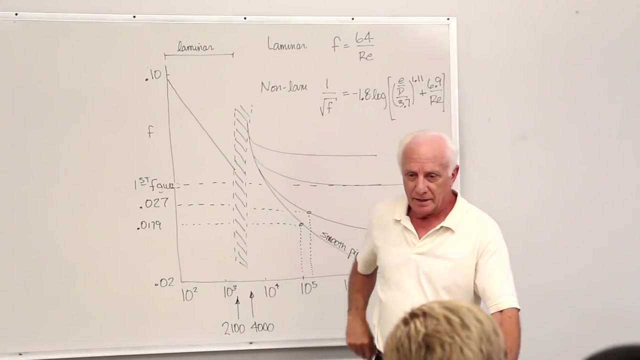 E over D. go to the little menu on the movie chart and find for galvanized wrought iron. okay, Find wrought iron There it is. So 0.046 divided by the pipe diameter equals 0.000 0.046.. Now of course you know if I go out and buy a steel pipe and I buy a 1-inch. steel pipe. is that 1-inch the inside diameter of the pipe? No, I scheduled it for you, by the way. Is the 1-inch the outside diameter of the pipe? No, Conclusion: a 1-inch pipe doesn't have an ID of 1-inch and doesn't have an OD of 1-inch. 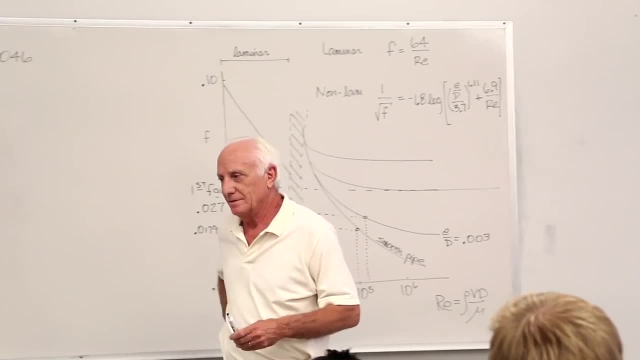 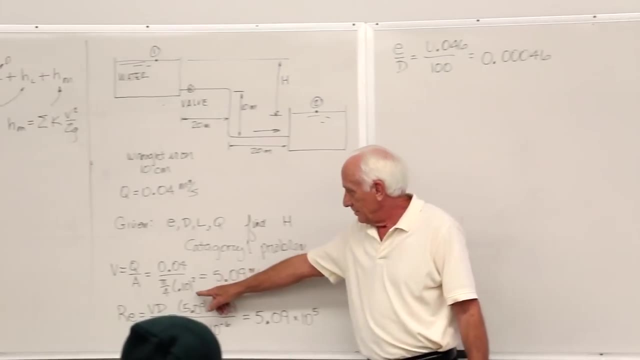 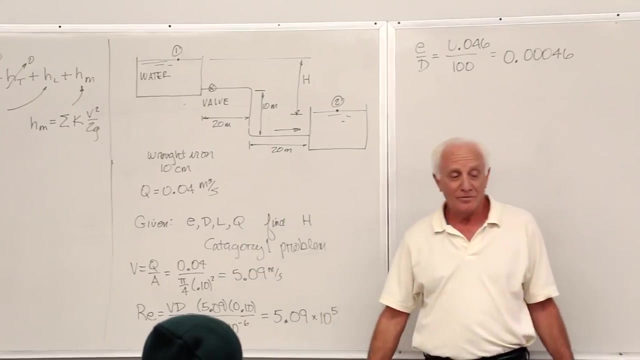 That's why it's called a nominal pipe size: Nominal. If you want to know the actual ID- and this Q should be based on, of course, the cross-sectional area where the water flows. That's the ID- You have to go to a pipe table and a pipe table tells you for a scheduled. 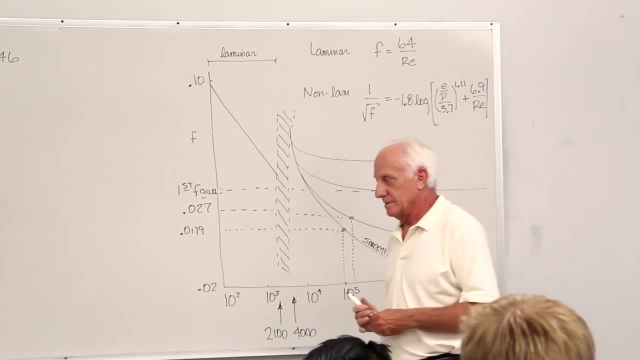 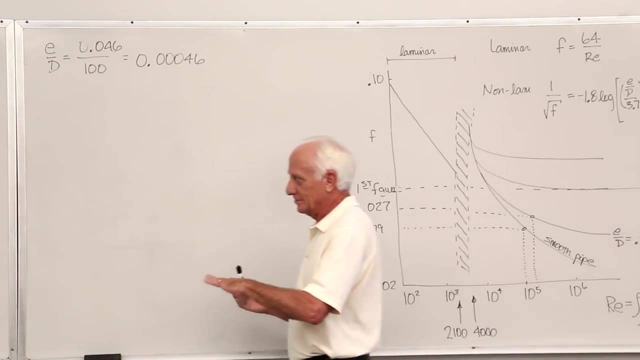 41-inch pipe. here's the ID, here's the OD. But in this class we're not going to worry about that. That's just a side light, just so you know when somebody says a 1-inch pipe is the inside diameter of the pipe, Be careful, Don't use 1-inch unless you know the ID is. 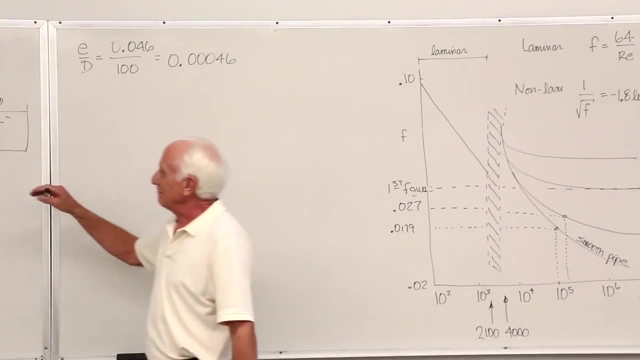 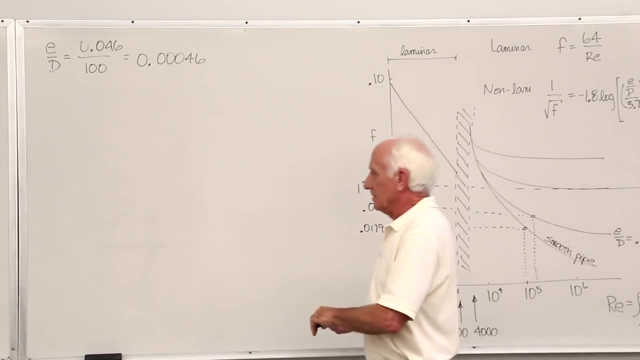 1-inch. Okay, In this class, though, if I say that's the pipe diameter, that's the inside diameter, Everything I say will be the inside diameter of the pipe. Okay, Go to the Moody chart with the Reynolds number: 5.1 times 10 to the fifth right here. Go up to the. 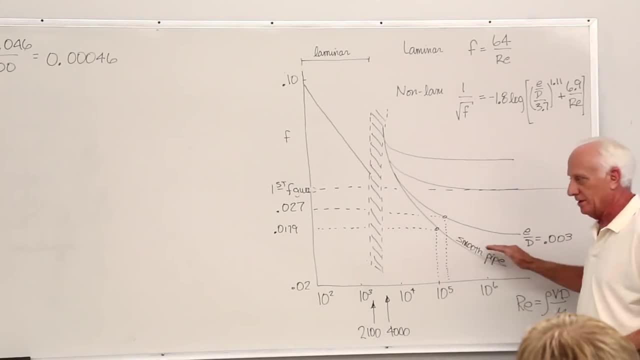 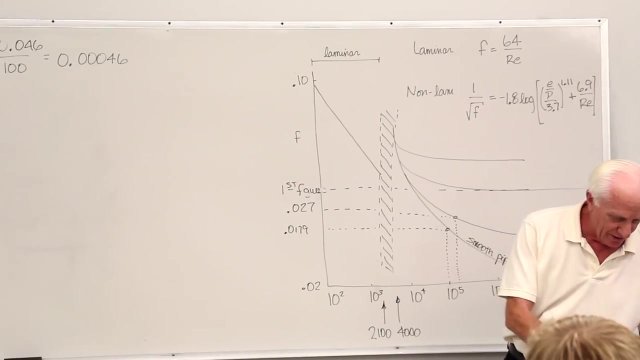 right line for E over D. legal point three. zero is four, six. It's down here somewhere. Go across Horizontally, always go across horizontally once you find the intersection. Go across horizontally until you find the friction factor And from the Moody chart it's 0.017. 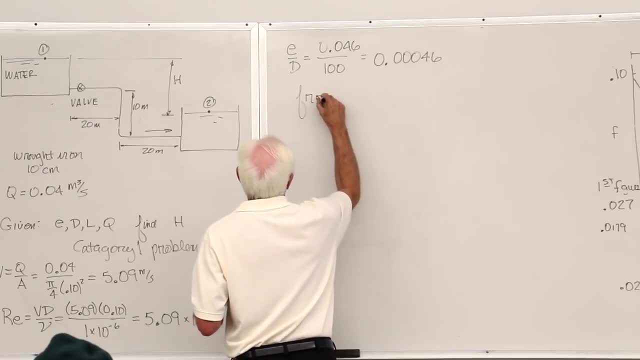 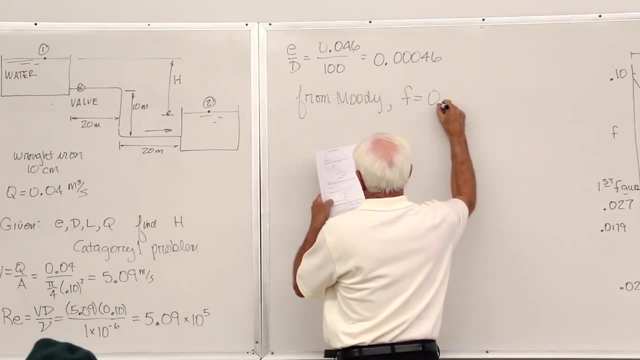 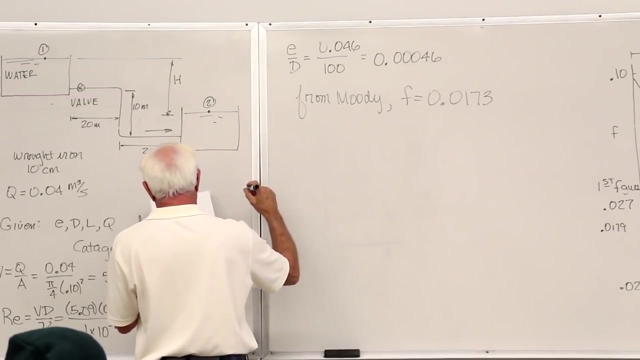 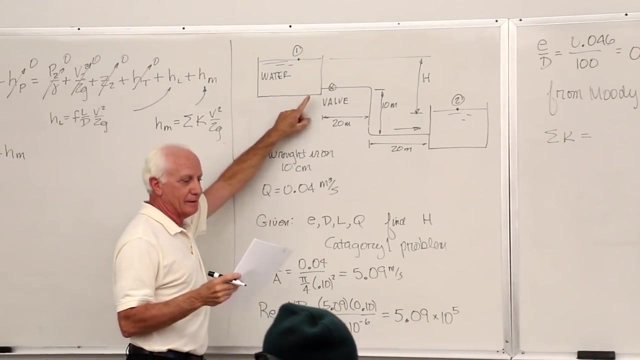 to an exaggerated three. Okay, Now we get. Let's look at the minor losses. Summation of the Ks. All right, So first of all, the water comes out of the upper reservoir. It goes into a pipe. Okay, Look at the minor. 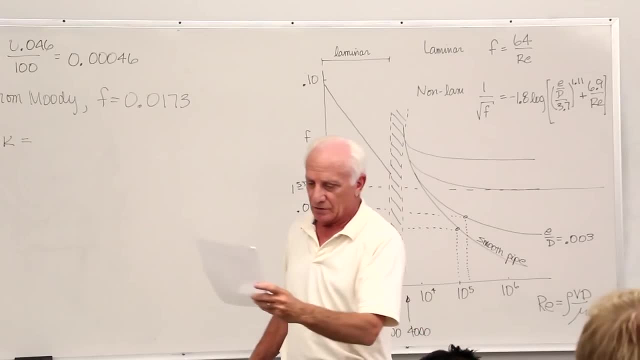 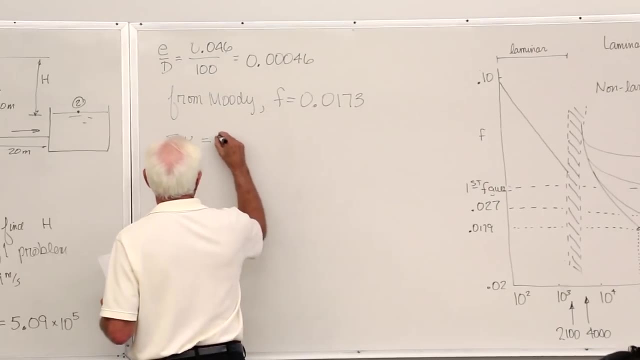 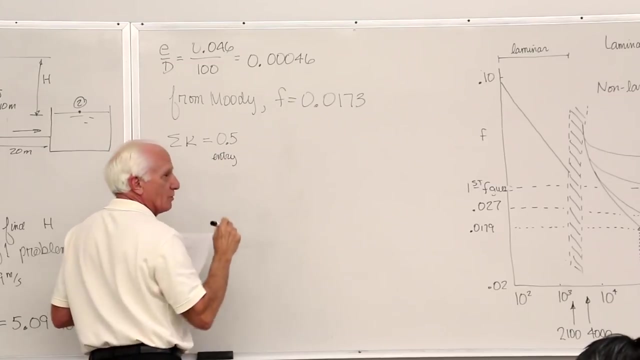 loss table. A square-edged entrance for a reservoir to a pipe. K is 0.5.. Okay, All right, Let's look at the minor losses. Summation of the Ks Entry. We're going to assume square-edged, unless told otherwise. You could make it like. 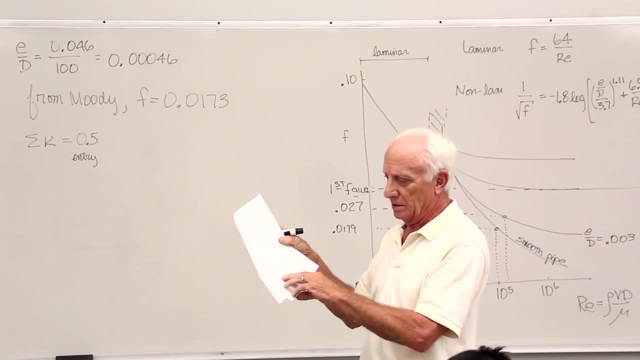 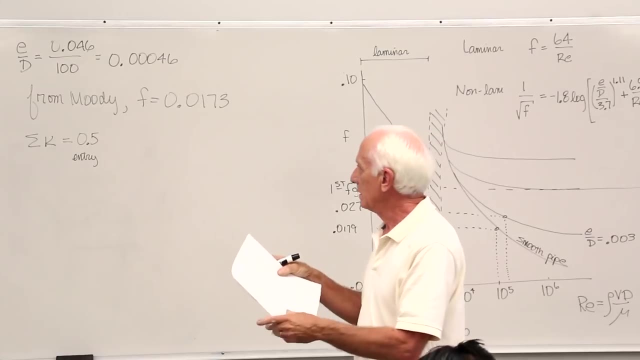 a well-rounded one, but that's expensive, not normally done. So unless it says well-rounded, assume it's always a square-edged inlet- 0.5.. By the way, the water comes out of the pipe and goes into the reservoir here. Exit. 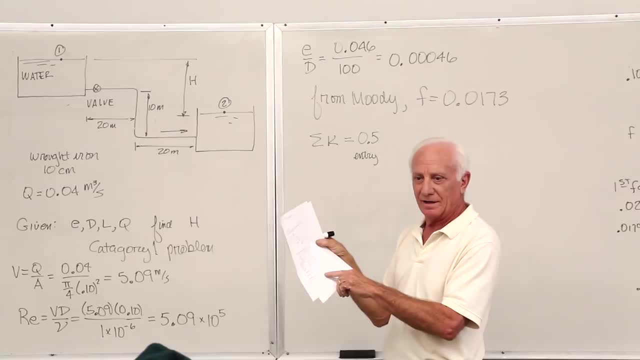 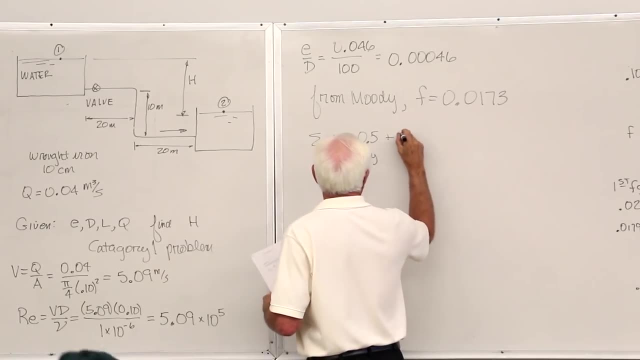 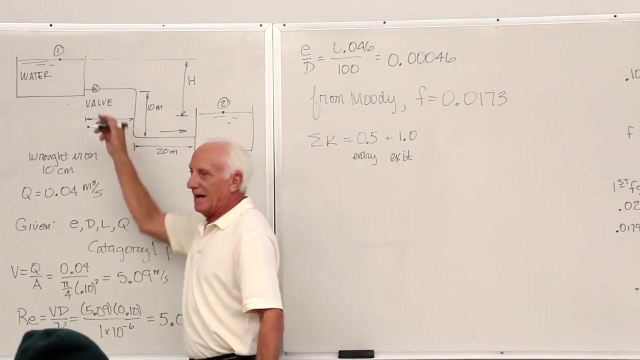 Okay, Pipe exit 1.. It doesn't matter if it's square as you're rounded, It's 1. Plus 1.. Now we go through a valve. What kind of a valve? told us That the valve was a screw. 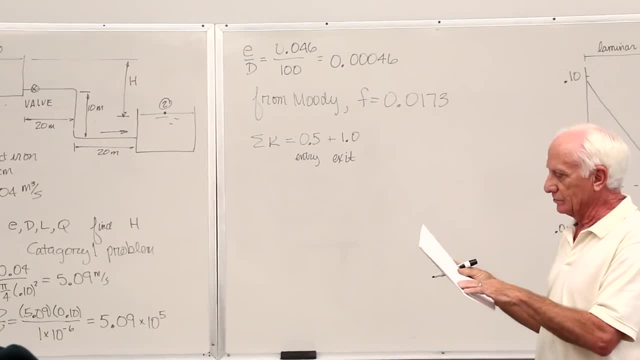 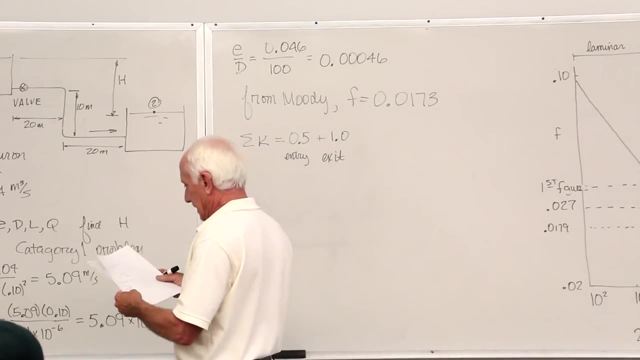 blow valve. So go to our page: Blow valve- Screw blow valve- Wide open, Okay, Wide open, Okay. The pipe diameter was 10 centimeters, So the blow valve fully opened- 5.7, I guess it was. 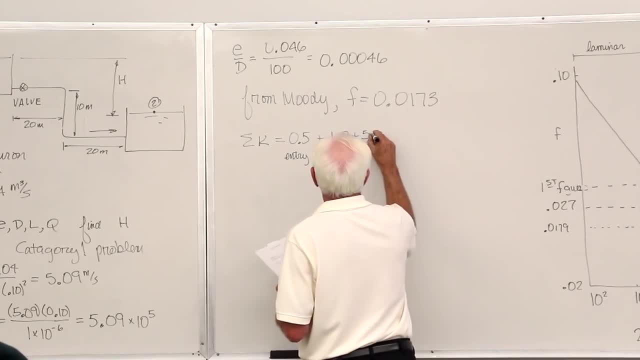 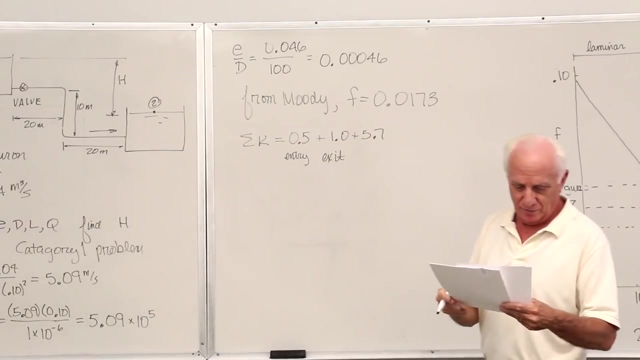 Okay, Yeah, it's a screw like 5.7.. Fully open blow valve, All right. And now we've got two elbows here and here. Unless you're told otherwise, always assume they're square-edged. Okay, They're standard elbows. Always assume standard unless you're told otherwise, So standard. 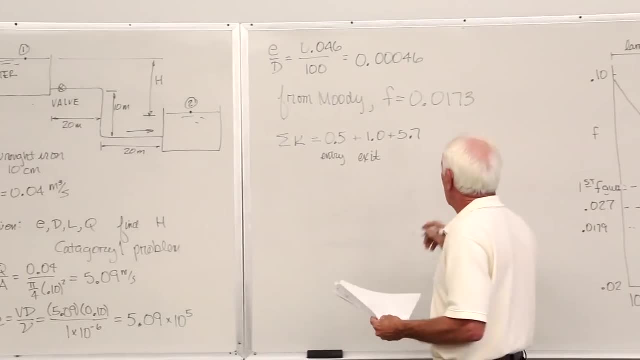 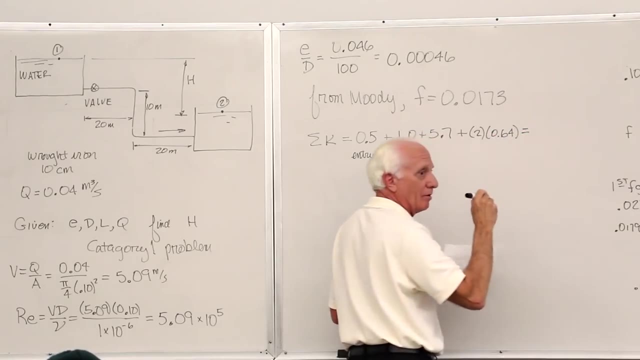 elbows: 0.64 plus 2 times 0.64.. So the summation of all the minor losses in that pipe network come out to be: let's see, Okay, That's 1,, 2,, 8, and 5.7.. And we're going to go through. 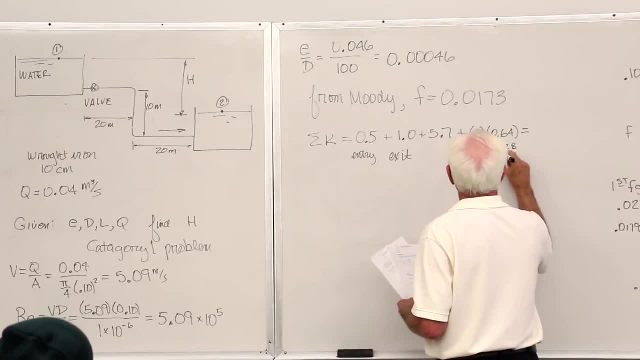 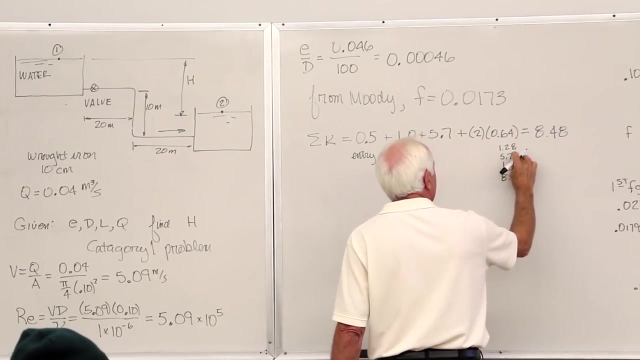 that Okay, Okay, Okay, 1.7 and 1.5.. 8,, 7,, 8,, 9,, 10,, 14,, 5,, 6,, 7, 8.. 8,, 9,, 10,, 14,, 5,, 6,, 7, 8.. Yeah, Okay. 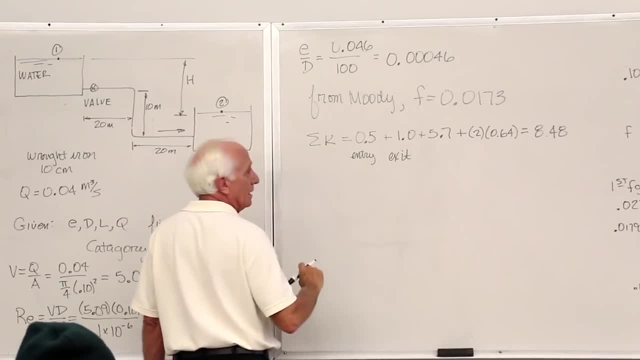 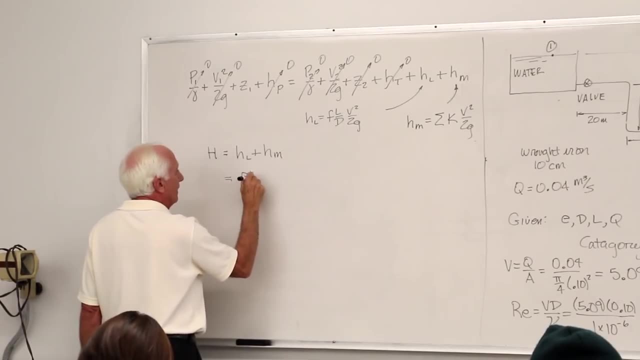 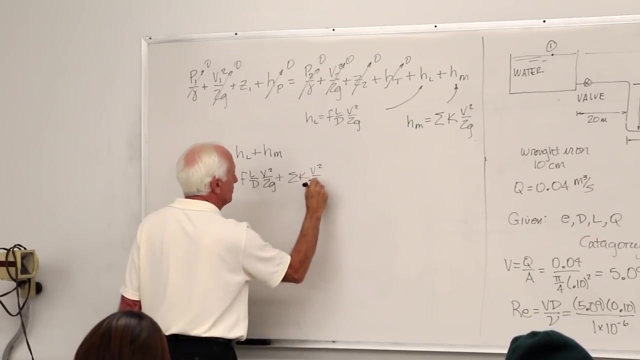 So that those are the summation of the case. All right, Go back over here. Do what it says. H equals F, L over D. Okay, L over D. B squared over 2G plus HM. summation of K's B squared over 2G. And let's see: 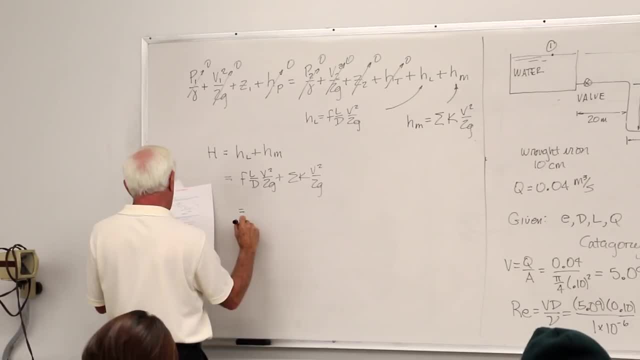 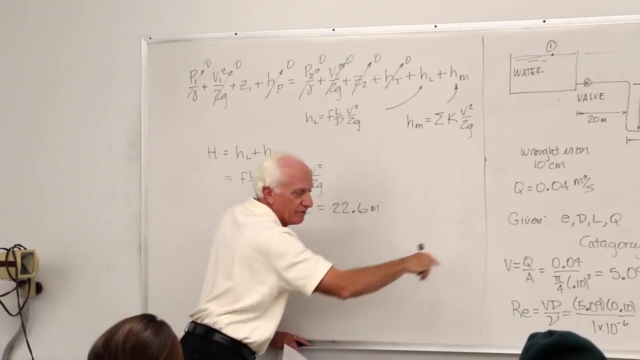 We have 11.4 plus 11.2, which is 22.6 meters. If you plug in the F over there and plug in the K's and multiply by B, it's all here. B squared, 5.19 squared. 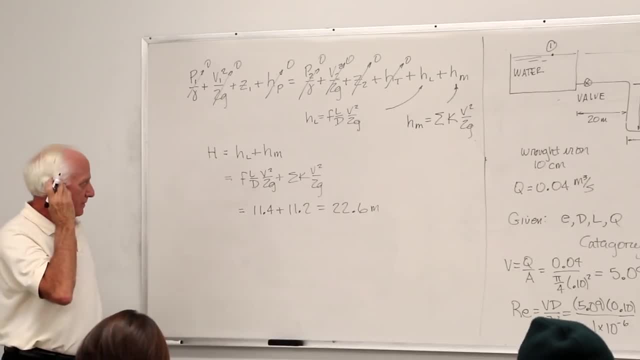 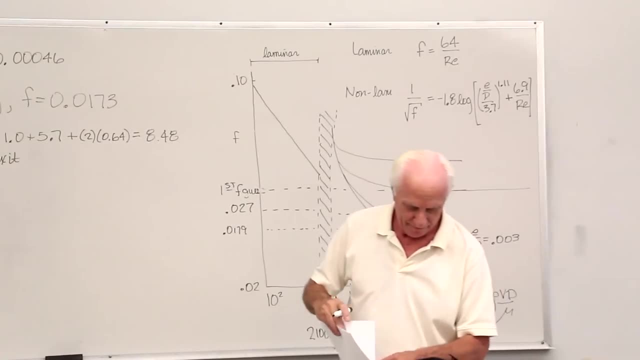 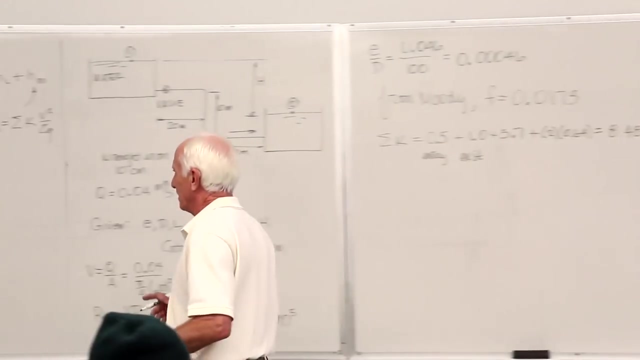 Okay, Okay, I won't go through all the gory details. That's what it is. Yeah, Is the length for the losses? Oh, yeah, Thanks, I won't put that in there. Yeah, Thank you, I meant to mention that. 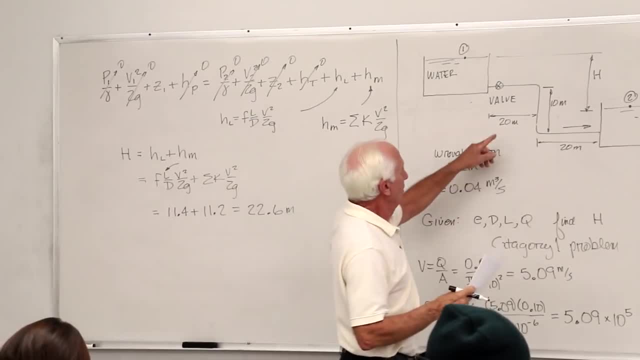 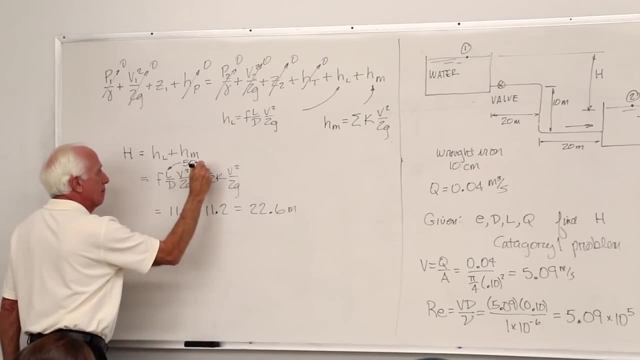 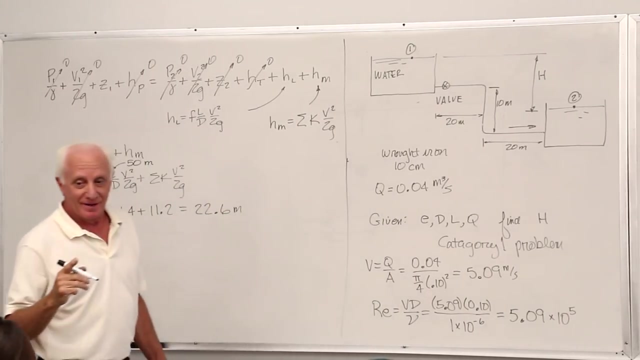 Is everything from point 1 to point 2. a straight line: 20 plus 20 is 40, plus 10 is 50.. Yeah, Thank you. Okay, Okay, Okay, Okay, Okay. Now, as I told you before, they're called minor losses, because normally they're not. 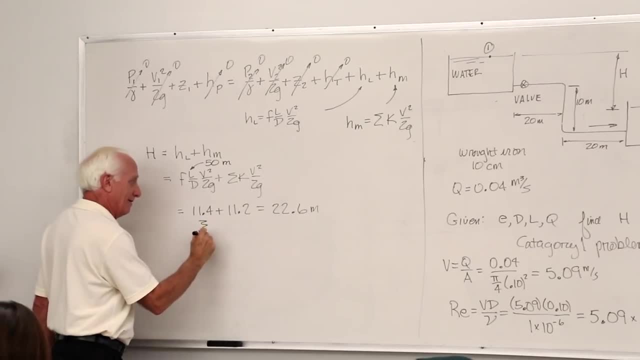 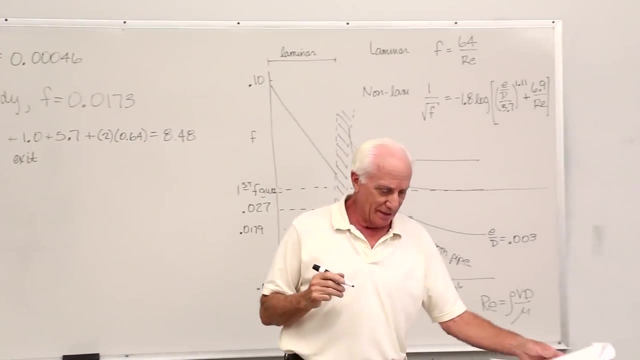 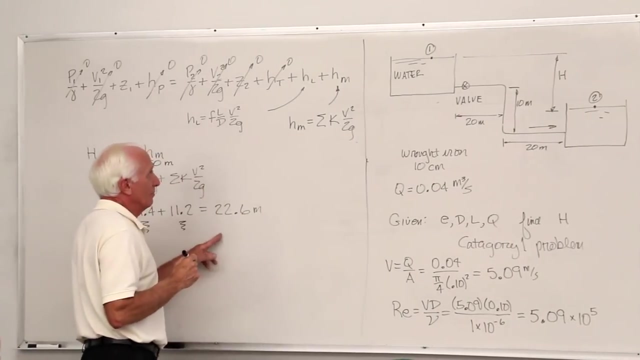 as big as the straight pipe losses. Not here, They're about the same. They sure aren't minor. don't neglect them. Why is that? Because the pipe length is only half a football field: 50 meters, Okay, Yeah. 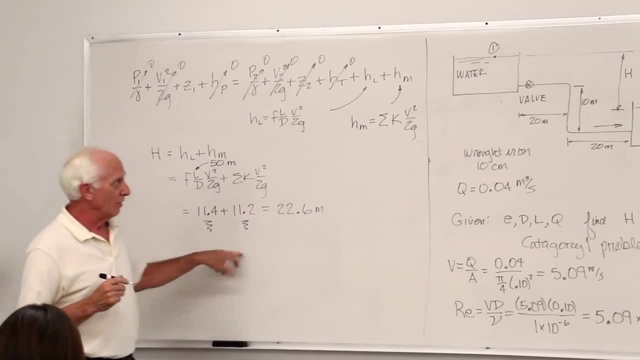 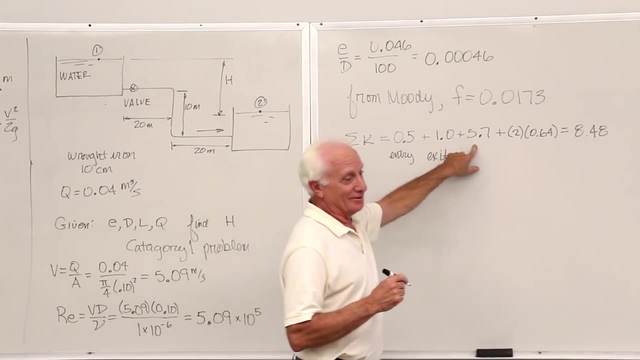 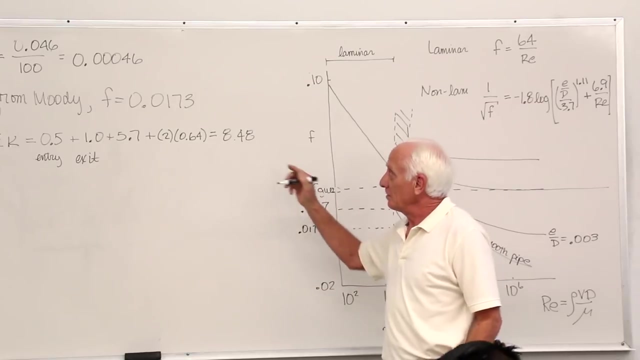 Yeah, Yeah, one too: The loss through that valve. the valve's a big guy. Look at the valve, There he is. What's the problem with that line? That valve is causing a big pressure drop. So, yeah, you can look at the model and say: what should I improve? Well, I don't know. 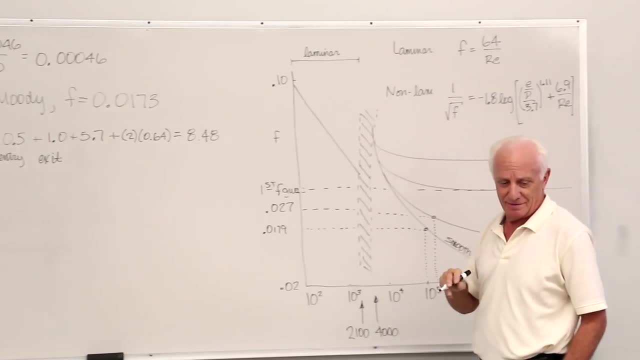 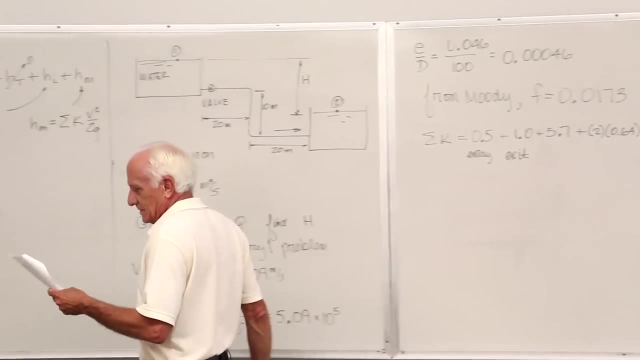 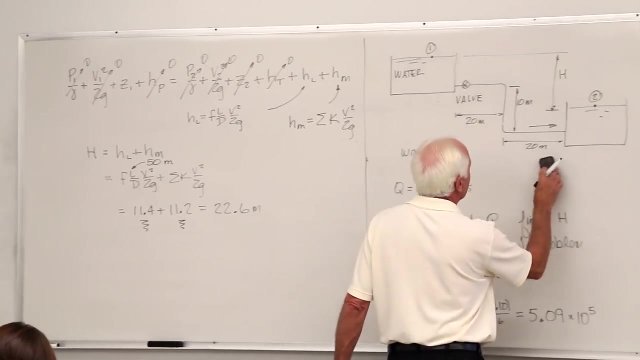 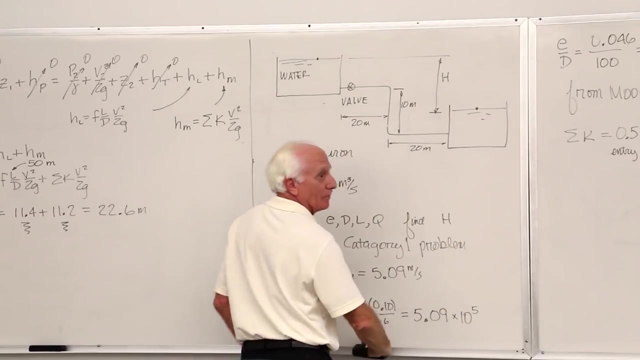 maybe change the valve. That's the biggest loss there, So you can do things like that. Okay, now The last one. we're going to work today, Okay. So now I say you know what I want to pump the water from the lower reservoir. 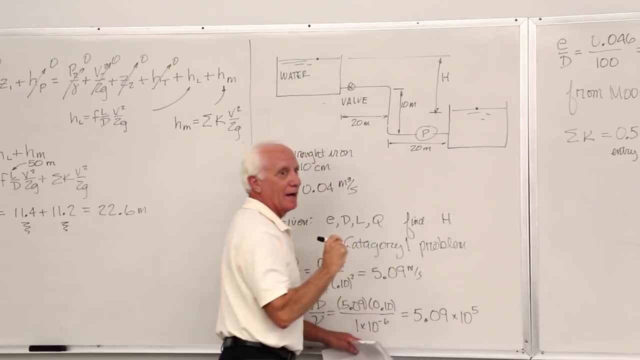 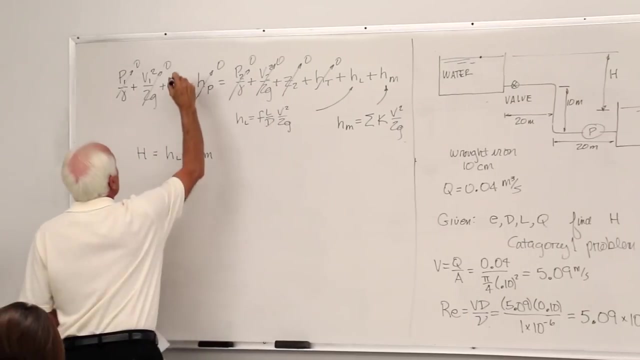 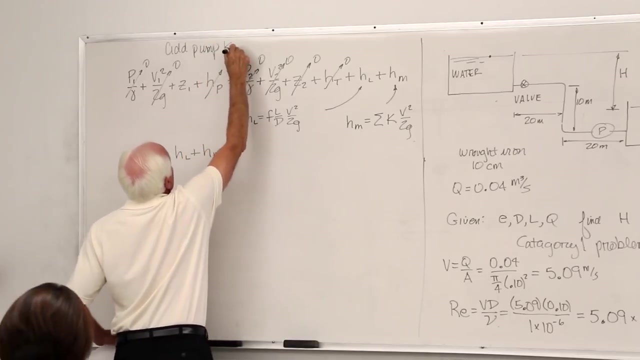 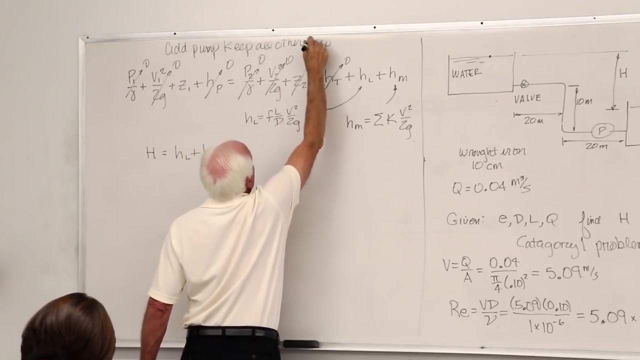 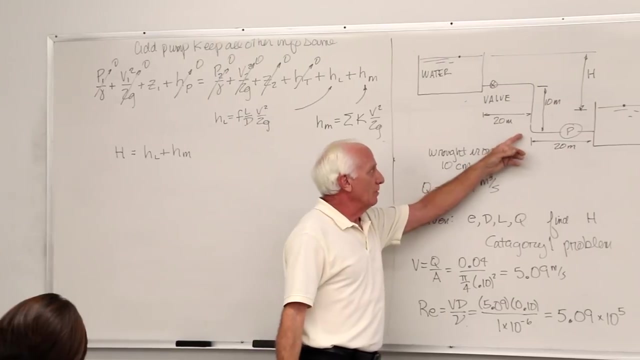 to the upper reservoir. I have pumped And I'm going to use the same conditions. So now, add a pump, Keep all other inflows the same. Is there a valve? Yes, there still is. Are there two elbows? Yes, there still are. Is there still 50 meters of straight? 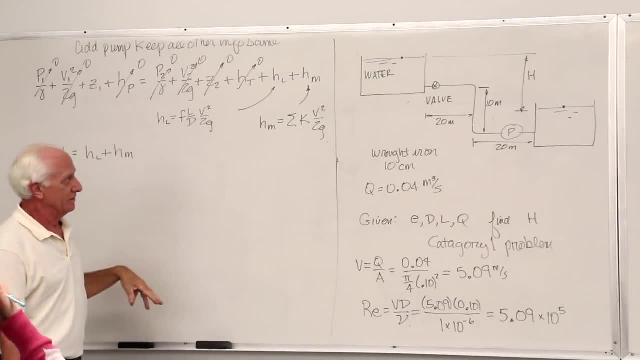 pipe? Yes, there is. Is the pipe wrought iron? Yes, it is. Is it 10 centimeters? Yes, it is. Is the Q.04?? Yes, it is. Everything is the same. I take the answer from the first. 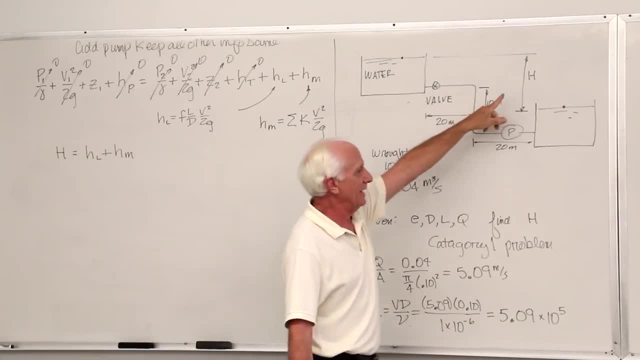 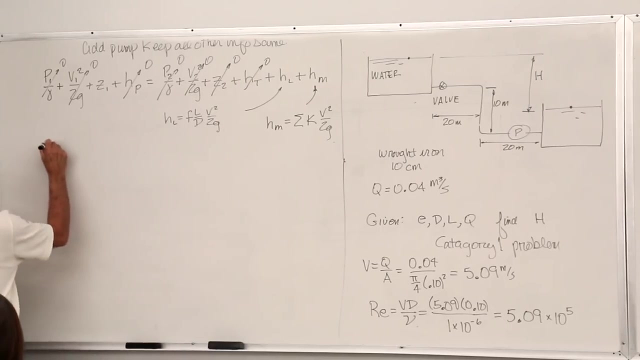 part, which was 22.4 meters. I put that in here for H, And now I want to see how much power has to be provided by that pump to the water to do the job. So find the power needed by the pump. 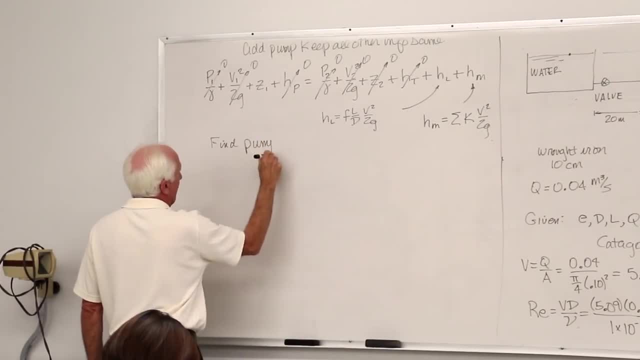 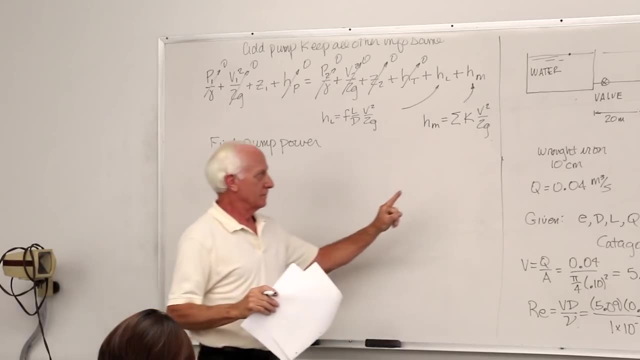 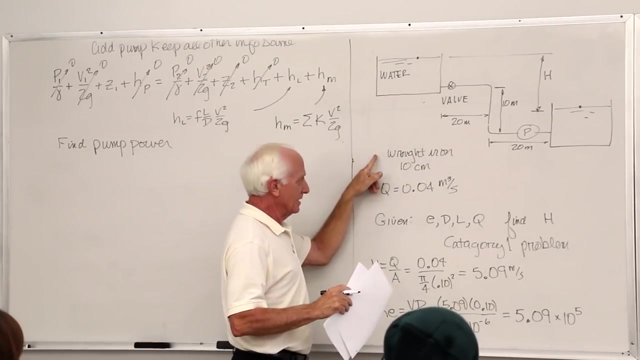 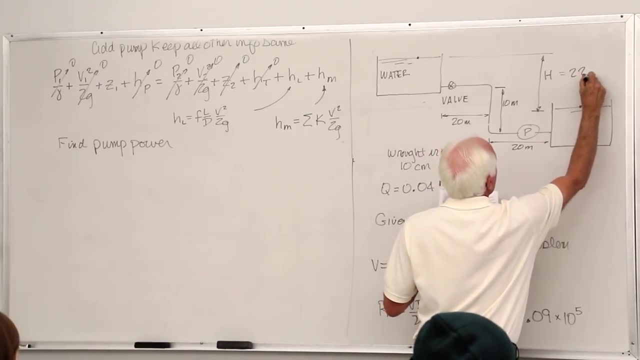 Okay, start again. There's a picture: Yes, yes, yes, valve, yes, water, yes, wrought iron: yes, 10 centimeters. yes, Q, yes. And now H: 22.4 meters, 22.6.. 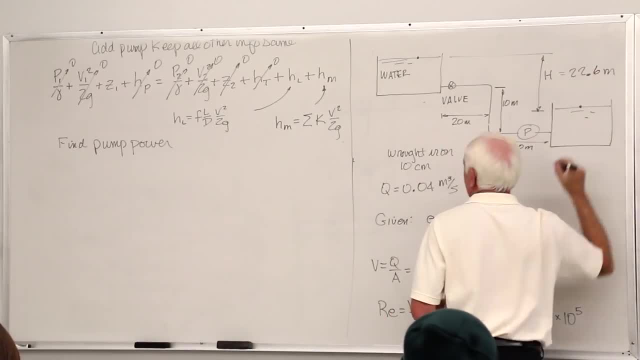 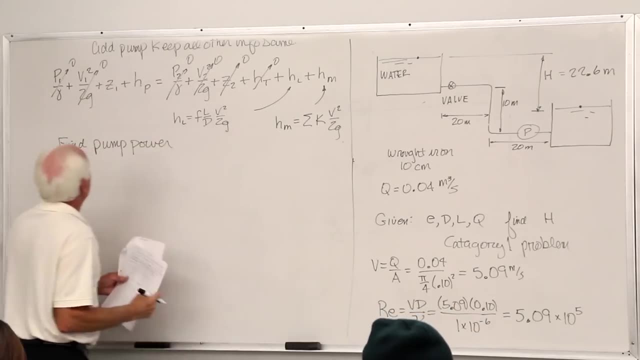 Q.04.. Okay, go back here and say: you know what? I can't do this. now There's a pump in there, Leave that guy in there. Yes, yes, there we go. Okay, let's put point one. You've got. 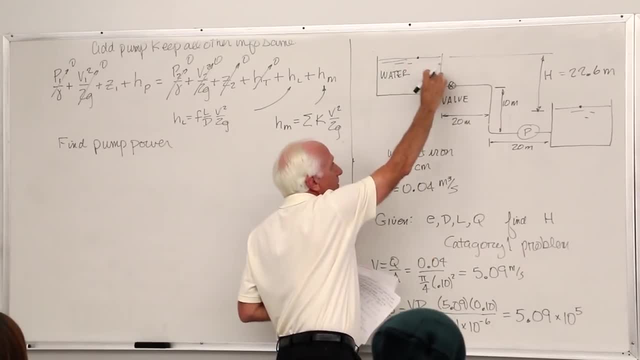 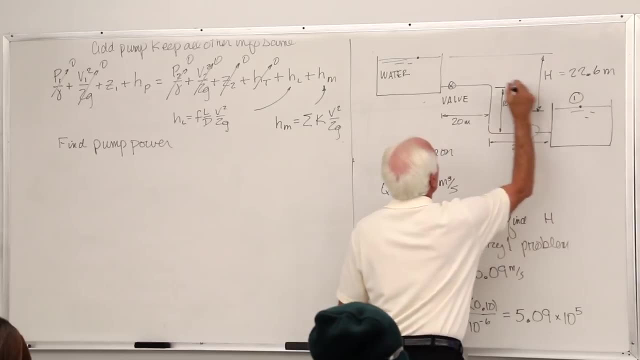 to flip your points. now for the first problem. Point one was up here, Point two down here. Why? Because that's the way the water flowed. Now I put point one here and point two up here. Why? Because that's the way the water flows, from one to two. 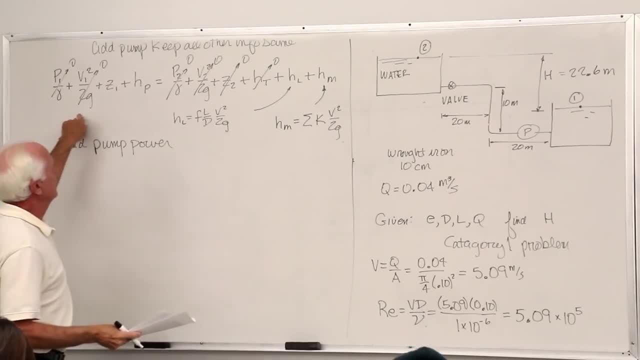 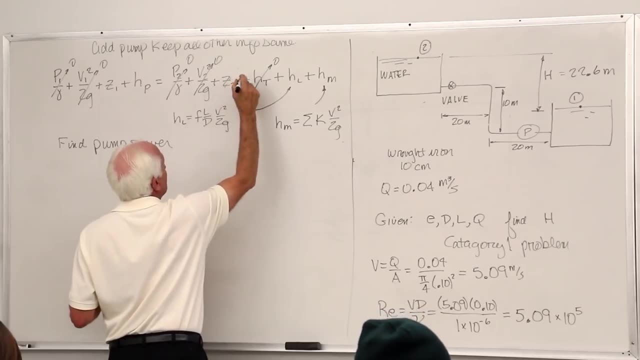 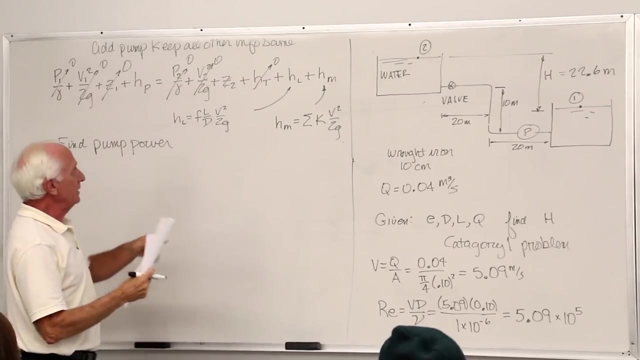 Okay, P10, B10, P20, B20, Z2, H, 22,, 6, Z1, ah, Laura's mark zero, Still minor losses. of course there's pipe are still pipe loss. yes, there is. 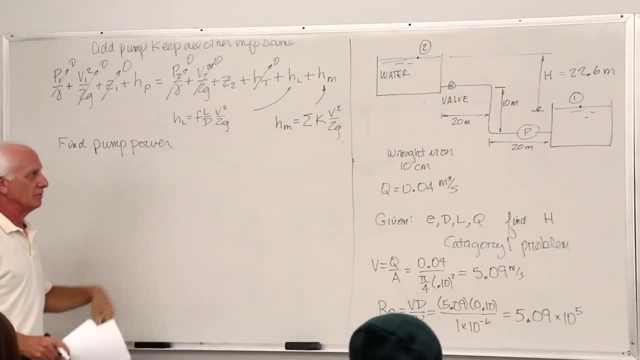 There's still minor loss. yes, there is valve, two fittings, entrance, exit, and so on and so forth. Okay, there it is. HP equals Z2,, 22.6, I'll put H in there- plus FL over D, B squared over 2G. 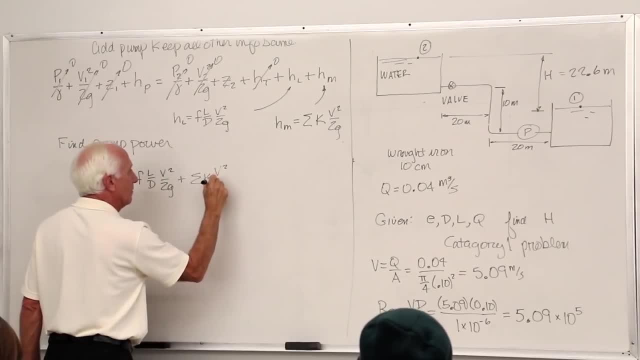 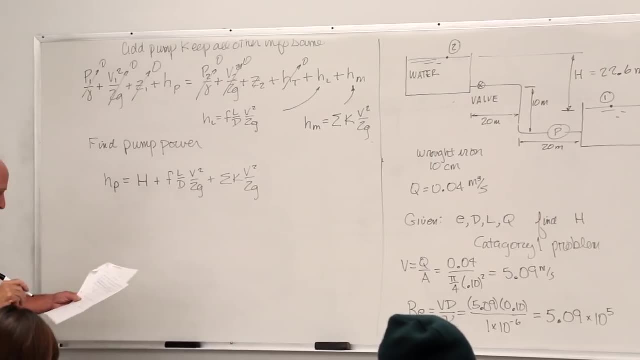 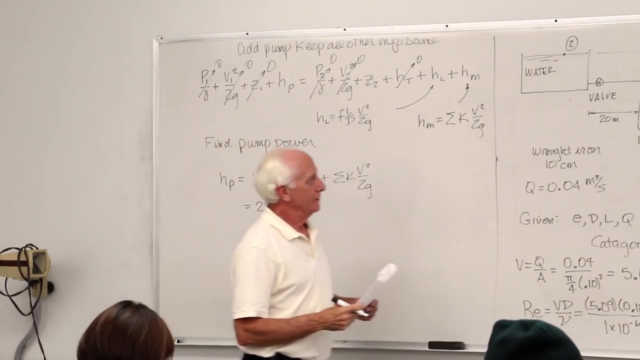 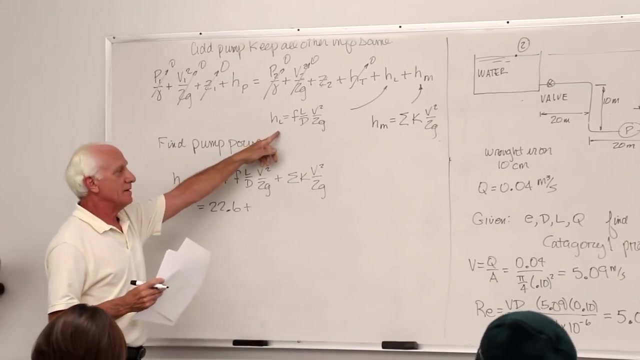 plus summation of K, B squared over 2G. Okay, we're going to put the numbers in 22.6 plus. I erased it, but I've already done that. Did F change? Well, let me ask a question. 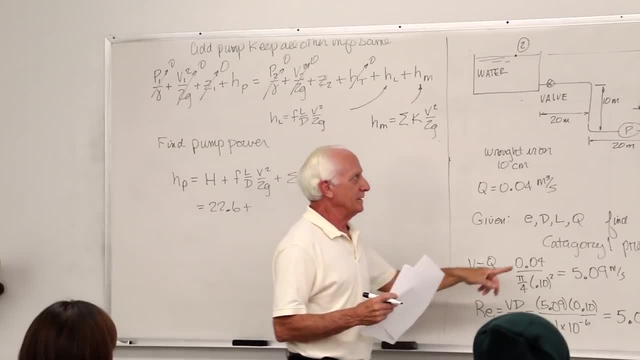 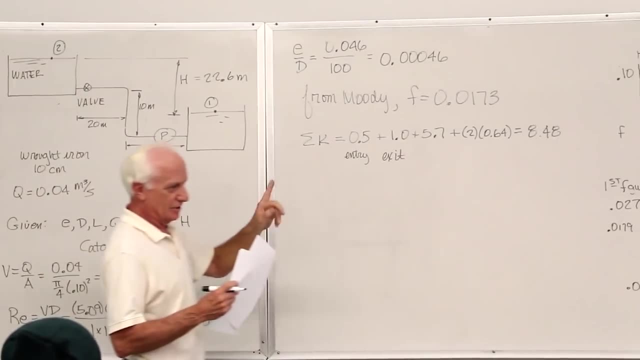 Did the Reynolds number change? No, Did E over D change? No, Is F the same now as the first problem? Yes, Okay, F didn't change. Did I change any of the valves or the elbows, or the entrance or the exit? No, 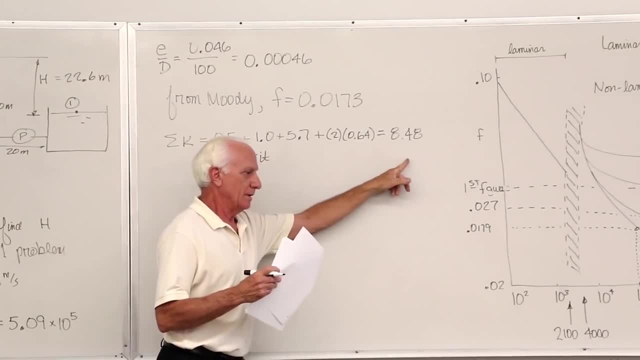 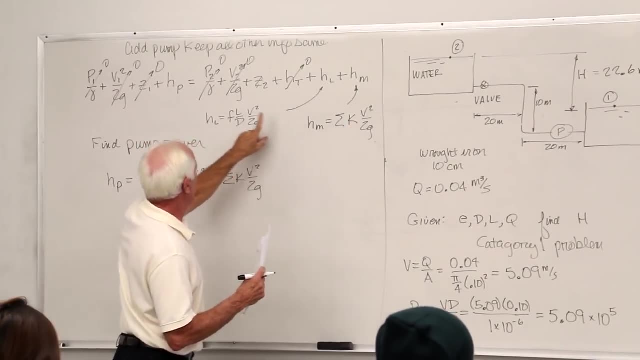 What's the summation of K's? It didn't change. Did the velocity change? Nope, I said 2.04.. B didn't change. K didn't change. B didn't change. L didn't change. D didn't change. F didn't change. 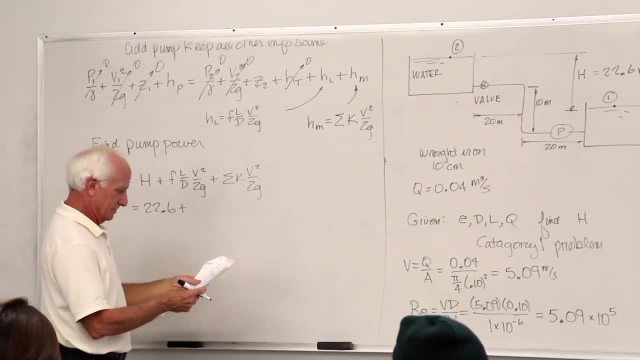 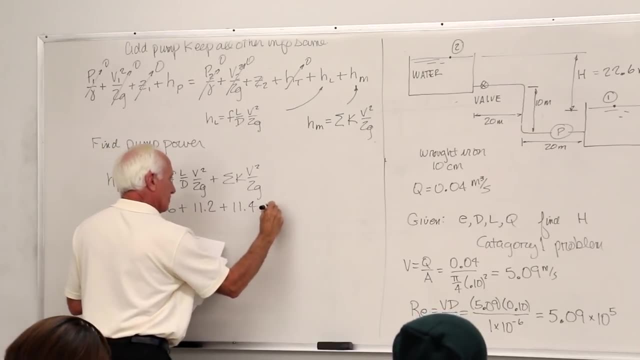 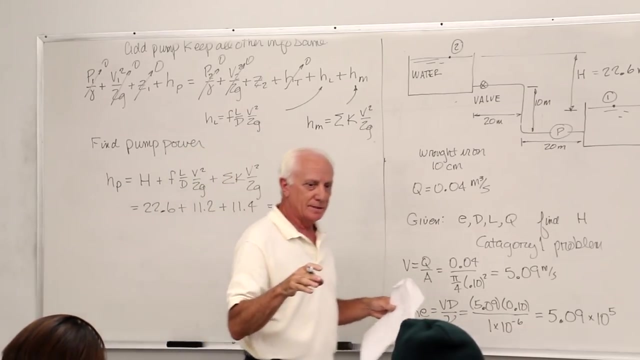 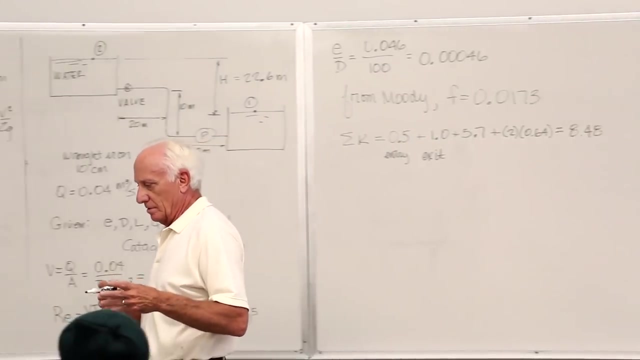 so take the numbers from the previous problem: 11.2 and 11.4.. So now the head. it must be developed by the pump: 45.2.. Let's talk about the energy that the pump provided. The pump is being driven by a motor. 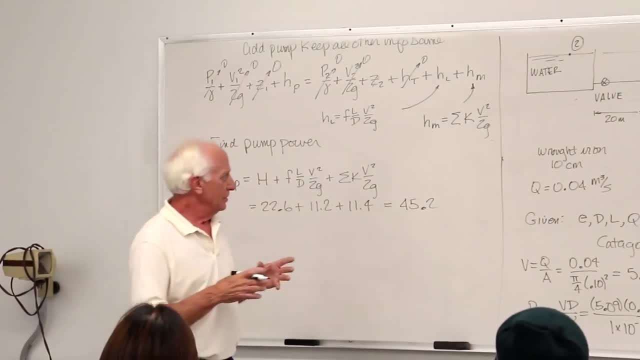 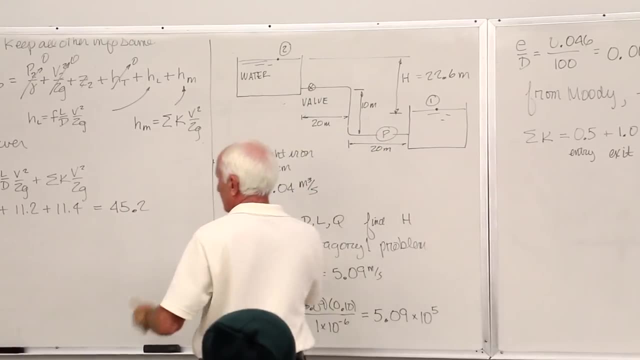 The pump is trying to do something to the fluid. What's it doing to the fluid? Number one is it's raising its potential energy from 0.1 to 0.2.. Okay, there it is. What else does a pump have to do? 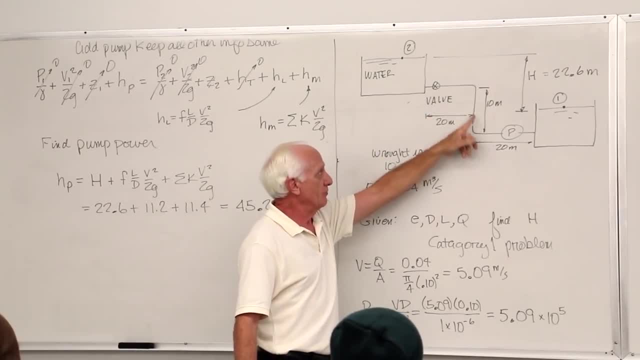 Oh, it has to overcome friction, because there's friction in these rod-arm pipes. There it is. Oh, and, by the way, there's a valve, two elbows and an entrance and an exit. it has to overcome that loss. 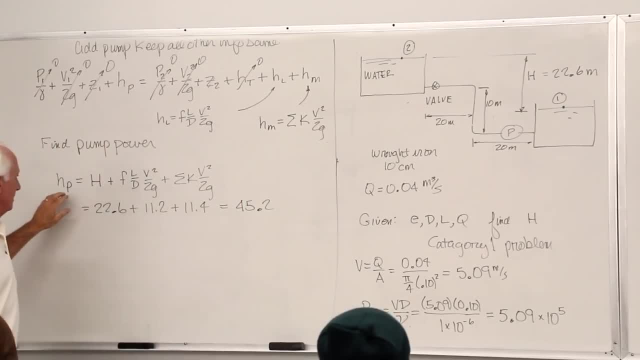 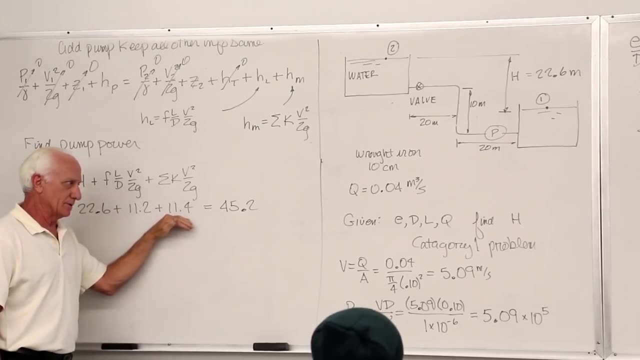 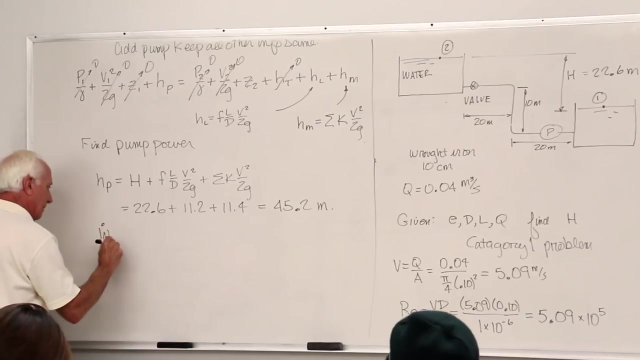 That's a loss of energy. So the pump, the power the pump needs, must raise the water level, it must overcome friction and it must overcome minor losses. that's what it means. Okay, now we know the power. W dot power is equal to gamma QHP. you know gamma, you. 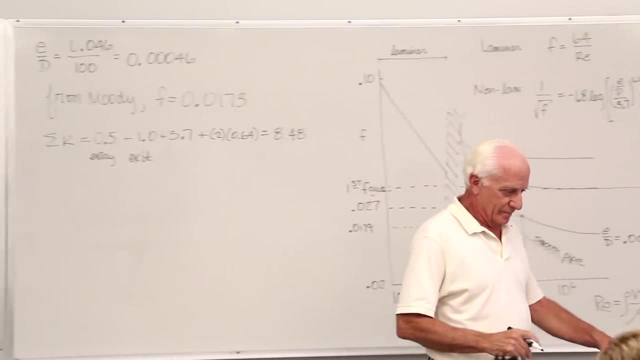 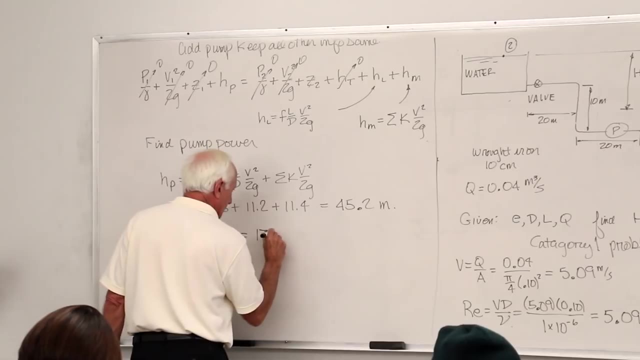 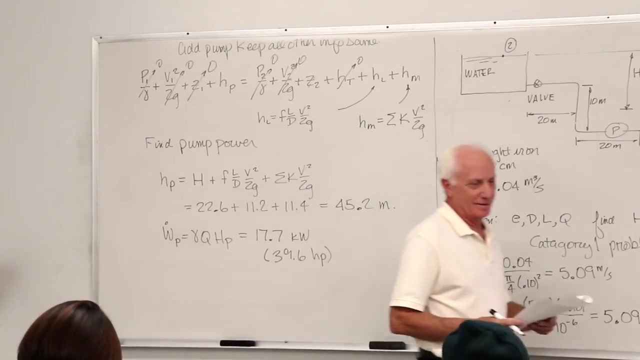 know Q it's given 0.04, and you know HP, 17.7 kilowatts, Which comes out to be convert that 39.6 horsepower. Okay, You probably use a 40 horsepower. I mean 40 horsepower needs to be driven, but the 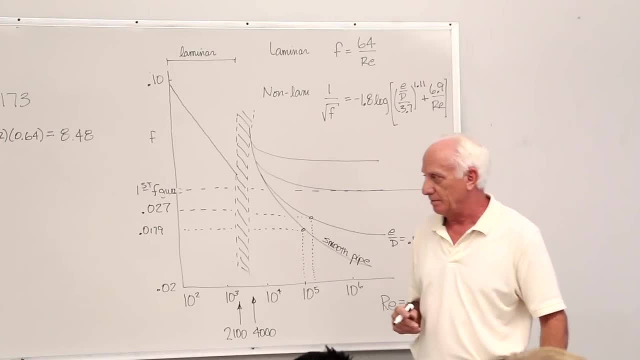 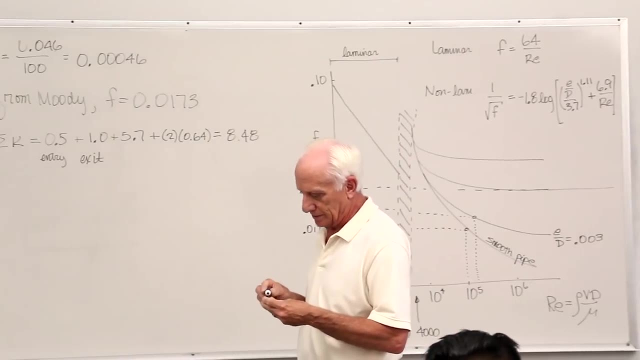 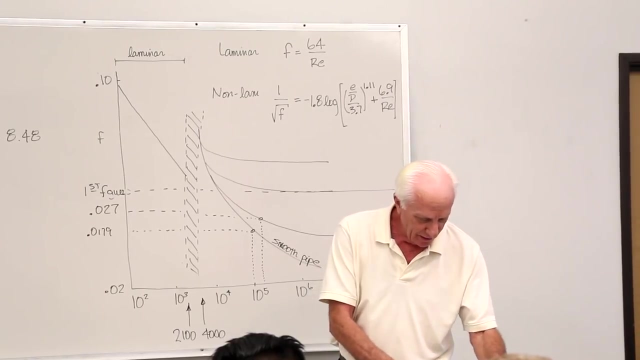 motor, of course, is more than that because of the inefficiency of the pump. So, anyway, the power the pump must provide to the water is 17.7 kilowatts. So we work the problem each way like that, which is a good thing. 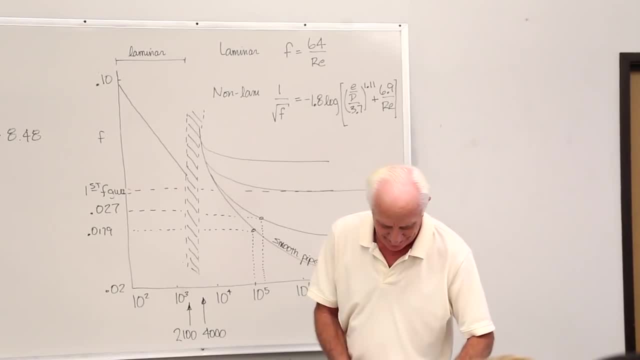 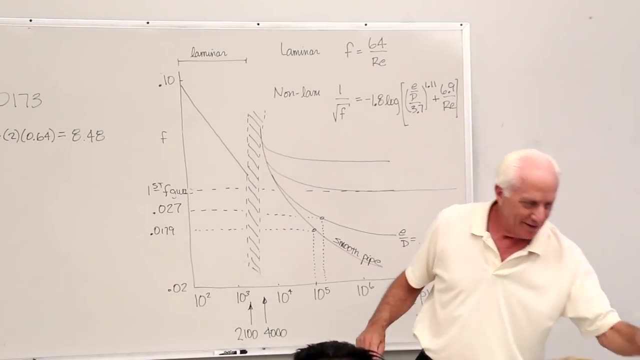 Okay, any questions on that? All right now. Okay, I think we are officially done, except when we're done, I've got all this homework that hasn't been picked up for the quarter, so if you're missing any homework or exams, it's. 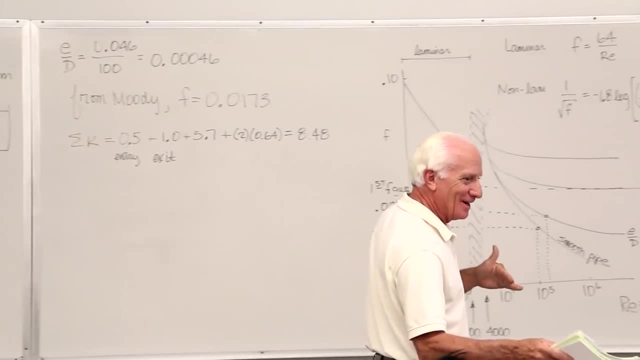 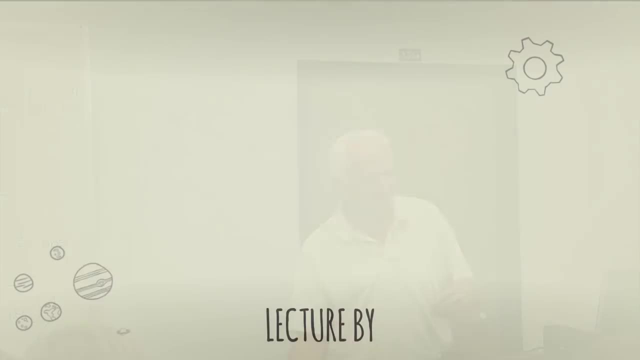 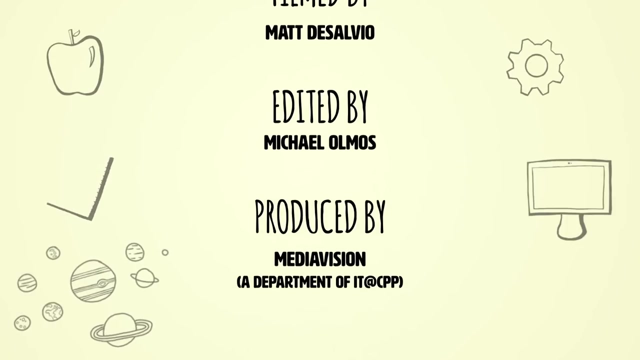 in the stat. So it's up here in front and otherwise we'll see you Monday afternoon. get a good night's sleep and a good lunch- Not too much sleep- And we'll see you then. Bye, Bye.